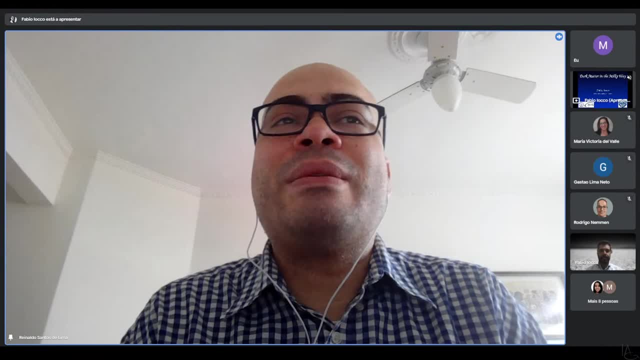 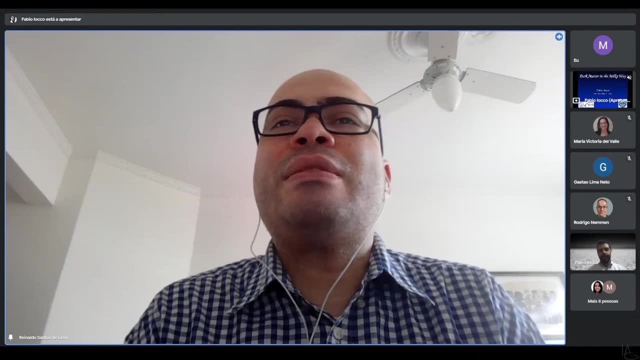 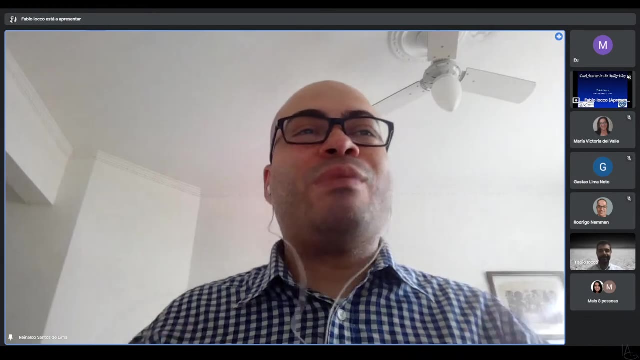 including the Kavli Institute in the US, Instituto d'Astrophysique de Paris, Oscar Klein Center for Cosmoparticle Physics at Stockholm and Instituto de Física Teórica in Madrid. Fabio, please correct me if I make any imprecision. 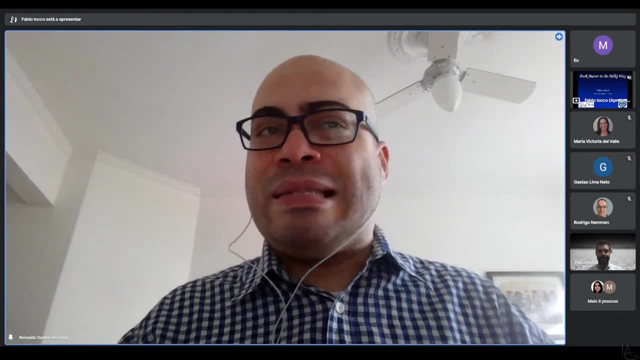 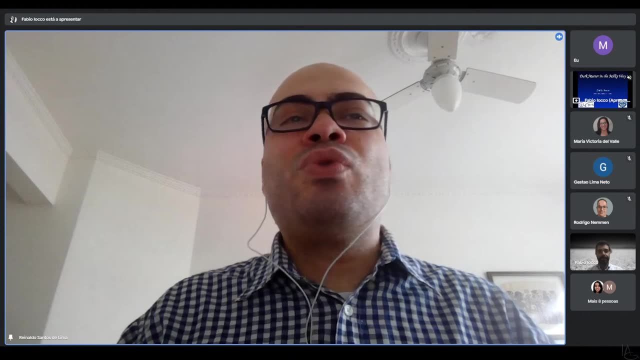 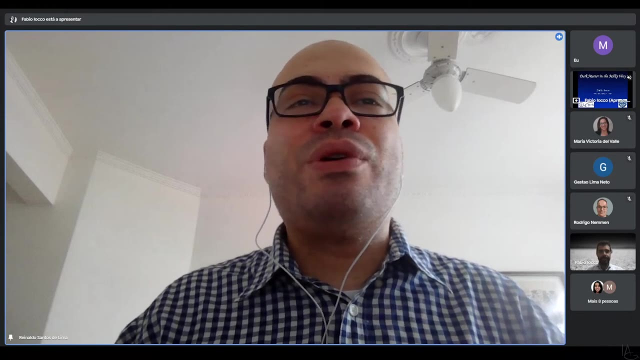 And from 2014 to 2019, he worked as a professor at the ICTP, at the Instituto de Física Teórica UNESP in São Paulo, and since then he is a faculty member. Currently, he is a faculty member at the University of Naples in Italy. 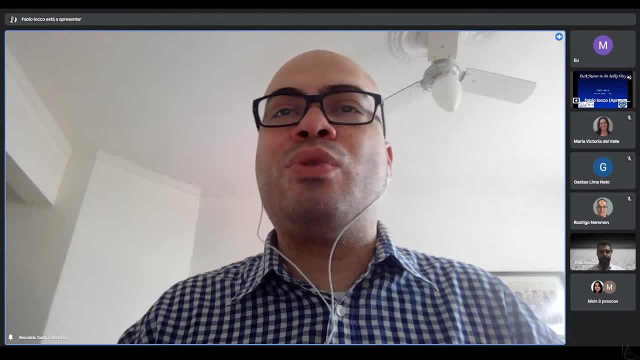 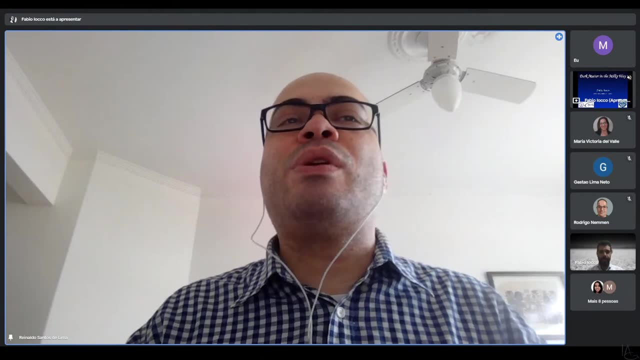 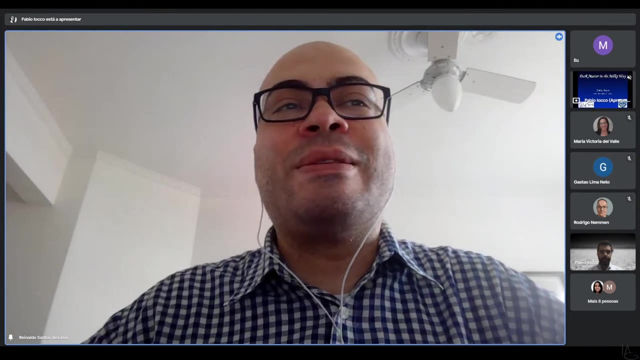 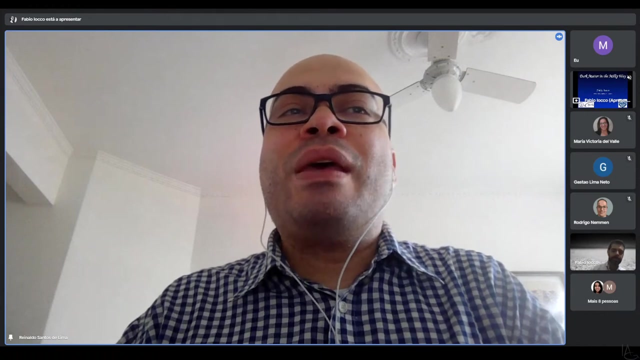 and he works in collaboration with the Astroparticle Theoretical Group, And some of his main research interests are related to Big Bang and Nucleosynthesis, the first stars, dark matter phenomenology and high energy astrophysics. And today Fabio is going to present the seminar Dark Matter in the Milky Way. 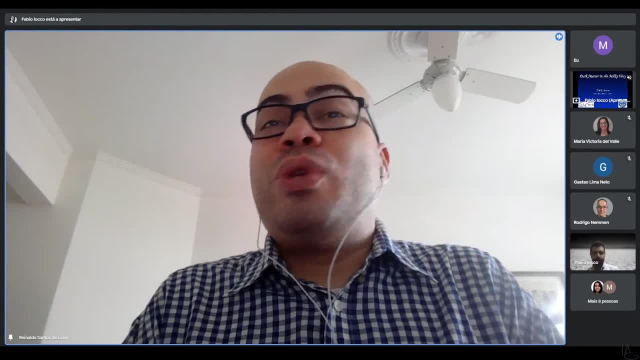 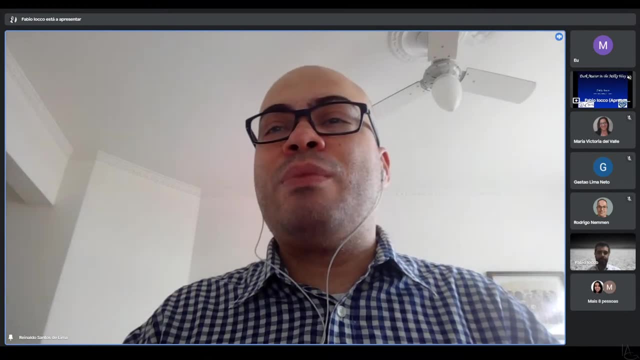 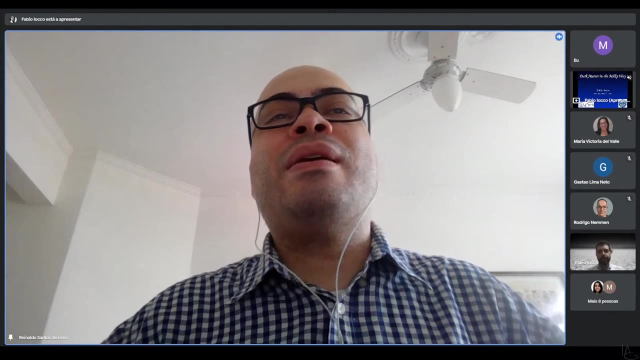 Questions can be addressed to Fabio during his presentation or after his presentation is open. if you want to just interrupt him, so you can push the button to raise your hands, And if you are following the seminar broadcast on YouTube, you can ask your questions in the chat. 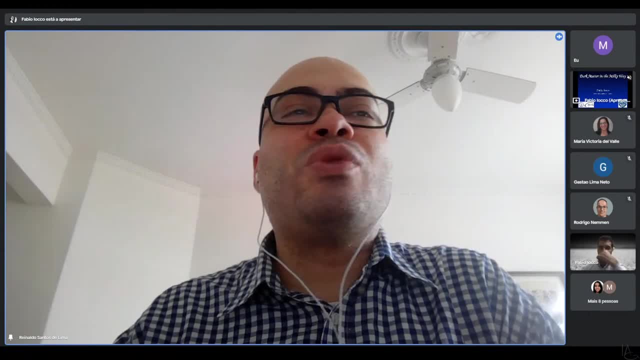 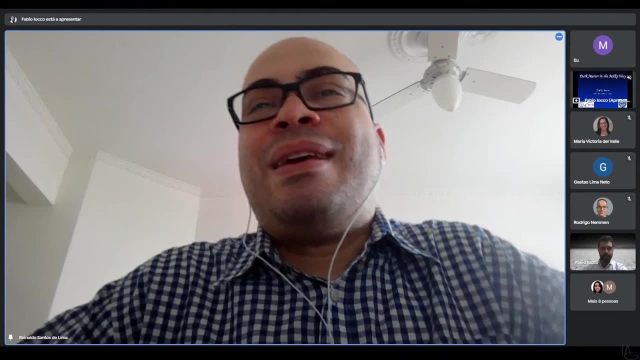 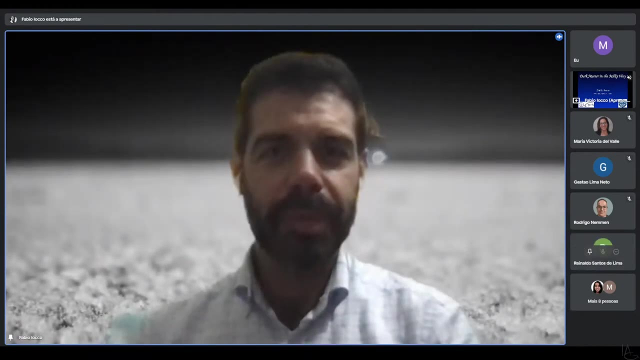 And before the seminar begins, I would like to ask those present to please turn off your microphones and cameras And please, Fabio, feel free to start. Thank you very much, Reinaldo. Can everybody hear me? I guess you could hear me before, so you can hear me now. 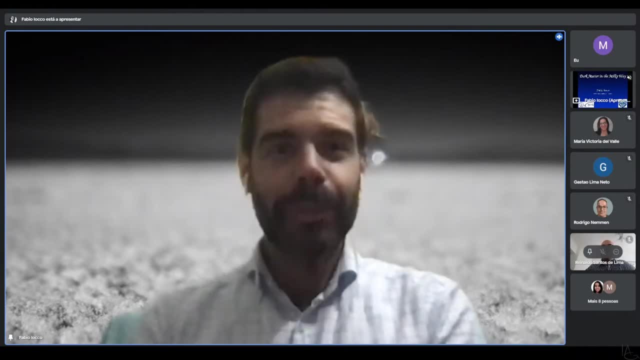 Yes, Unless you say differently. Great, And thank you very much for the invitation. It's really a pleasure to be back to IAG, even if only online, but it's really a pleasure to see the community And to feel part of it again. 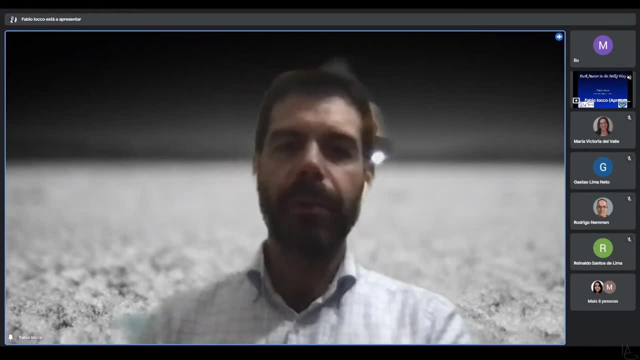 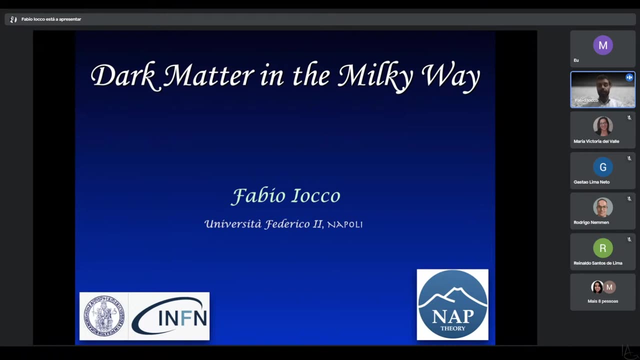 So I will present some work that I've done over the last approximately 10 years in different formations, And so part of the work that I'm going to present has also been done while I was in Sao Paulo, across the Red Line, with respect, across the bus line actually that connects IAG to Barra Fonda. 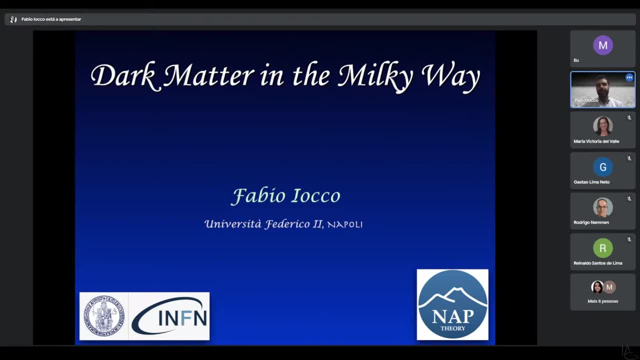 But it's still fresh, I would say, And part of the work was done while I was sitting at the IAG. I was there as a guest quite often, So it is fitting. So I realize that the title of this talk, put this way, is a bit generic. 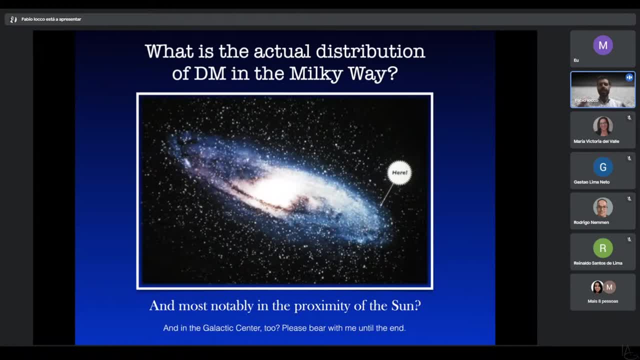 Quite very much so. So the questions that I was trying to address, that I will try to address, is: what is the actual distribution of dark matter in the Milky Way, most notably in the proximity of the Sun, Even more interestingly to me, at least at the Galactic Center? 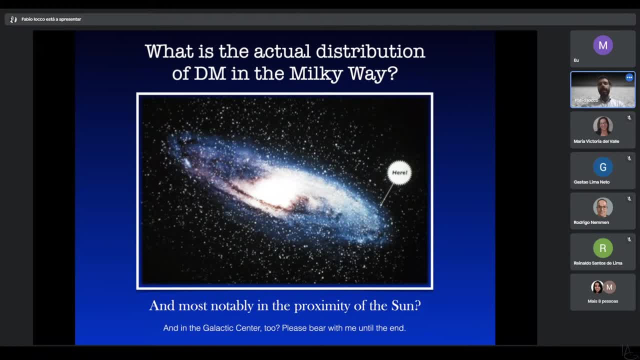 though this has very different dimensions, although this has very bitter surprises in the end- and also how the distribution of dark matter, how we can access the information about the distribution of dark matter, carrying uncertainties, somehow reflects on the knowledge that we have about the nature of dark matter. 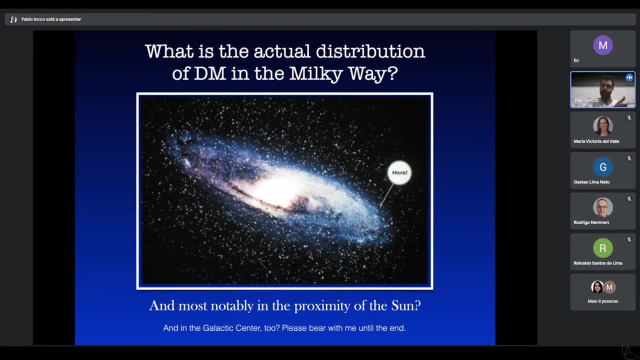 So how we can propagate from the astrophysical uncertainties that I think are more of interest of the community that is listening, now down to particle physics, which is a little bit the two things that I've been doing and I've been doing consistently. 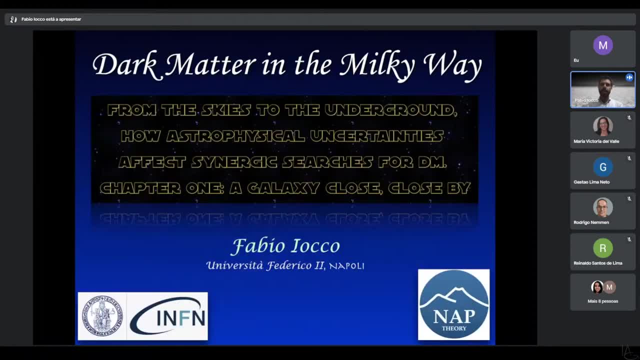 So, if you want, the title of my talk can be put in this way, which is a little bit more clear about the content of the talk. And while I was putting in this sort of jokey form, I realized that a galaxy, you know, this is the Star Wars thing. 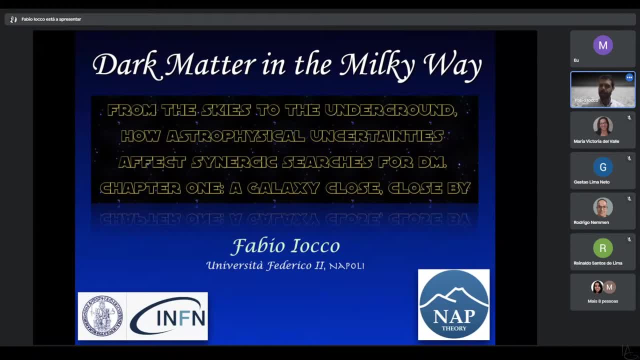 and there's a galaxy far, far away. And then I was thinking about the Milky Way and a galaxy close, close by, And then it occurred to me that, indeed, the galaxy far, far away, which Star Wars talk it's been taken, and the stories that emerged from Star Wars, 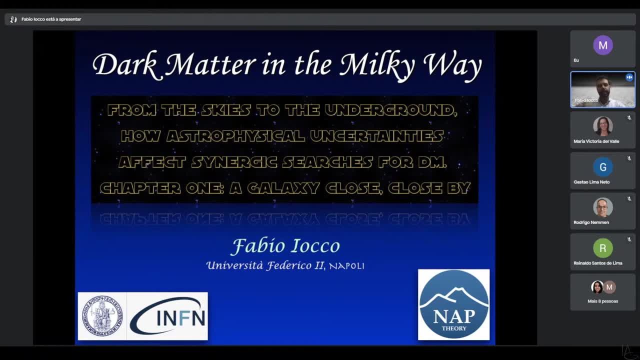 have been heavily inspired, at least as a shape, as a form, and especially in the figure of Han Solo and all the pirates that appear in Star Wars, has been thoroughly shaped by the foundation of Isaac Asimov, And so recently my father passed away. 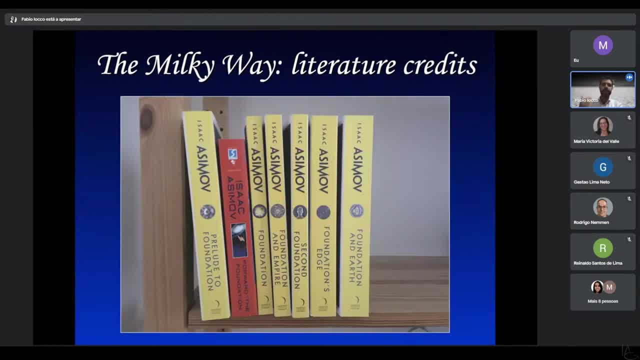 and I dedicated myself to reading books that he had given me when I was a child, when I was 13 years old, which is a highlight shift now, And this summer, I dedicated myself to start to reread the older foundation series. 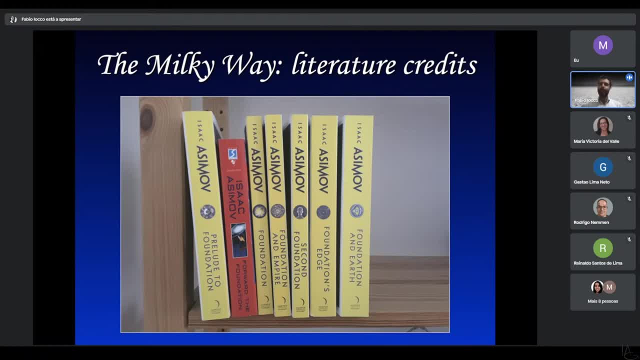 and I found amazing inspiration about the galaxy and how the galaxy is not only an object of scientific study, but the passion for the galaxy for me is apparently well-radicated from the time I used to dream about and look about it, And so these few slides are meant also to break the ice. 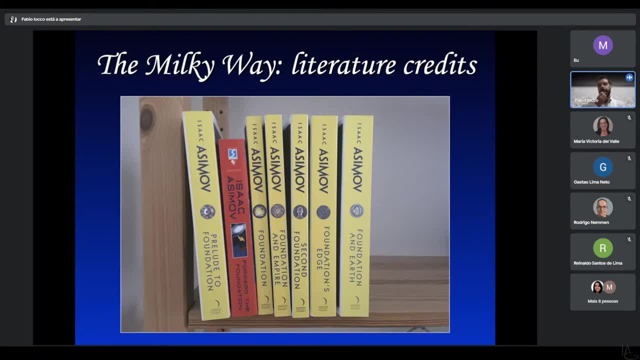 and to allow some people to come in. And I also realized how the part of the Milky Way, the fascination for the Milky Way and the fact that we call the Milky Way the Milky Way, is something extremely centric to the culture, to all the cultures. 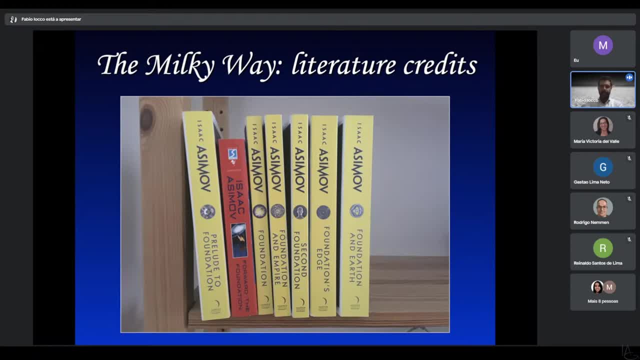 But the fact that we call it the Milky Way is due to one myth in particular, And I don't know how many of you are familiar with the Greek myth and why we call it the Milky Way, Which is in fact, again related to the name of galaxies. So the Milky Way is called like that because of milk, And I'll come to the legend that has the milk in it, But milk in ancient Greek, and it's a Greek legend, but milk in Greek is said galaktos. So the galaxies, and the galaxies are, by extension, related to the Milky Way. 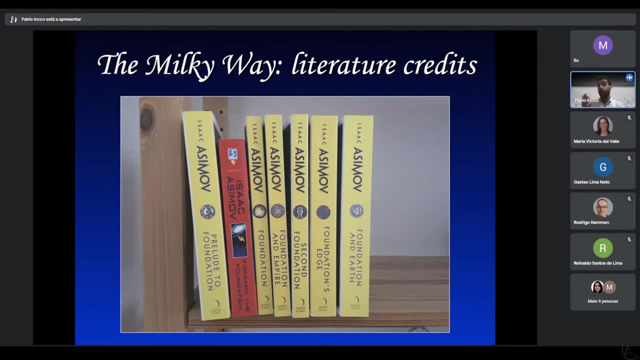 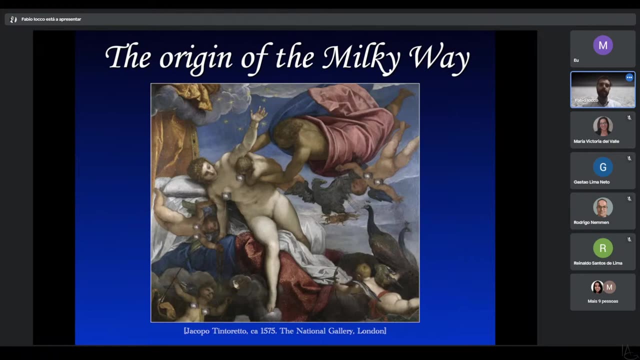 even in the name, And so the legend- which is obviously not the only legend- about the origin of this stripe in the sky that we see from the northern and the southern hemisphere in the Greek mythology is due to the fact that Zeus Jupiter actually was very fond of a mortal. 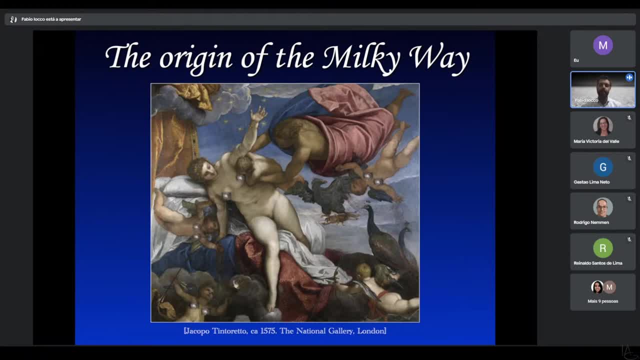 We could not call it love. I don't know if we would call it love today, but he was very fond of a mortal And she gave birth to a son out of dispassion, dispassion with Jupiter, And Jupiter was extremely scared that the mortal 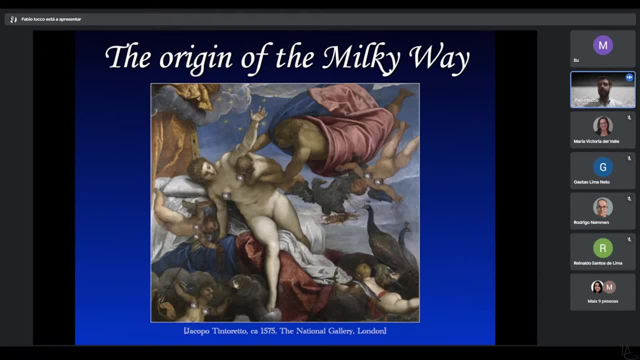 that this baby could have only mortal skills and mortal weaknesses. So he had this brilliant idea to take the son out of an adulterous relationship and have it breastfed from his wife, who was a goddess, And so the baby would absorb the milk of the goddess and the power. 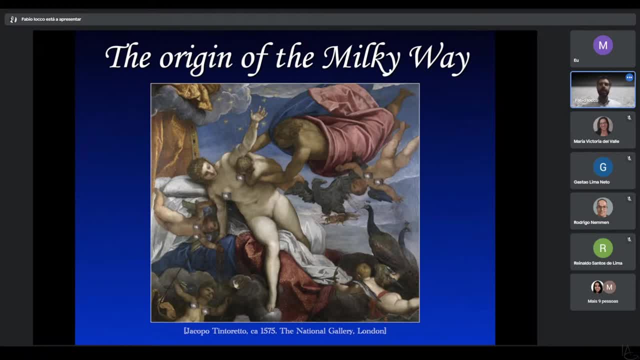 So this baby that later became very famous- I'll tell you the name in a little bit- This baby was. he got there. Amazingly, the wife of Jupiter, Hera, did not reject the baby, although it was the son of his husband and someone else. 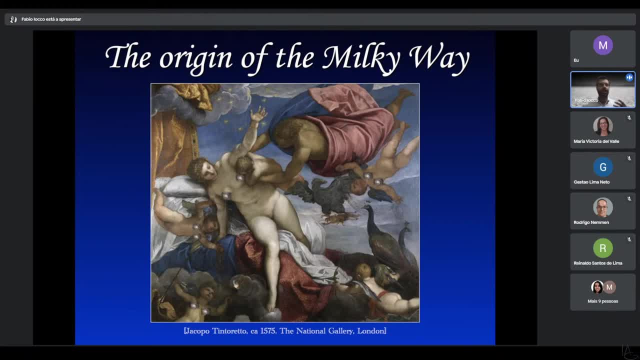 And she started breastfeeding the baby And the baby started crying, etc. And some milk spread into the sky. Of course, everything was happening into the sky, because these are gods, And therefore this stain that was left in the northern sky that the Greeks could see. 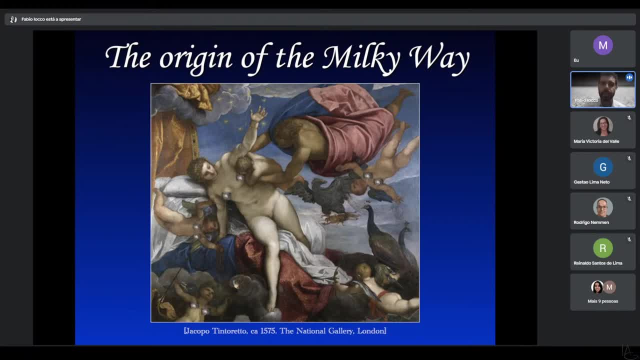 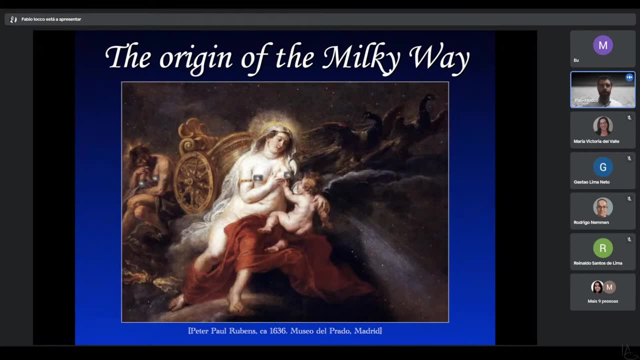 it's called the Milky Way. Now, there's several interpretations of this legend. I prefer this one by Rubens. You might also notice that, not knowing the policies of YouTube and all the institutes around the world, I covered all nipples, male and female. 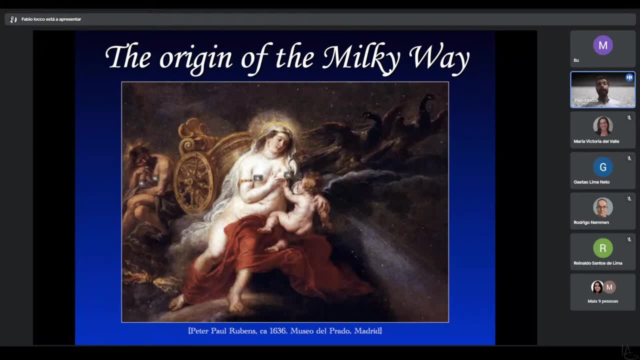 so that there is absolutely no obscenity, But I found that it's very powerful. There's a lot of legends, but as usual- and I don't think this is right, but somehow mesmerizingly, the Western culture has imposed itself in its own view, even in the general name. 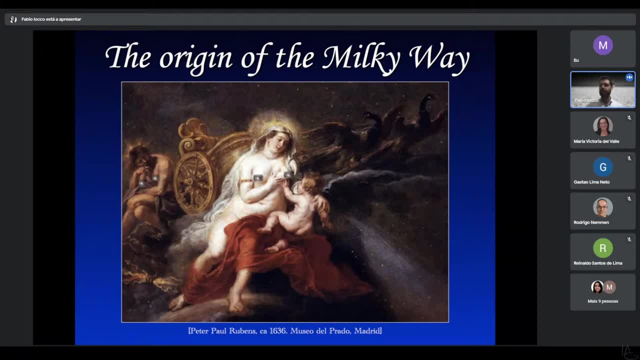 Now all the legends that I found, especially relating to the southern hemisphere, very interestingly, many legends from the southern hemisphere. see the black parts of the Milky Way, see the gas clouds that are in absorption, rather than the haze, In fact, if you look at it from the southern hemisphere, 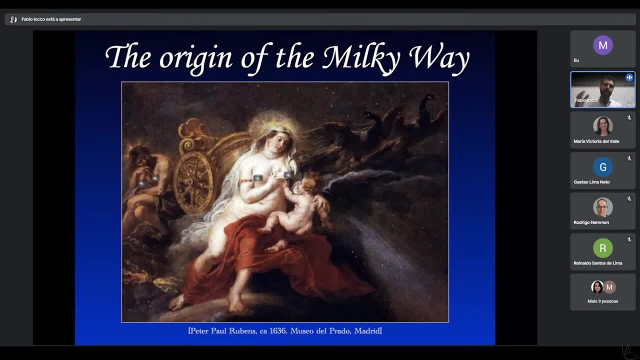 that makes more sense. And, just as a last thing, you know that all this thing of breastfeeding the baby and giving him godly powers, of course it worked, because the name of the baby is Hercules and of course it became mortal, but very, very powerful. 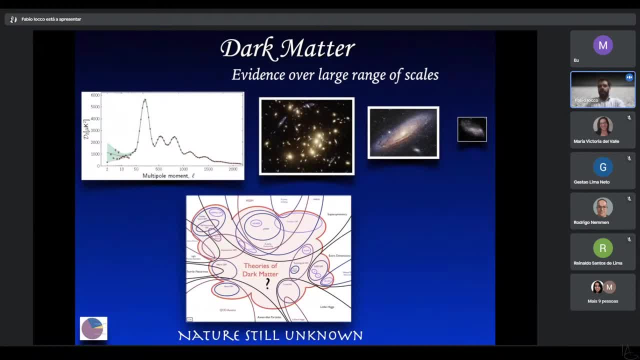 So let's get back to Milky Way and why I think it's interesting, not only per se, and again, all this introduction was to show you that I find it interesting as an astrophysical object and as an object of observation for human activities. 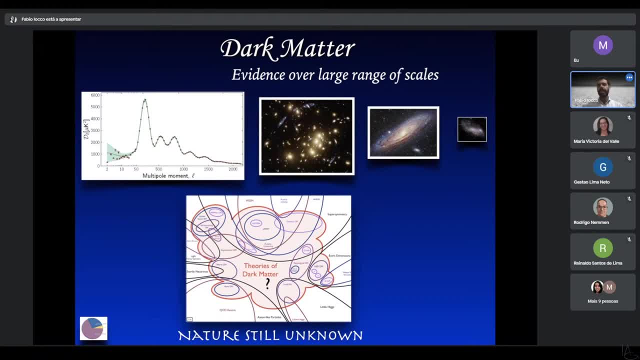 But it is interesting for what I've been doing in the context of dark matter, because the problem of dark matter, if you wonder, the existence of dark matter, arises on many astrophysical scales. it arises on very small scales, pressure-supported galaxies. 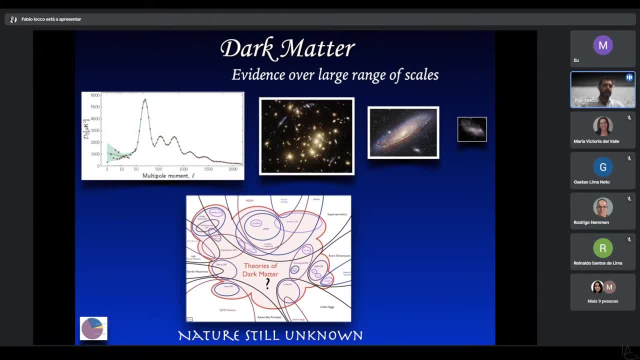 it arises on disk galaxies, bigger systems. it arises in clusters of galaxies and is most notably found in the CMB, in the Cosmic Microwave Background. Now, the thing that I found extremely satisfying is that all of these proofs independently with different physics. 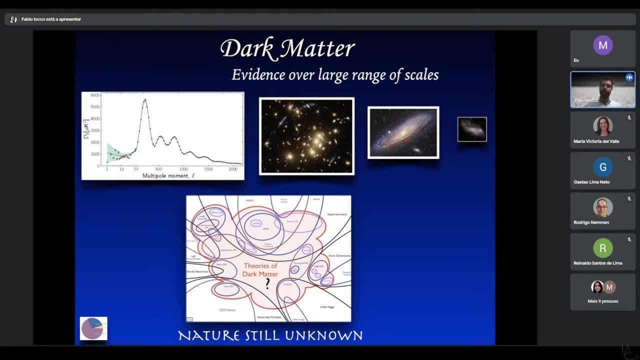 and with different techniques, point to the existence of a component which is gravitationally coupled and non-electromagnetically coupled. yet we do not know what this dark matter is. Okay, So, from an astrophysical point of view, we'll just take a fluid. 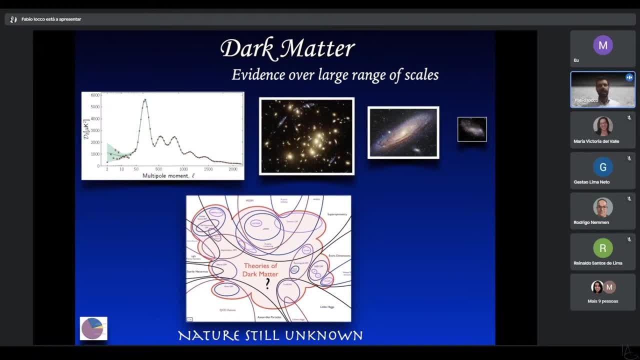 we don't know what it is. it has to have some properties like. it must be produced as cold. so the relative velocity, the velocity-to-mass ratio of the particles at decoupling and matter radiation equality must be small. There's a lot of things that comply to that. 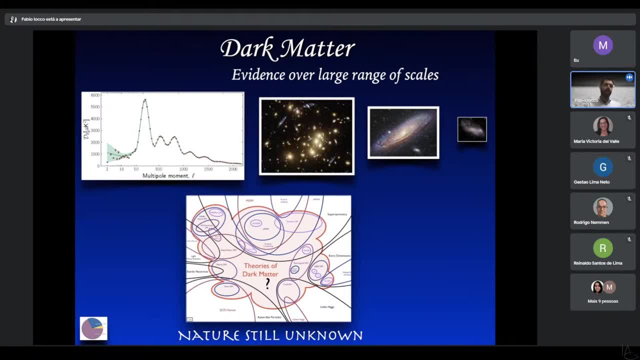 We tend to think of dark matter as something non-baryonic, so an extension of the standard model which is widely depicted here. but we might also think of it as some special type of baryons that have been locked down in primordial black holes. 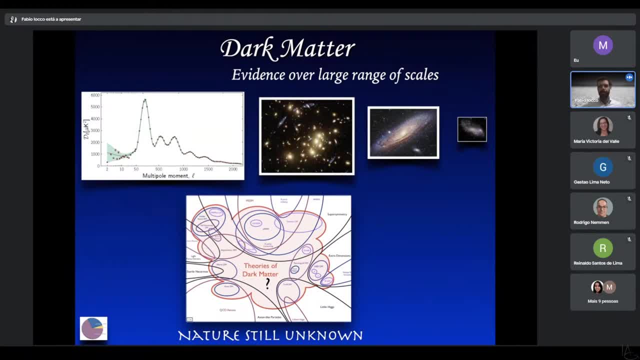 For the moment, this doesn't affect what I'm going to say at all. As long as there is a five-to-one ratio of dark matter to gas, we can follow the evolution in the Universe and we can cosmologically reproduce the galaxies that we see. 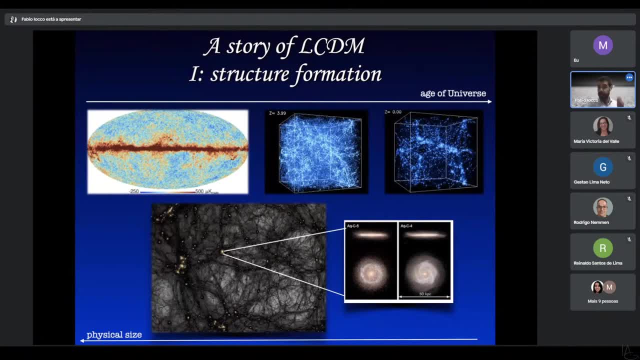 If we start from the perturbations that we observe in the CMB. so this is an observation: we seed perturbation with the same spectrum, we evolve them, and there's people who do it also in IAG: we evolve them. 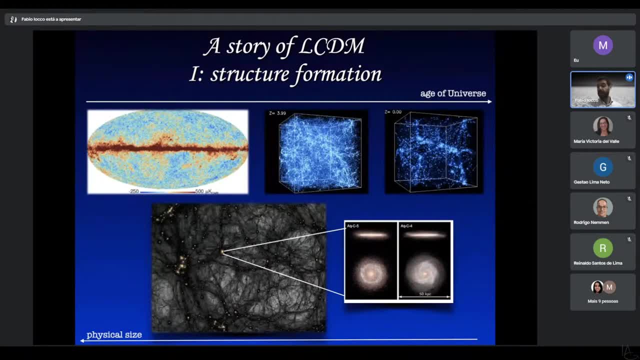 we can form the perturbations of density in the way we see them today, and so we have a spectrum of a power spectrum today and a different redshift that resembles the one we observe, and, even more interestingly, recently at least. 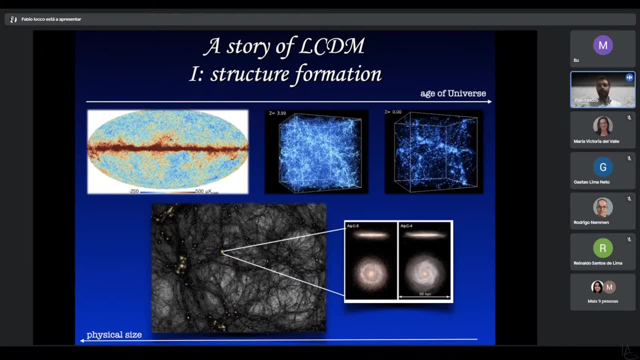 that was not the case when I was a student. we started forming galaxies, so we started having numerical solutions of equations that do not only include fluids which have simple properties like just gravitationally coupled, but people have started simulating an additional fluid which has subgrade physics. 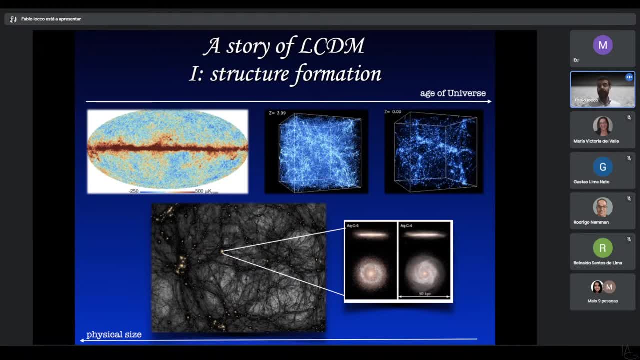 that mimics the property of the gas, and they can form galaxies. The most remarkable thing is that they form galaxies on the different scales and they have galaxies that match the observation in the simulation. So if you want the theoretical solution of a cosmologically expanding Universe, 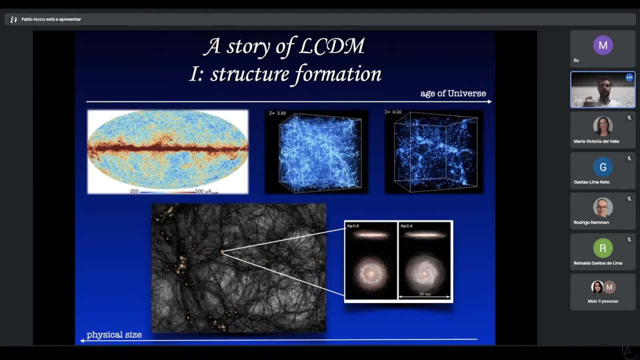 which includes a dark matter fluid and the gases fluid, and I would like to regard simulations as the theory in a way, because this is what we have as the closest to solving the equations is in good match with the observation modulo. some problems which, for the moment, I will not talk about. 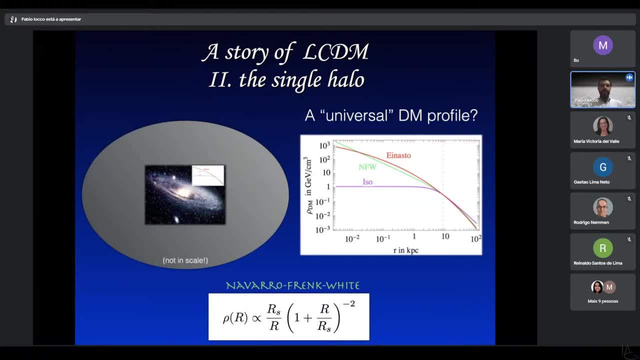 Now, if you look either at the semi-analytical solutions of the dark matter within the structure that we form or at the numerical solutions- and you can do both- you will find out that you expect the gas that forms the galaxies to collapse toward the center. 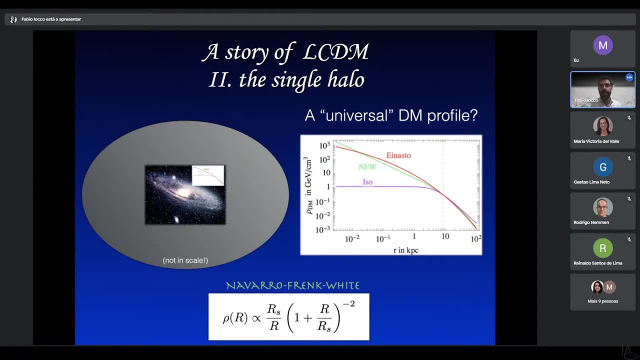 of this gravitational potential, these wells, and to form in the center, in the innermost part of this halo of material, which is mostly dark matter, And in a way, the prediction of how the density, so how the matter or the matter distribution. 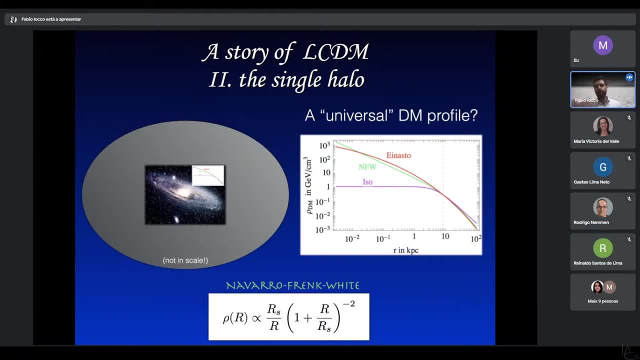 of most of the matter in the halo, so dark matter is most of the matter. dark matter is most of the matter in the halos is something that has plagued or has been in the community for a long time, And whether you have a density distribution. 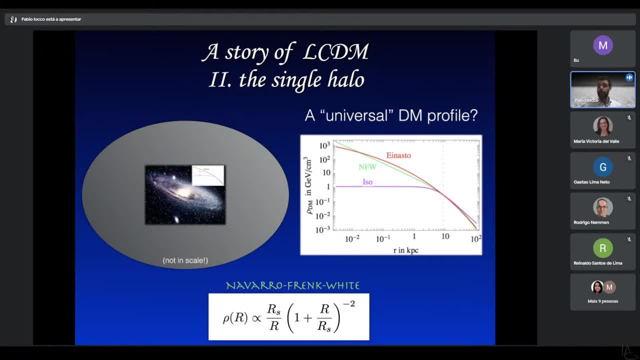 what you're seeing in this plot is density, it's not mass. Of course, mass should go out as you go out at. radius is something that has been discussed in the community for a while, And, in fact, some of the problems about the dark matter. 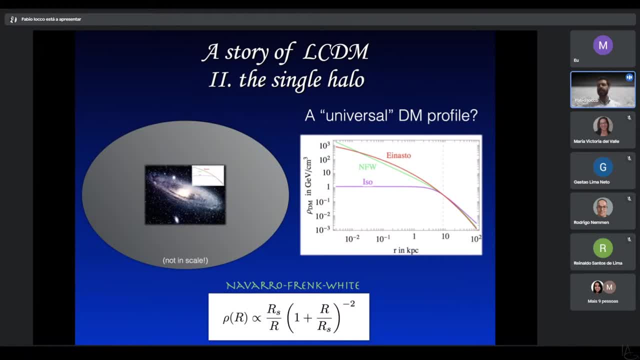 some of the mismatches, some of the frictions between the model and observation was: what is really the shape of the density profile in the innermost parts? Now you might see that this is logarithmic. So when you go to the outermost parts of the halo, 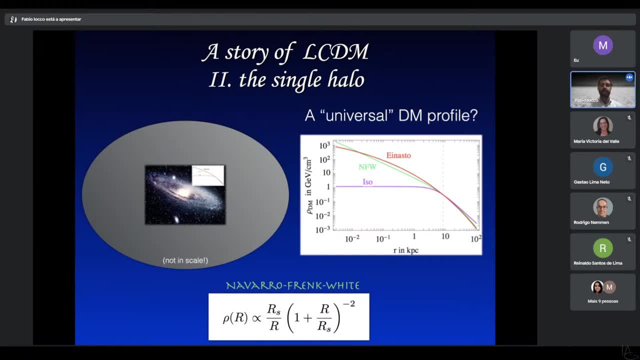 more or less all the inasto, which is observationally inspired, and FW, that comes from simulation isothermal, which comes from the analytical model, with some approximations, but all of them tend to agree that there must be a slope of R to the minus two. 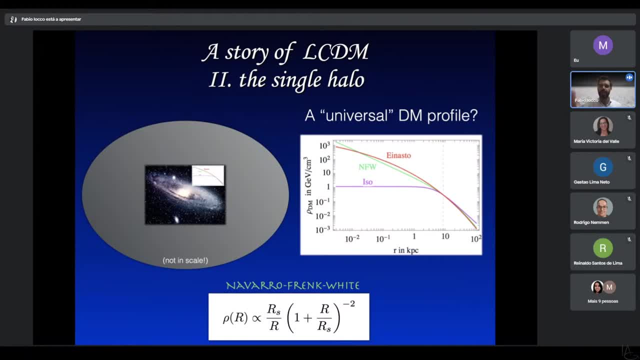 which is fine, which is what you need to justify flight rotation curves. I will get to that, But in the innermost parts there's been a huge debate. Now the scale of this will depend on the size of the galaxy, but for this moment, 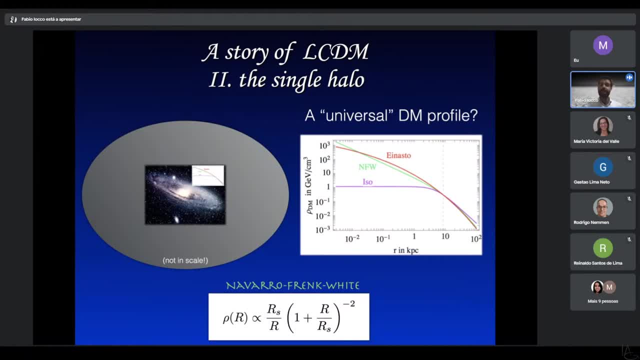 it doesn't really matter. So people have usually adopted this parameterization, which is called the Navarro-Franklin-White- I'm sure you know the name It's. after all, it's a broken power law. okay, It's a parameter that has no scale. 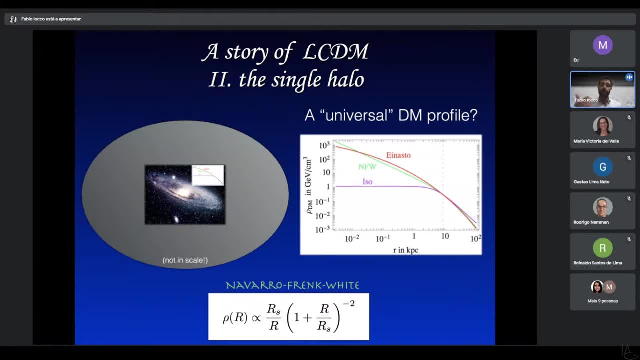 It just has a scale that has to be fixed. So it's self-similar on different orders of magnitude of the galaxy and even in clusters. But the interesting thing you might see here, there is a slope that is fixed. You know R has a minus two slope. 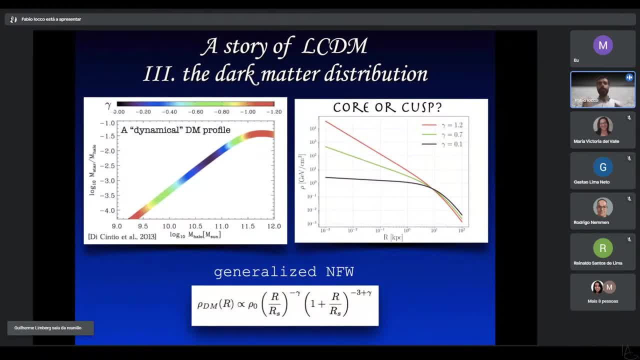 and here there's minus one slope Now. when people started simulating galaxies in the halos- the Navarro-Franklin-White comes only from simulations that include only dark matter- When people have started simulating galaxies inside the halos, 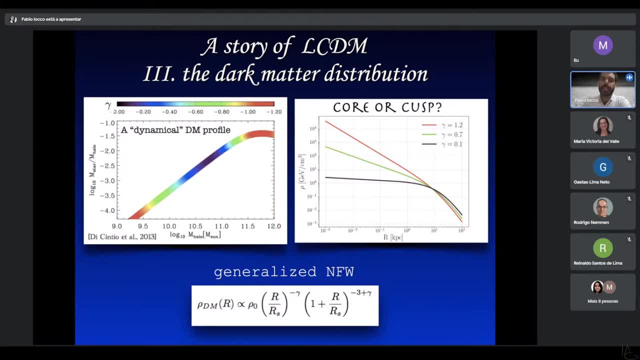 so the formation of an active component. they found that the actual slope that they expect from galaxies of different size in the center of the halo changes And that's because the formation of an object inside the halo. it changes the properties of the dark matter non-trivally. It's still only gravitational coupling, but by collapsing material in the center you will alter the gravitational potential and therefore you expect different slopes, which depend to some extent on the ratio of the halo with respect to mass of stars in the galaxy. Now the color codes in this plot. 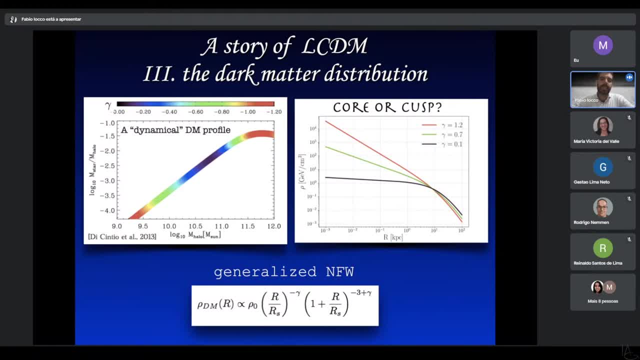 are coded as they are here. So you might see that for a certain ratio of stellar mass to stellar halo, you expect a shallower slope, And for at the extremes of this mass star to mass halo, you expect a higher slope. We can get to the physics of that. 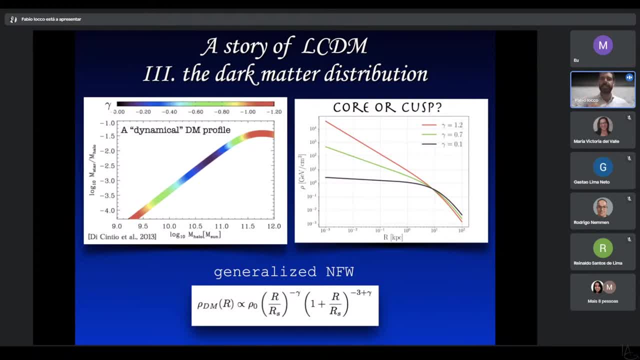 and I can give you references. But the core point of this is that you do expect that the shape, the slope of the dark matter profiles depend, depend on the mass of the galaxy. And, if you want to, this is a second order or first order prediction. 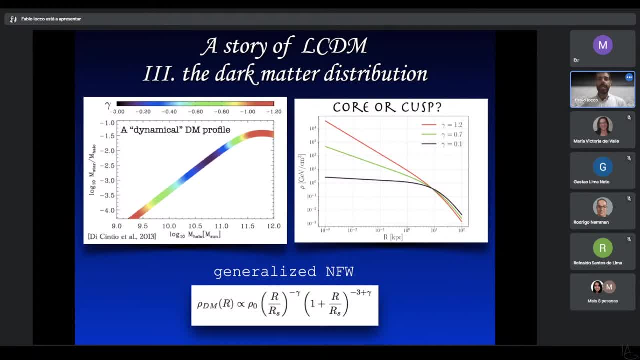 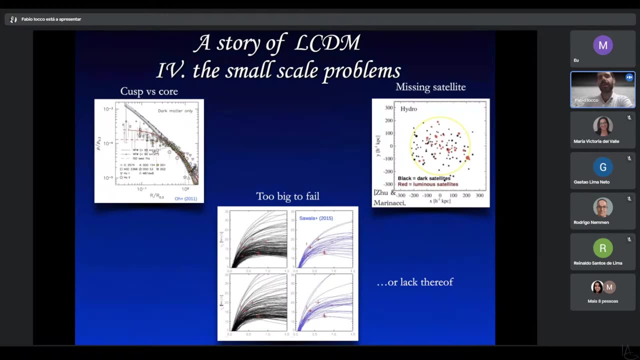 of the Lambda CDM when you start including the physics. So the actual distribution of dark matter within galaxies is something that is intrinsically and intimately related to the predictions of Lambda CDM. Now there's a lot of small scale problems that I have to mention. 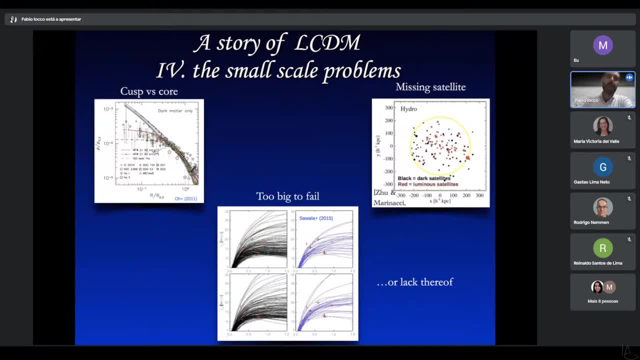 Otherwise I'm going to be crucified later on. I have my opinions on that. I personally believe, on the basic of much evidence and a lot of recent literature, is that the missing satellite problem, that someone who is a little bit more aged than me. 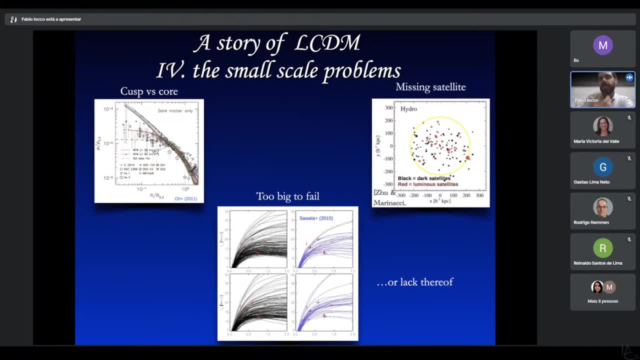 might remember, as a major problem is not withstanding at the moment with the data that exists, either observationally and prediction from simulation. The too big to fail problem can be put in relation with cusp versus course, or whether it's a slope, it's a spike or it's a slope. 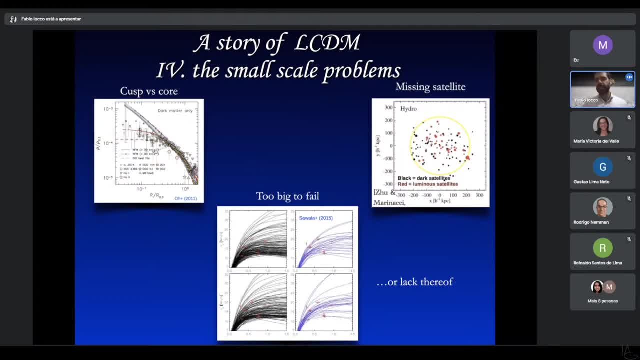 There's different versions of it and they can be discussed, But I would say that numerical simulations today are way more converging towards the data than they were 20 years ago, And that's because we are finding that including the baryons in the simulations. 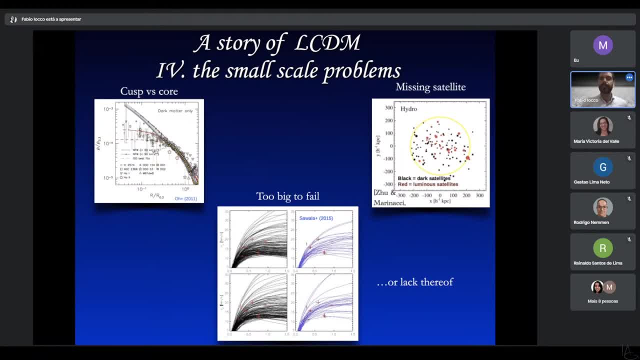 gives a flavor and a prediction to the theoretical standing of the Lambda CDM, which is really incredible. Still, we have no clue about the nature of the dark matter. Whatever is dark matter in the simulations is something like a cold fluid that interacts only with gravitation. 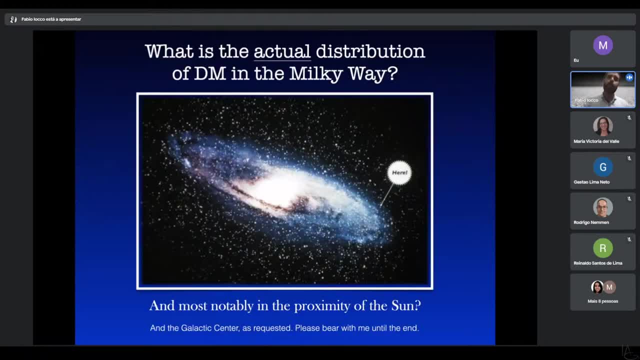 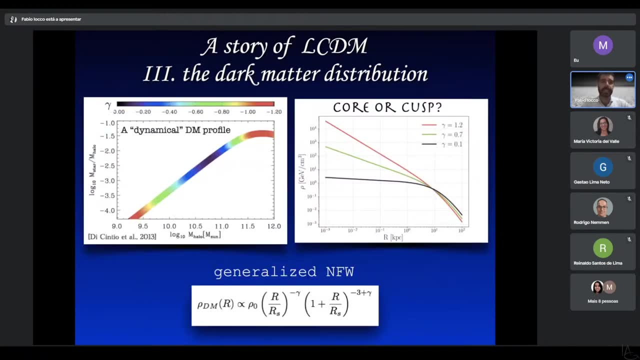 So far, so good, But of course you might have exceptions. Now, why the Milky Way is interesting? The Milky Way to me is interesting because, as a typical galaxy, is somewhere around here. so 10 to the 10, with this M star to M halo. 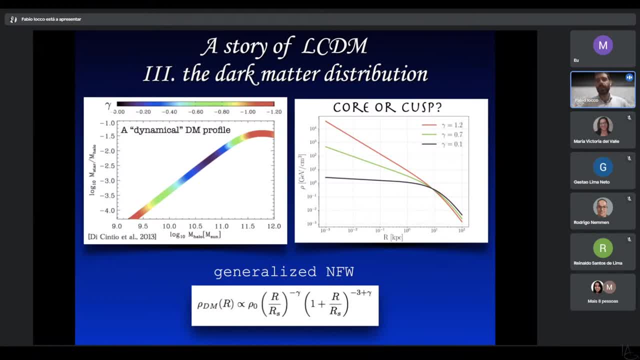 testing the model in the Milky Way is not only a cozy way to comfort yourself and to say, okay, I live in a place which is more or less normal- It's in the median of things- but it might also give you some additional information. 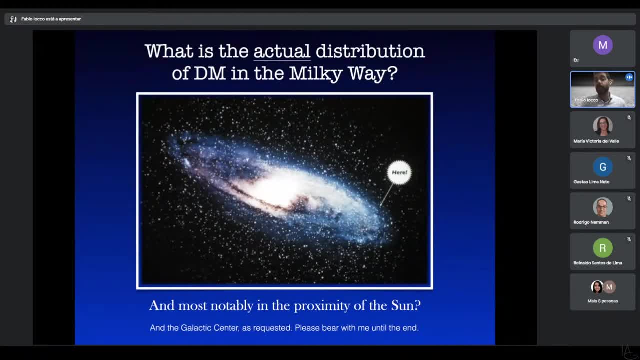 And, of course, it's the galaxy which we have closest. It's a close, close by galaxy. Okay, We might expect some surprises or not, but it's a system that is worth studying as presumably a typical system. Now, why do we want to know? 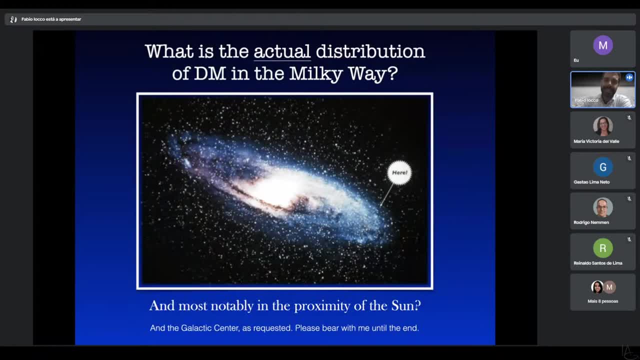 There are other reasons why we are interested in the dark matter density throughout the Milky Way and the dark matter density around the Sun. Now, wanting to know the dark matter density around the Sun is something that it might be extremely interesting for some particle physicists. 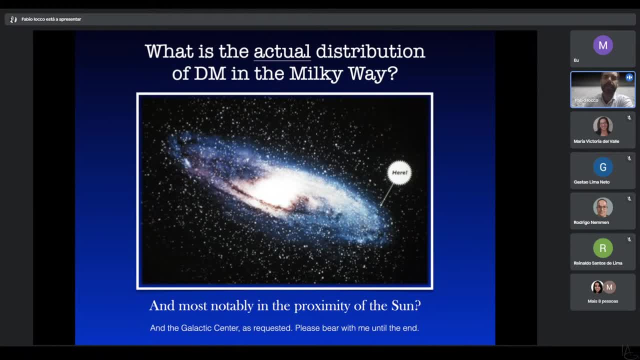 because if you have a specific opinion on what the dark matter is and if you build an experiment that might see the scatter of the dark matter, if it's weakly coupled around the Sun, you want to know what is the specific density of that matter around the Sun. 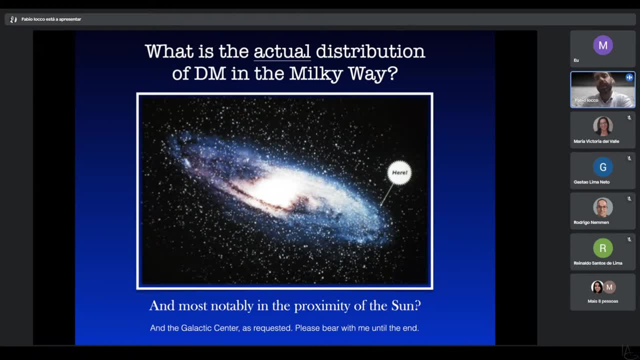 because that's what's going to affect your experiment. On the other hand, you might be interested in general in the gravitational structure of the Milky Way and the dark matter above a certain galactic centric distance. that makes most of the gravitational potential. So that's something that we're still interested in. 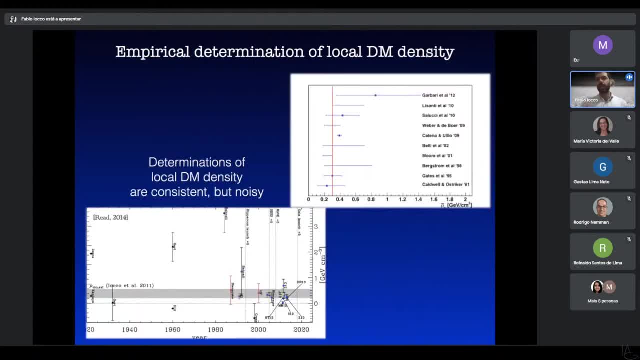 So let's get to the data, astrophysical data. What do we know about the presence of dark matter around us? the closest we can. So these are historical determinations stratified in the plot by Justin Reed. That's a little bit old. 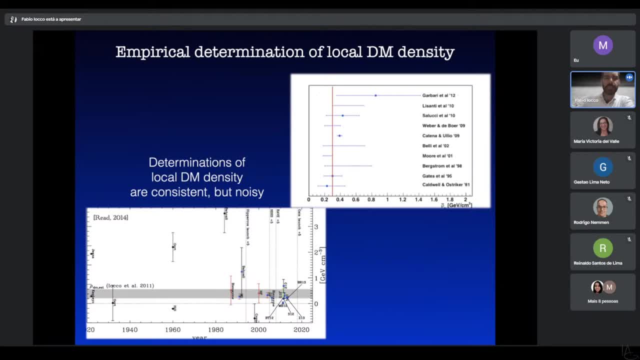 I have another plot, which I don't know if I put here. that I did with my student Maria. That was in Brazil too, And so if you look at the local density of dark matter, that's this axis, is GV per cubic centimeter. 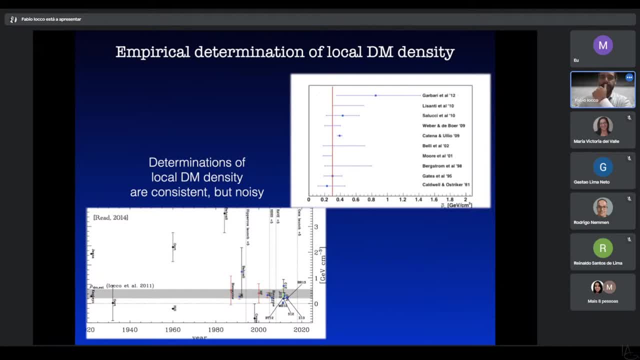 If you like it, in solar masses per cubic parsec. you can see it here. There is the tendency to use a certain value, which is 0.3 GV per cubic centimeter, which is historically inspired, which is this red line. 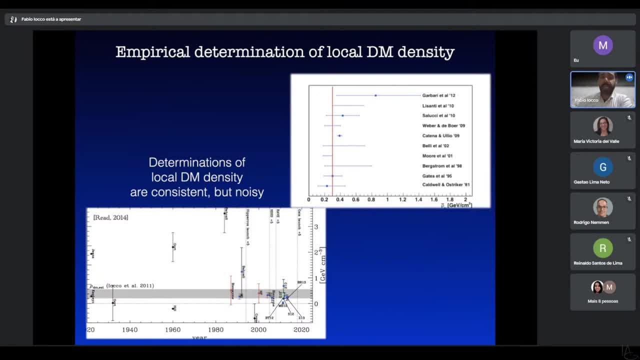 It's just represented here. But the very interesting thing is, if you take different groups and they are listed vertically here, there's nothing on the vertical axis but space to have different groups. They all somehow gather around this volume with big uncertainties And that's a concern. 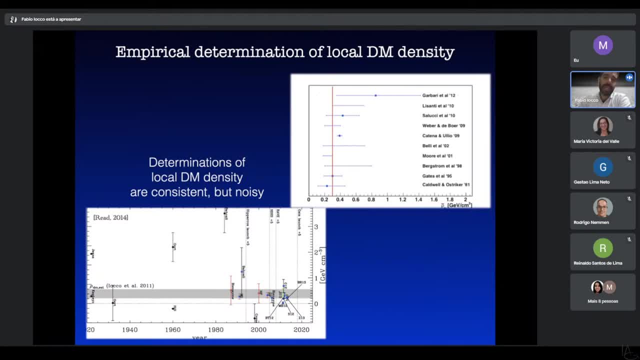 And, as you might see, some of these are actually compatible with zero at two uncertainties. I'm not calling them sigmas because they're not not. all of them are statistically uncertain, So I don't feel comfortable in calling them sigma. But the thing that we noticed is: 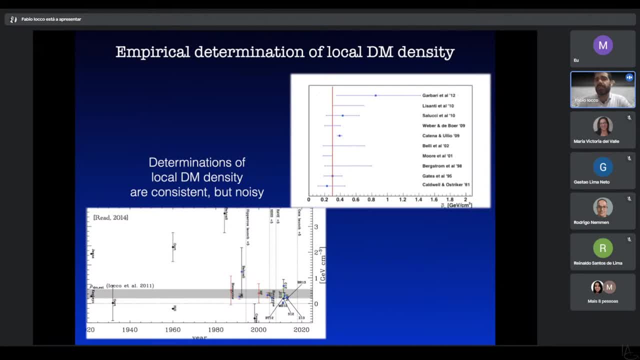 look, it's true that all the central values are up and they seem to be somehow close to these historical values- 0.3 GV per cubic centimeter- which, funnily enough, is close to the earth value and the captain value. 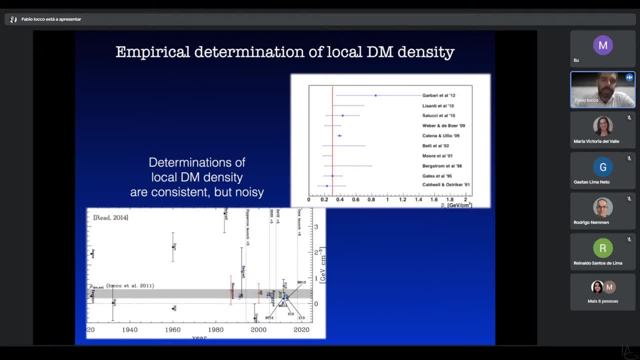 but it's also compatible with zero. So do we have or do we not have that matter around the sun? Does this infringe the paradigm that is coming from the Lambda CDM? What does it say? How is the Milky Way located in that plot? 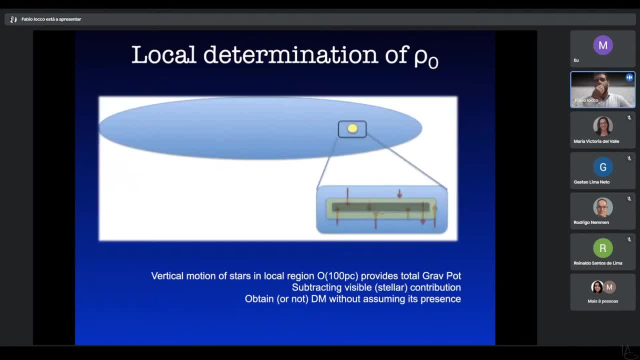 Where would it show? What do we know about it? So there's been different ways to answer this question. We set up to the task to try and understand how the different measurements are done and if we can improve. Now there is the local determination. 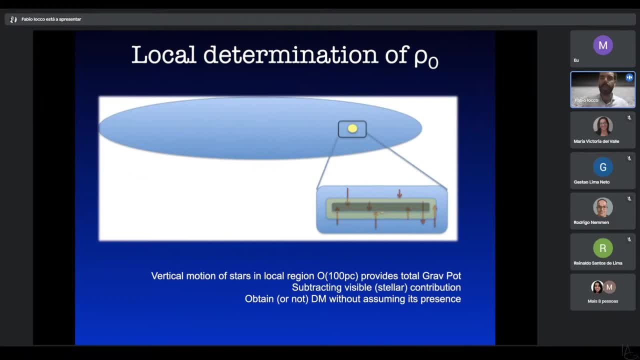 of the dark matter density, the local dark matter density which I call Ronaut, which is done by measuring the movement of stars in a slab and around the sun, something like 100 parts a quiche. And then, if you can measure statistically, 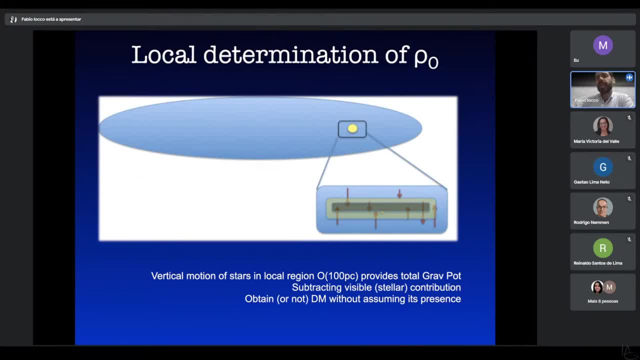 the movement of the stars up and down. you know that that's caused only by the local gravity in the disk. There's a lot of assumptions that you can make and justify about the shape of the Jeans equations if you pick the right tracers. 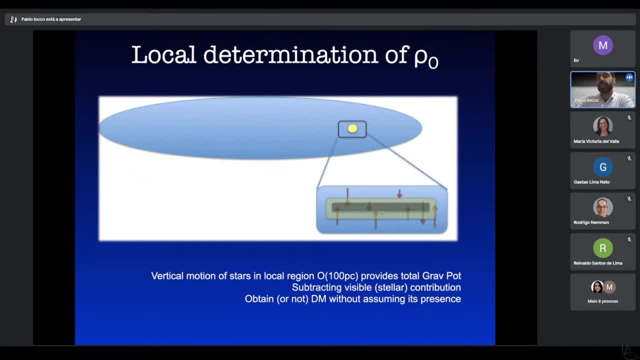 And so you will know that it's just. it just depends on the local slab of matter. Now you measure the stars in the disk around the Earth so you can subtract. you can subtract the yellow slab and then whatever is left is the black thing. okay, 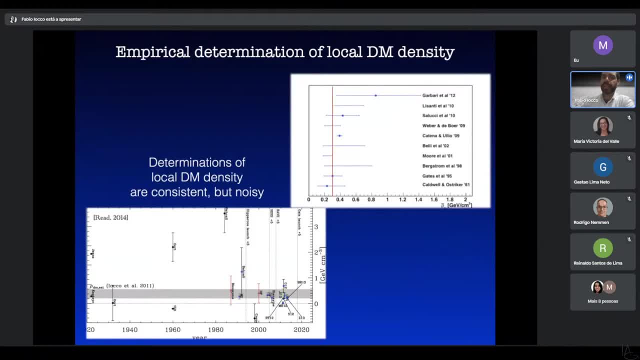 So this is the local determination of Ronaut, and is the one that gives the biggest uncertainties. Now, the good thing about this method is that you are not making any assumption of the presence of that matter. You're just solving the Jeans equation. then you're subtracting. 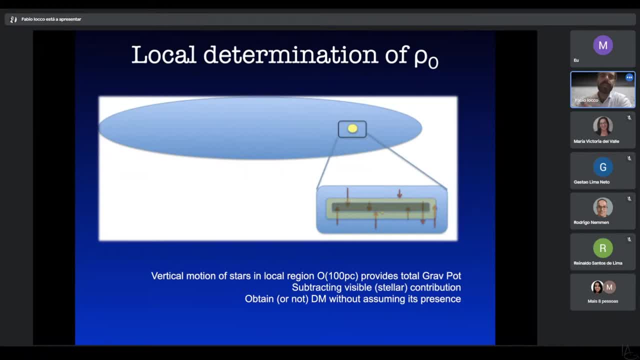 the gravitational component from the stars, And if it comes bigger than zero, then you win because you made no assumptions about the component. okay, The drawback is there's a lot of big uncertainties, especially systematic uncertainties, but the drawback is that it's only local. 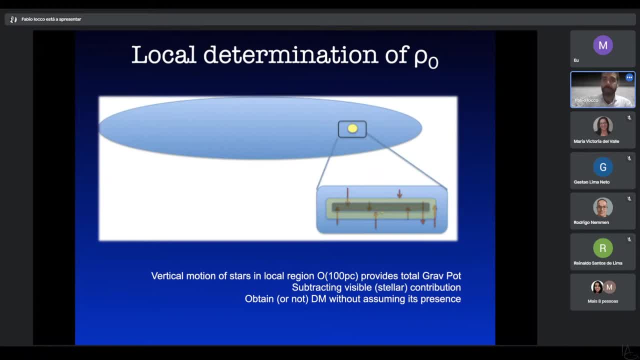 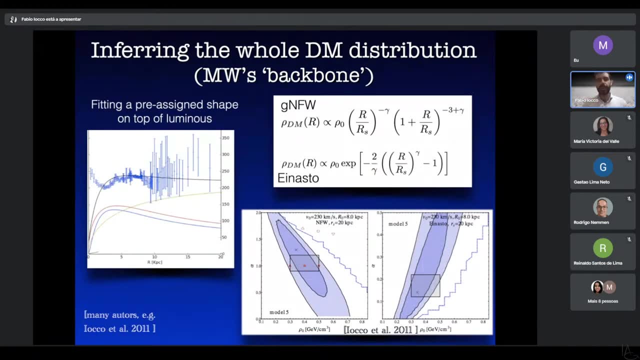 So you can only learn about the density around the sun. Now, instead, you can use the very well-known method of the rotation curve. and now the primer about this- for those who don't know about it- is that if there is a disk, 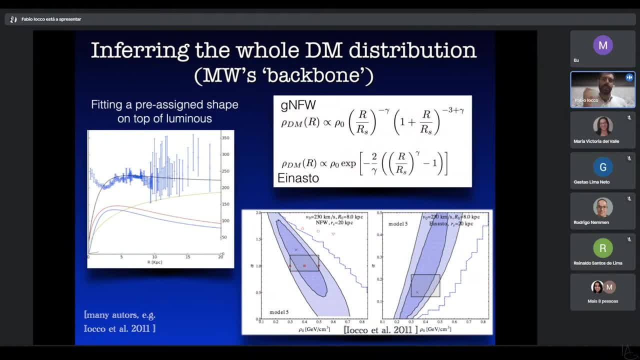 a galaxy is a disk. you know that this disk has to be in balance with rotation, So there is gravitational pull and basically centrifugal force, and stars do not go away. the disk exists So by tracing the velocity and therefore the centrifugal force. 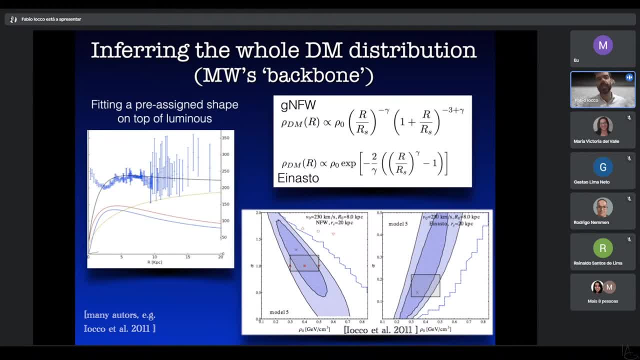 at each point you can trace the enclosed mass, okay, So one convenient way is to plot the velocity And, as you can see, the velocity stays constant, more or less constant, even when you get out of the stellar disk, which is 10 kilopascal. 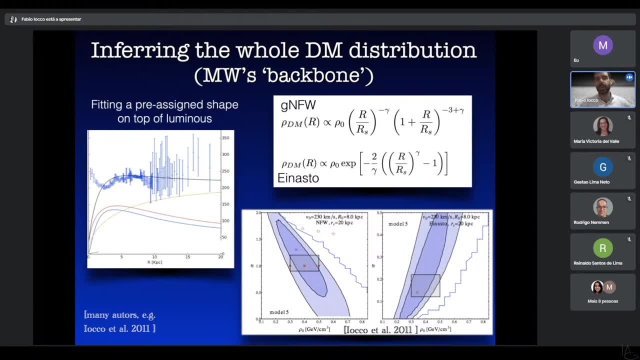 And that means that it's interpreted like there is an extra component, which is the yellow, whereas the red and the blue are the components that you expect from different visualization or different realization of the stellar disk. okay, So we see the stars we model with Newton. 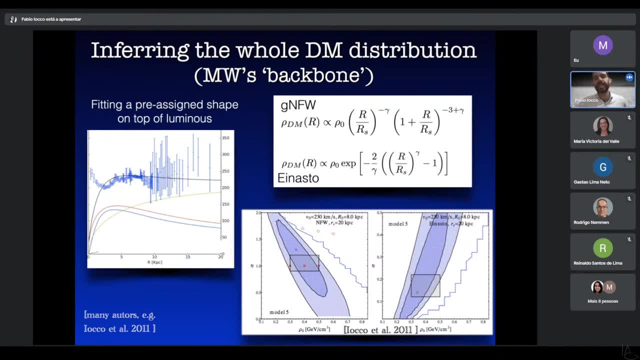 we predict the velocity we would expect from the stars, and that by no means fits the curves. Now that gives you the possibility to just take a shape like the one of GenFW for this additional component and fit few parameters on the top of the stars. 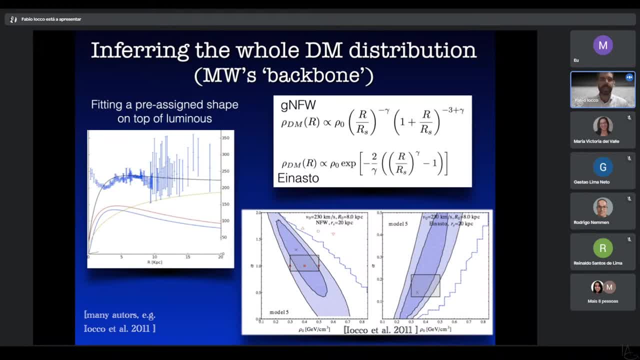 to whatever best fits the data. That's what people have been doing, that's what I've been doing even in 2011,. so it's actually 10 years. I was right, it's 10 years. And then in the parameter space, 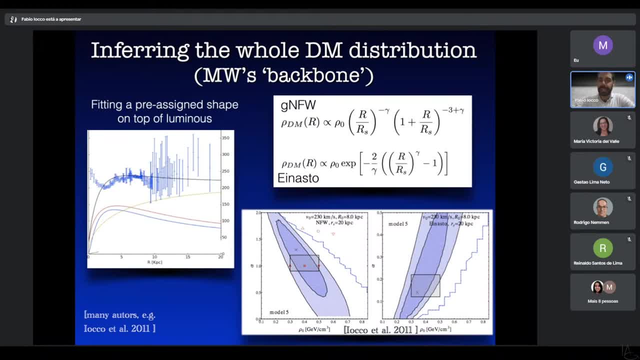 of where you have a slope alpha and you have a density on the x-axis. what you get is these contours. Now, this box is what it was suggested for. a Milky Way halo in a simulation- not, I'm thinking, the Milky Way. 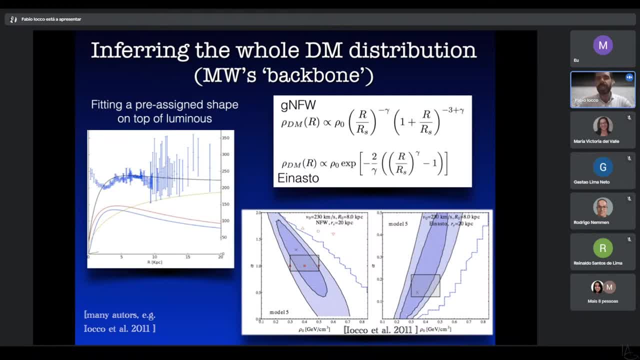 so a Milky Way-like halo in a random simulation. They would suggest this parameter space, this box for a Milky Way-like object, and what we got from the real Milky Way was something like this that nicely fit within the prescription of the predictions of the simulations. 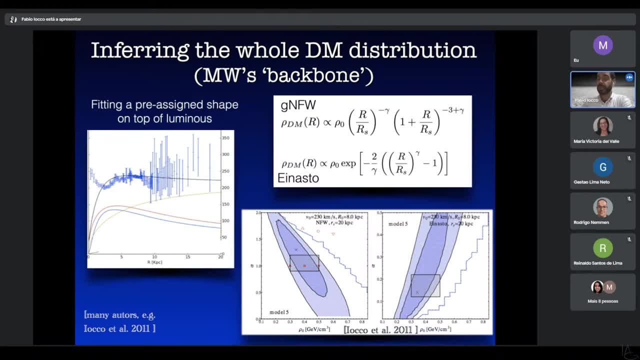 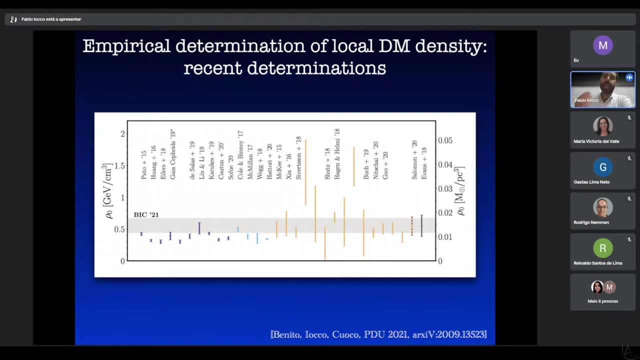 So this was very nice, it was very good, it was 2011,. it was a very good piece of work and I will explain also a little bit how we did it. And the thing is that today, what we get in updating that plot, 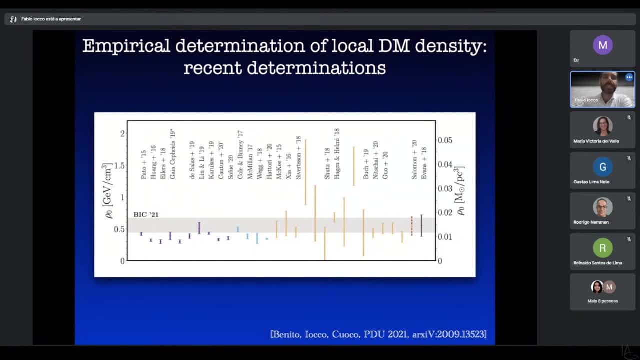 that I showed you. 10 years later, we're still somewhat in the same situation. We have determinations with relatively small uncertainties that are more or less the rotation curve needed. we have local determinations that give you big, systematic uncertainties, and they all more or less 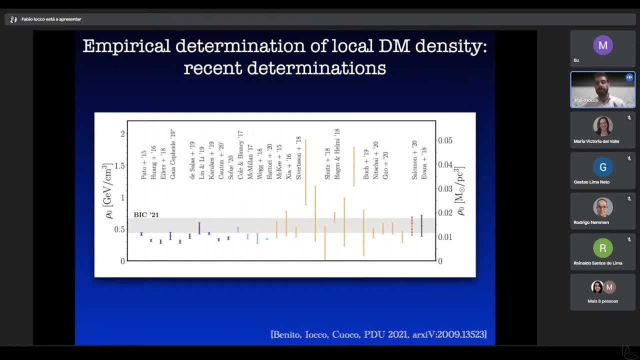 go around the same volume. their central values are more or less stratified around 0.4, 0.5 GeV. but there is one thing that I didn't mention, And the important thing that I didn't mention is the following. 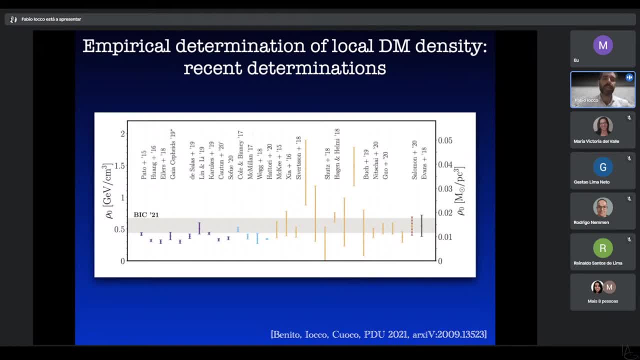 If you want to be certain about how far away this is from zero, so how certain that this is five sigma away. this is a sigma and you're five sigma away from zero around the sun, so you are absolutely certain that the gravitational potential of the stars. 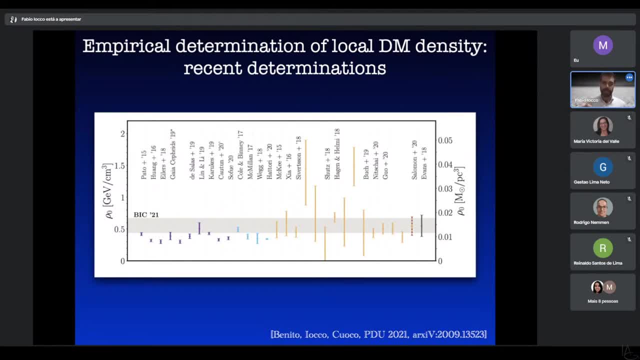 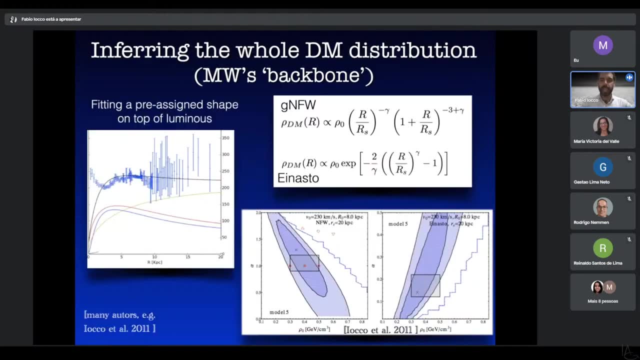 at the position of the sun in the galaxy is not enough to sustain the rotation of the galaxy. there is something more that you have to do Now when you do this sort of game. so you try to infer the local dark matter density by fitting the total shape. 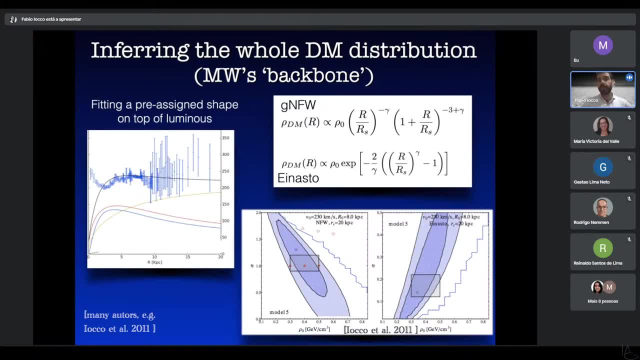 that's nice, on one hand, because you're getting the total shape in the whole galaxies, not only the local one, but it's bad because, contrary to the local method, you are making the assumption that dark matter exists. You are fitting the power law. 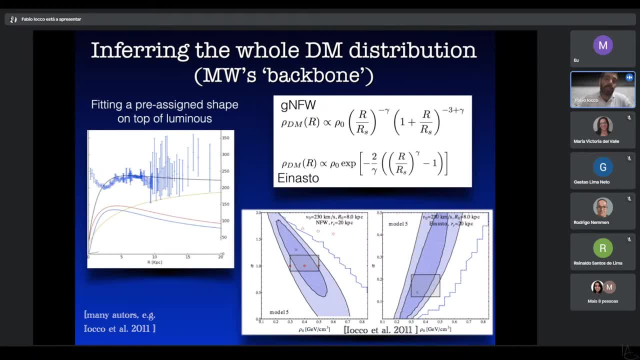 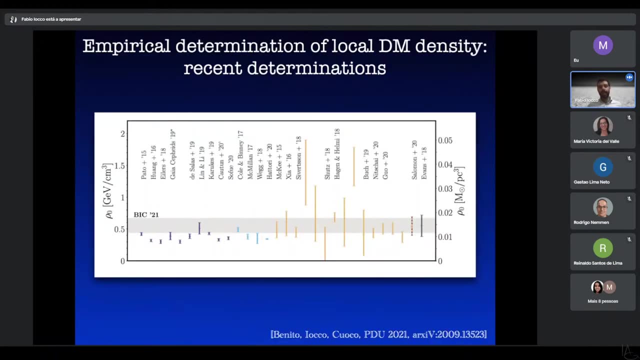 which is a non-zero power law on the top of the data. So there is an answer. So you are plagued by somehow, to some extent, that is possibly quantifiable of your answer. So what we did in order to get as possible, an assumption-free answer. 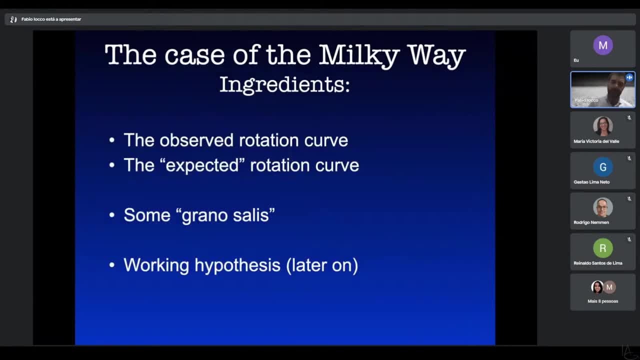 about whether there is dark matter or not. we did something very simple. We started. this was something that proceeded from the work we did in 2011.. We consulted with a lot of colleagues and they thought it was an interesting work to be done. 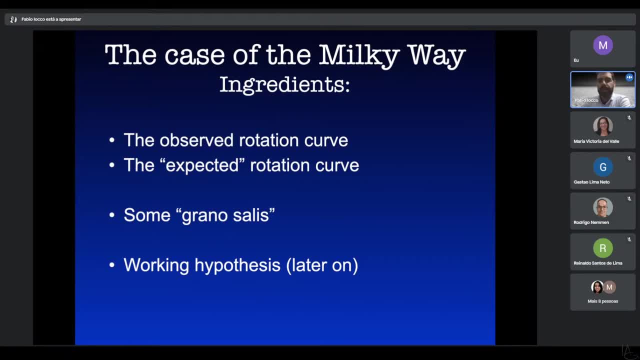 So we reclassified all the observed rotation curves, data that existed Then independently we modeled the expected rotation curve. Now the expected rotation curve is not that theoretical. I will show you how. this is only data inspired, So there is no theory besides Newton. 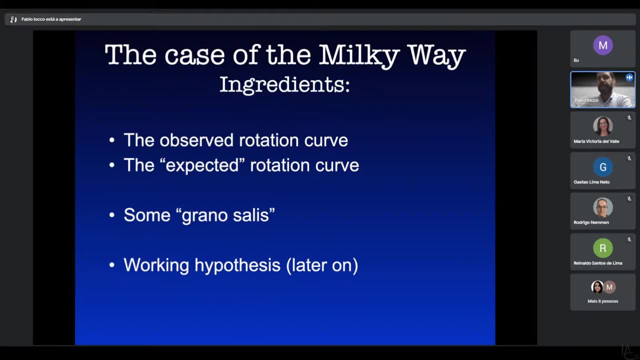 Okay, And then at some point we made some simplifying assumption that do not include the existence of the dark matter. So we did not assume the existence of dark matter up to the point at which I will specify it. Okay, So there's different tracers. 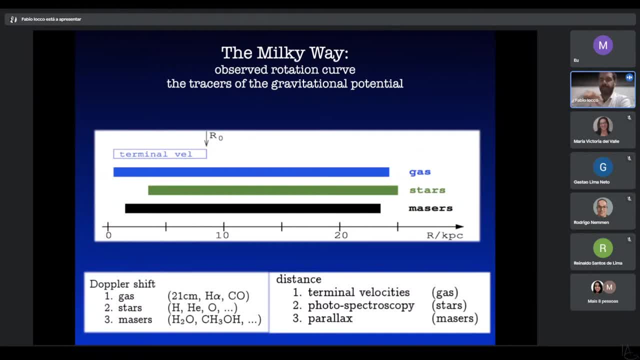 that trace the circular motion and they're distributed differently with the radius as it comes from the distance from the galaxy. So you have gas clouds, you have stars, you have masers, which are gas clouds, And technically speaking, also stars are gas clouds. 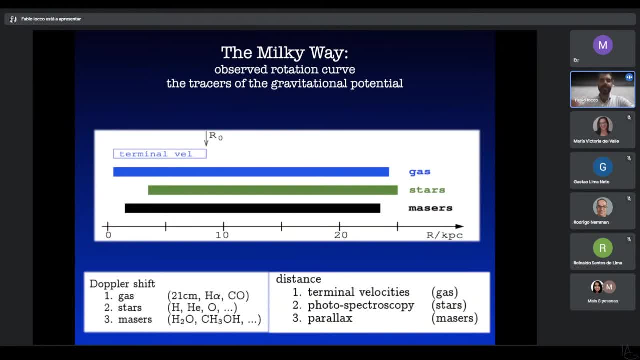 but we can understand each other. So there's gas that you can measure in optical or near optical absorption, There are stars, by themselves observed as stars, and there is masers- Okay, And they are distributed different ways, with different characteristics, And you can collect them together. 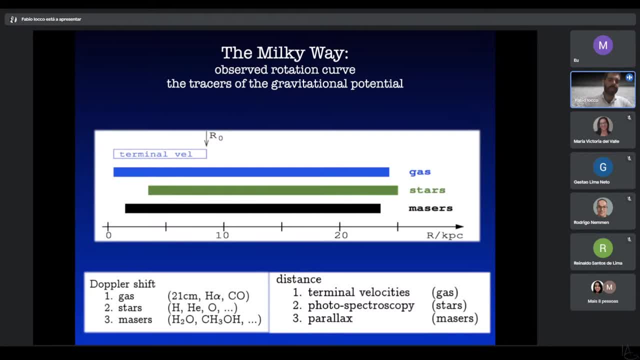 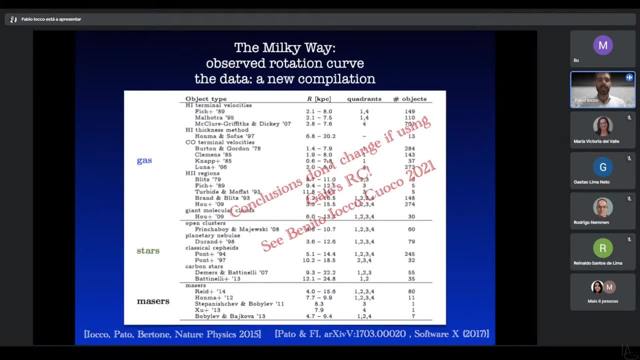 Now it's possible that some type of these tracers are affected by some systematics, Okay, And some other traces are not. So we put all the data together and we produced a nice gimmick that allows you to look only at certain type of objects. 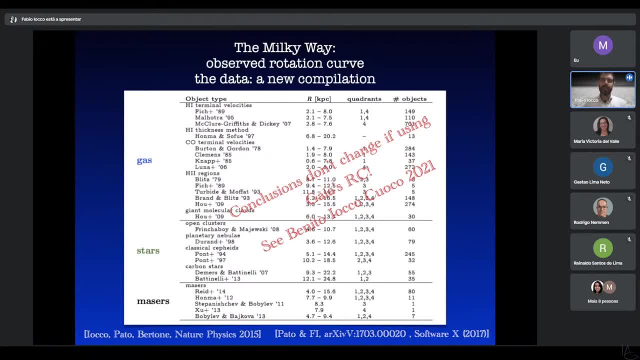 And the important thing is that when we started removing either randomly, data sets or systematically- so we did not consider the gas, we did not consider the stars, we did consider only the masers or any sort of combination systematic study- we always got the same answer. 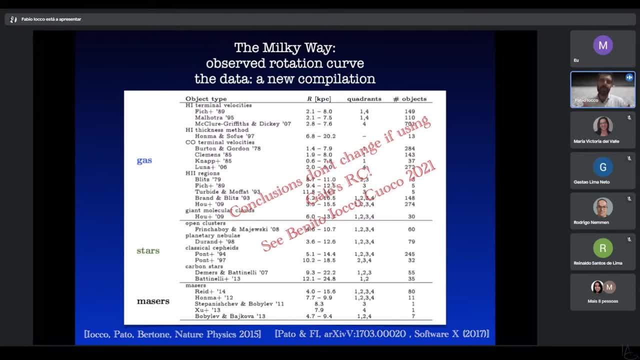 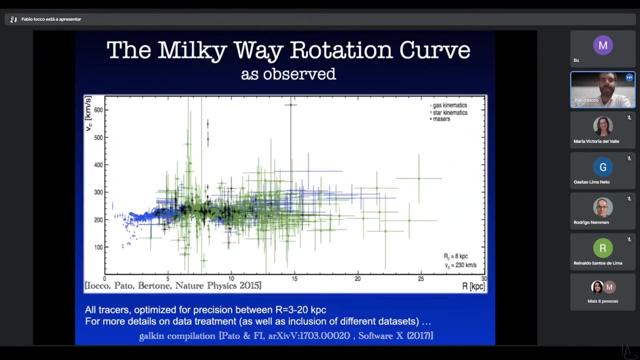 The statistical strength was different, of course, because we had different data, but the answer was all the same, So we knew that the data were consistent. We also did a very an extensive compatibility study later on with the Trotta group, But this is safe on statistical basis. 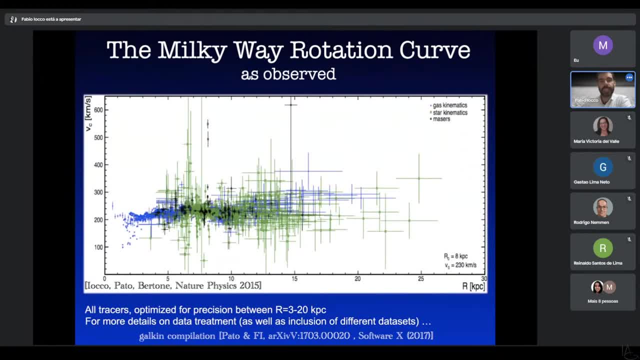 So what we did is we put together all the data and this is the observed rotation curve And, as you can tell, even by eye, it's sort of flattish and it doesn't go down out of the galactic disk. that extends up to 10 kiloparsec. 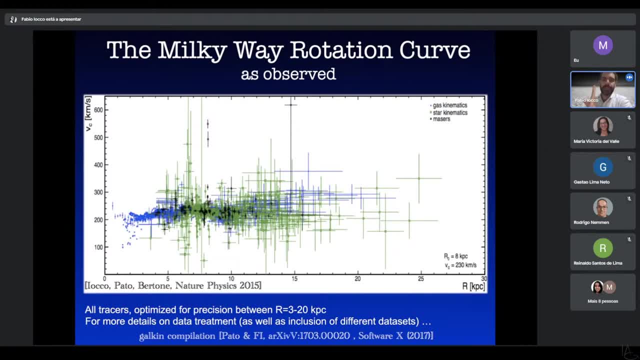 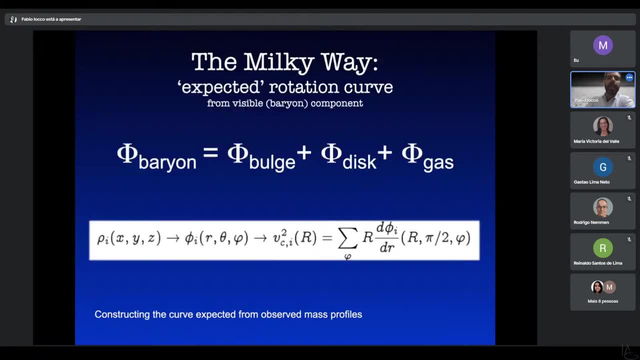 And this is by no means the interesting part of the work. This is just compiling data. Unfortunately, at the time I was a postdoc. I was not a graduate student, so I had to do it myself for real. But now comes the interesting part. 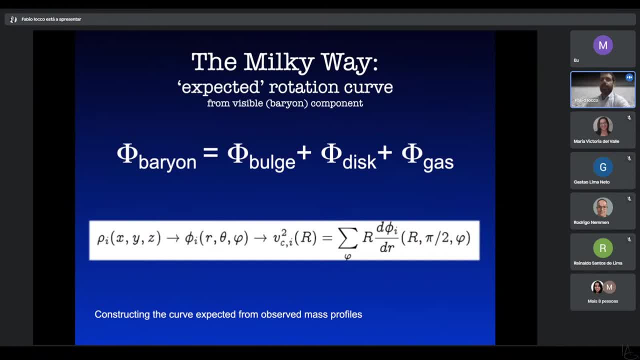 What is the expected rotation curve? The expected rotation curve is what you expect from the visible component, because it's visible and it's there. And, of course, you can split up the galaxy just in components, By the way you observe them and you decide to put them together. 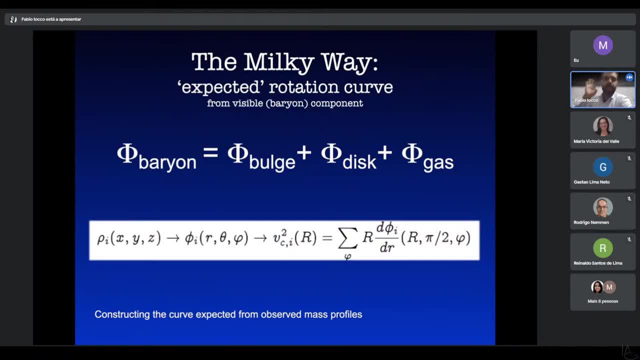 But they're all there. There's nothing that we add on the basis, or it should be there, It's just observed components. You usually split it in bulge, disk and gas And then from the density you can infer the gravitational potential. 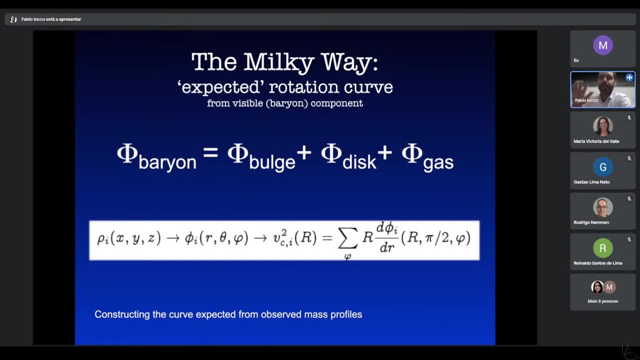 assuming that it's Newtonian. It's a full 3D reconstruction of the gravitational potential And then we compute what is the component in the disk. But we do not make an assumption of non-spherical symmetry. That's not one of the assumptions. 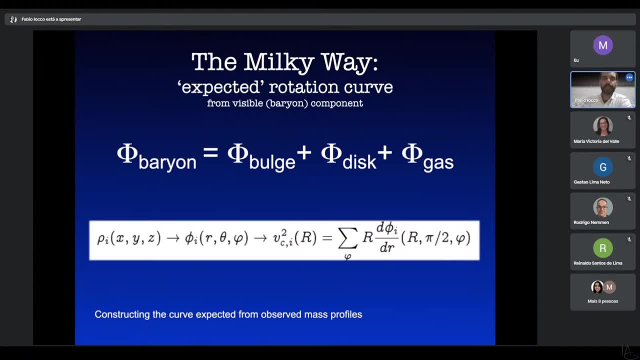 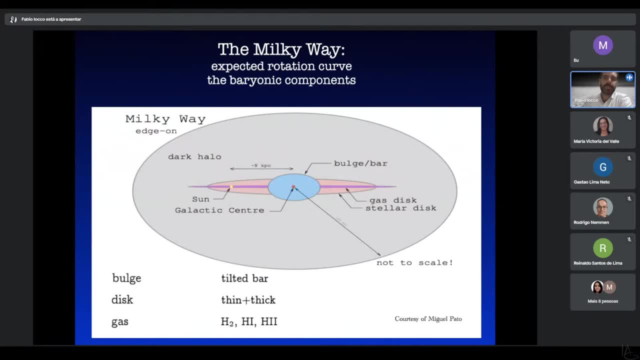 we make, It's a full solution of the 3D potential. Okay, Now it seems that this part is the simplest, So the visible component is the colorful one. So you see the bulge which is central. You see a disk of stars. 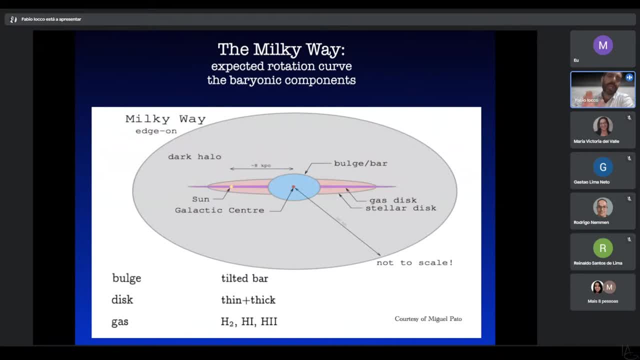 a stellar disk And then you see a gas disk. Now we included the gas disk because it's so absurd. But, to be honest, gravitationally speaking it's negligible, But we include it anyhow. There is uncertainty associated to that. 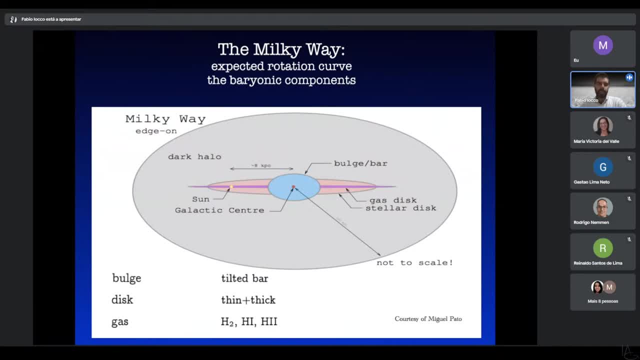 And now it comes to the treatment. Now, when we started with this, we thought that there was no agreement. There was a little debate about what was exactly the shape of the bulge, So we called our astrophysicist friend. 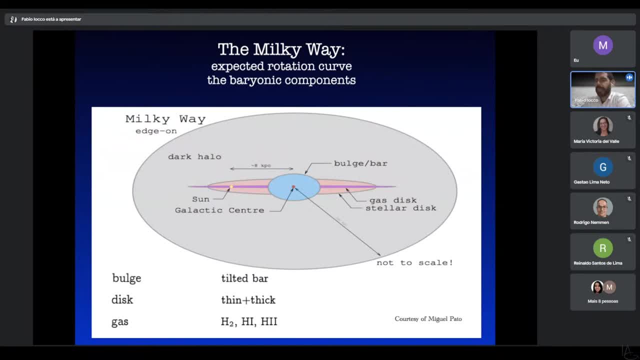 our observer and he said: no, no, no, no, no, no. There is no debate at all. There is only one bulge model, the one belonging to my group, And we called someone else who said exactly the same thing. 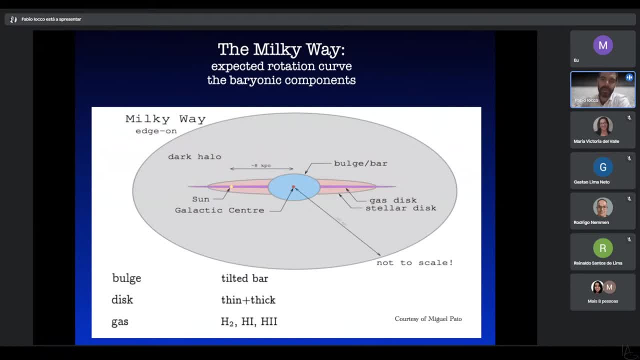 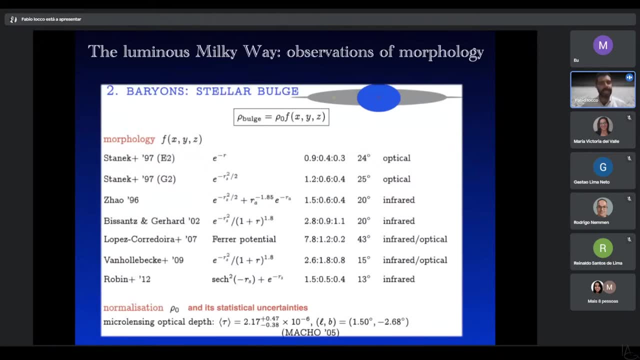 He said, yes, the bulge, the good bulge, is the one from my group And that extended to several groups. So we realized that of course there is no debate. The important thing is to pick all of them and not do anything with them. 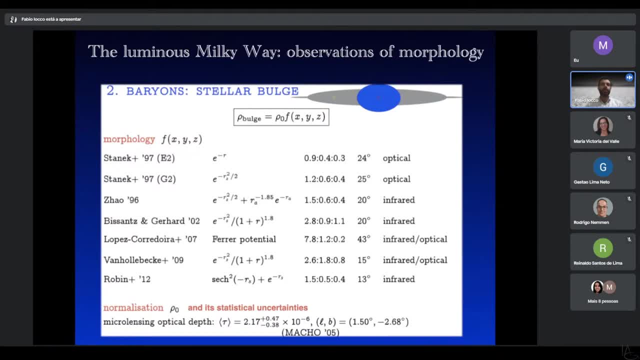 So if you want to be conservative, you have to allow for the possibility that the systematic uncertainty on the stellar component of the bulge is the uncertainty that derives from the bracket of all these models. We do not fold them, We do not weigh them together. 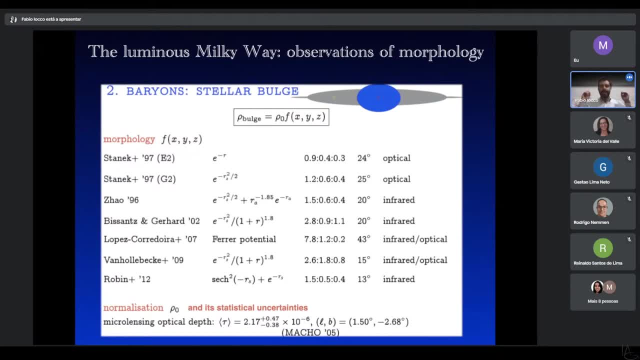 We just say our ignorance is the systematic. The systematic is our ignorance. And it's how far apart, Worst case scenario, the smallest or the biggest, But each one of them carries a statistical uncertainty. Okay, So the way we normalize this bulge, 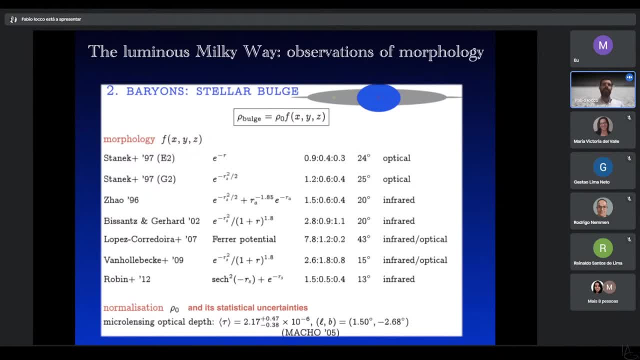 is by using microlensing optical depth. I can get to the details of that, But the important thing is that each single bulge, stellar component in the bulge, carries a statistical uncertainty, And there's several of them, Okay, Which we do not mix. 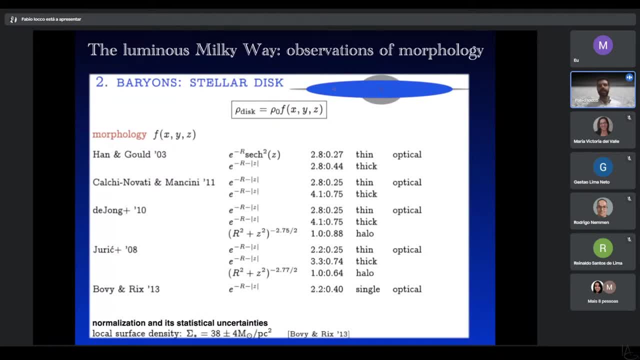 Same thing with the disk. Of course every group has their favorite disk, So we consider the systematic, all the possible disks. We do not average them, We do not mix them in any way And each one of them carries a statistical uncertainty that comes from a local surface. 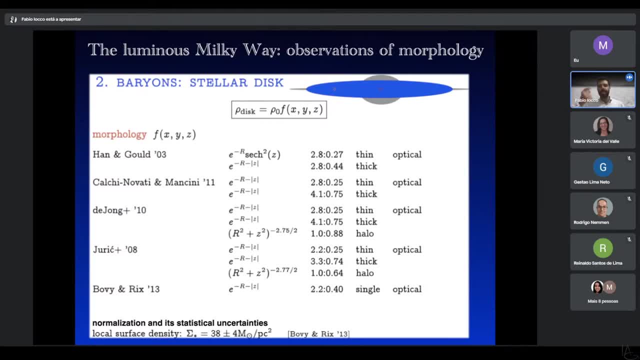 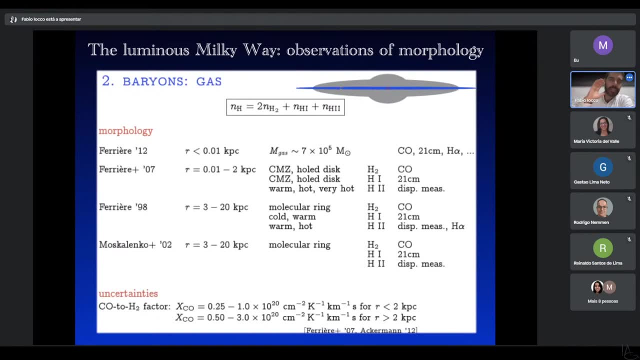 density determination. So it's not a microlensing anymore, Although the disk enters in the calibration of the bulge. it's exquisitely technical. Anyhow we get to this, There is the gas. Thank God there's only two or three models of gas. 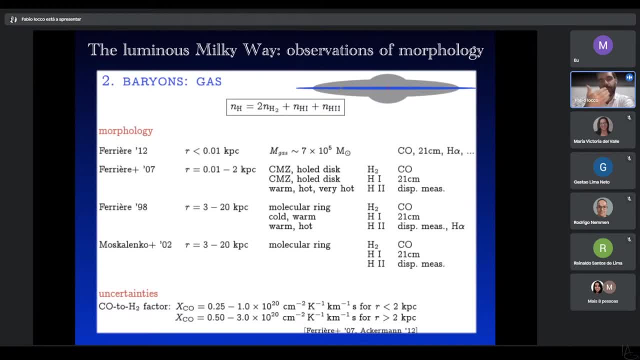 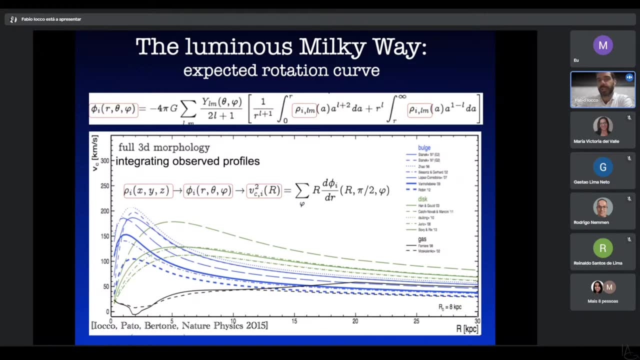 not as many as the others, And it doesn't really matter, Although we include that the uncertainty. So what happens now? What happens now is that you have all the blue are alternative to each other, All the green are alternative to each other. 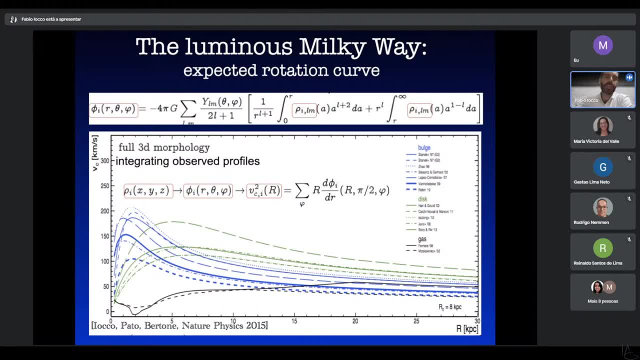 And the two black, which is the gas, is alternative to each other. What did we do So? you have an index A, B, C, You have an index I, J, K, O, O, And then you have an index. 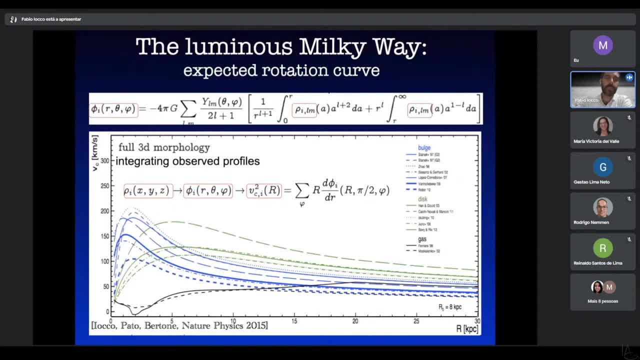 also say these are numbers: one, two, three, four. The blue is numbers, Then you have letters A, B, C, D, And then you have alpha and beta, And so each possible representation of the galaxy in stars. 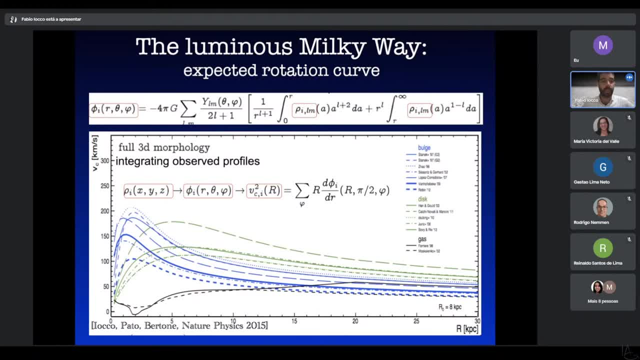 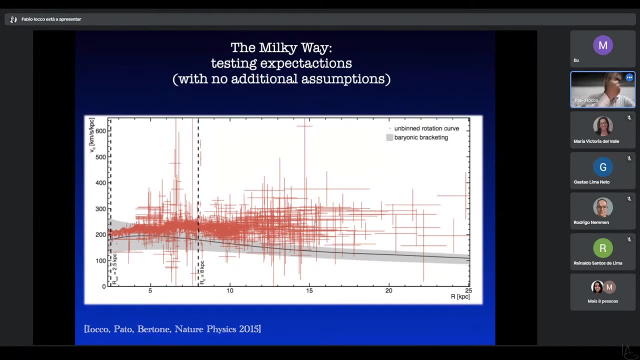 is one combination of the other, of the three, And so you just permute all of them and you take them independently. Each possible realization will have a statistical uncertainty Well posed, And so what you see here, the black line is the central value of one component. 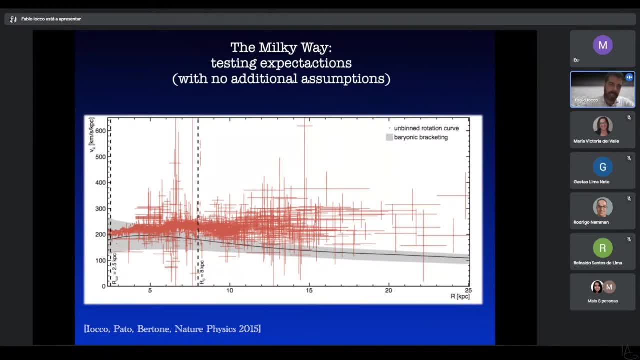 Then there is a gray line here that you cannot see. There's another gray line here is another possible component. So you will have- we call it alternative morphologies, Okay, Each single alternative or possible morphology of the stellar component, of the visible component. 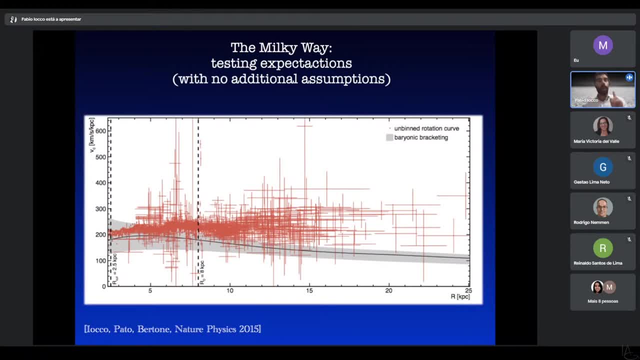 carries a well-posed statistical uncertainty. And now, one by one, so separately, we tested the null hypothesis. So there is no dark matter, We don't know it, We're ignorant. There is no dark matter, It's just stars that we observed. 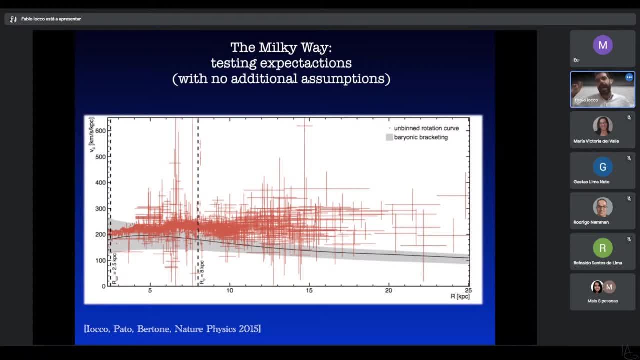 It's well-posed to use Newtonian gravity And there is a rotation curve. I'm assuming there's a balance between centrifugal force and gravitational force And we tested the null component. Can one morphology account for the rotation curve Parameter less fit? 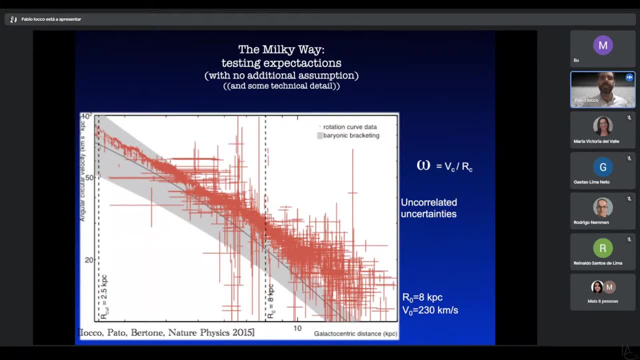 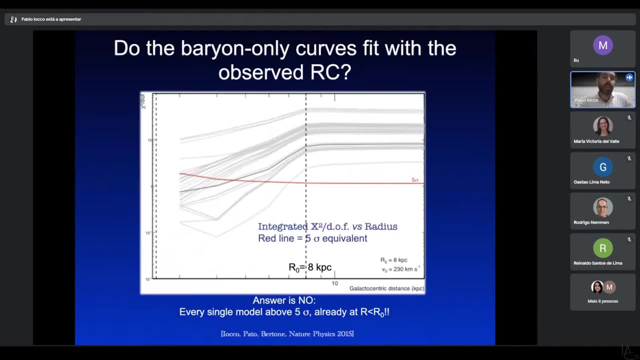 Okay, This is the same rotation curve seen in logarithmic scale Parameter. less fit, each one of them independently. Okay, So I have a goodness of fit for each one of these possible components And, as you can see, and as you can see, 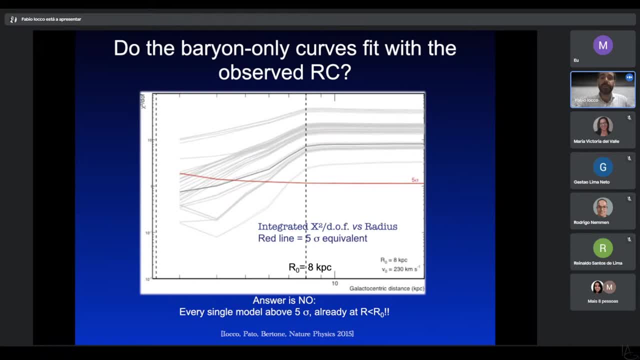 the chi-square per degree of freedom goes very bad above the five sigma line, even inside the solar circle. So that's the zero assumption, That's the zero order. We need that matter. We need something additional to sustain the rotation curve, even within the solar circle. 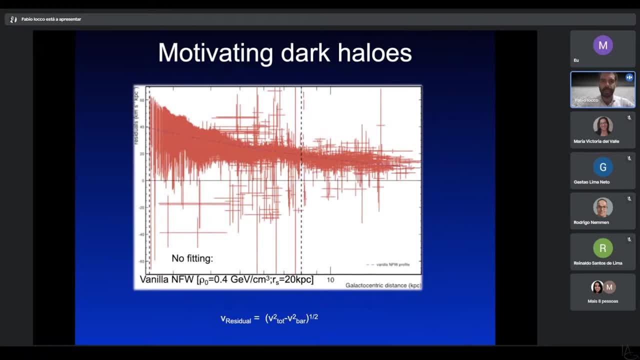 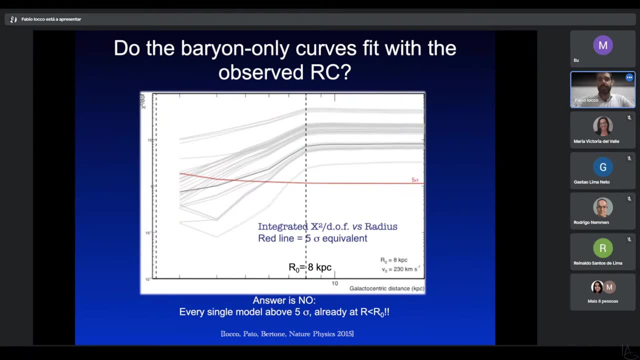 This result is solid for change of galactic parameters and a lot of other things, And so, once now that we have a good confidence of the fact that there is a dark matter component, which is simply the fact that stellar component cannot account for the rotation curve, 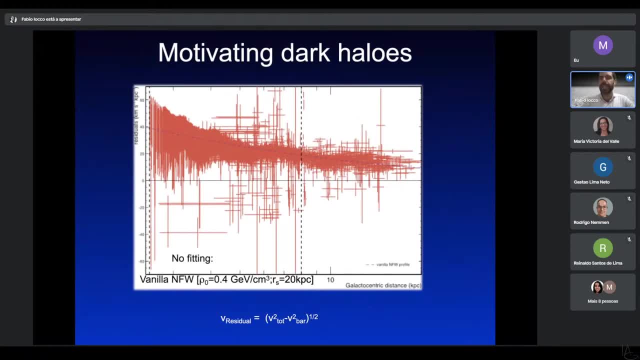 we do allow for the possibility of a halo, And we do it because if you take the residuals between the observed rotation curve and any stellar model, they go like this: This is the residuals. And if you pass a standard NFW normalized to the canonical value, 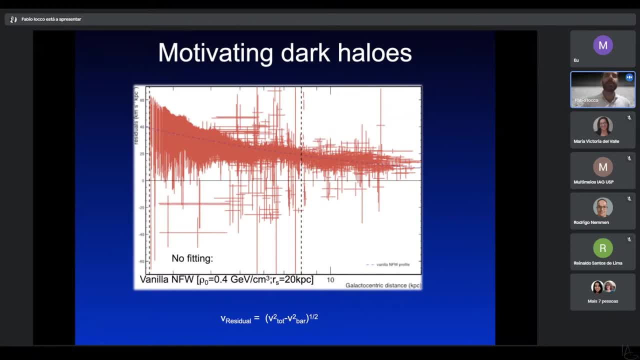 it just goes in the middle of it. No brainer, We're taking something like just a number from the papers and it just goes through it. Now, of course, this is no good motivation, but it's clear that it tells you that you're going in the right direction. 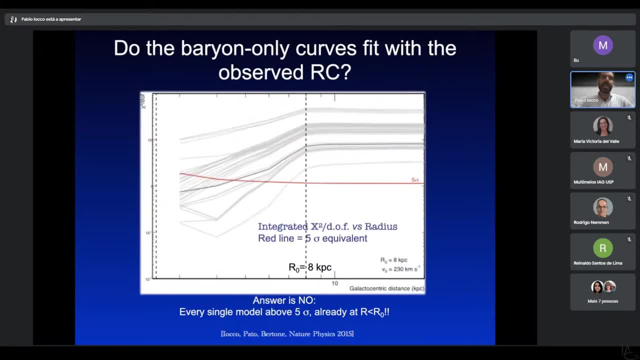 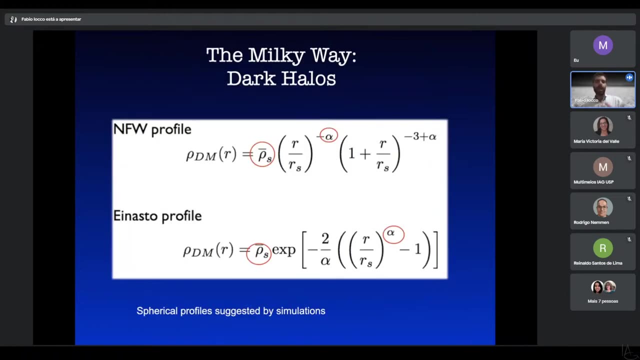 So, for now, the take home message is: there is no way, absolutely no way, to accommodate the rotation curve of the Milky Way, even within the solar circle, even within the solar circle with the stellar component alone. Okay, At this point we decide to add: 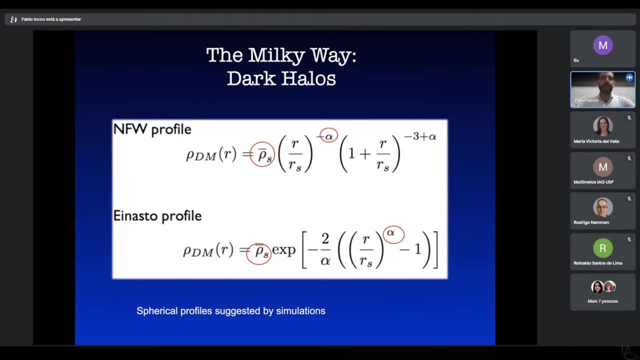 on the top of the game, a dark halo. It might either be an NFW profile, which is parameterized to the density and the slope and the scalar radius, or an anastro profile which has a slightly different. all in all, they're just broken power loads. 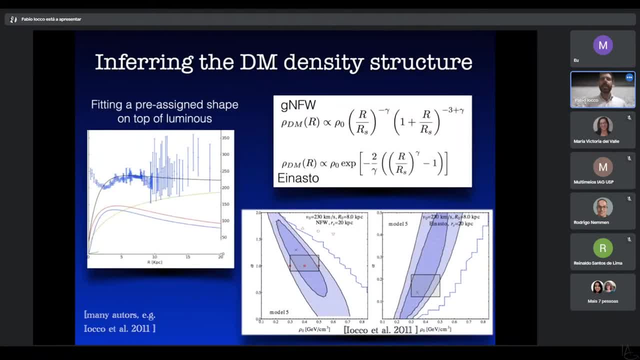 with different characteristics, for use for convenience, And what we did was the same game that I showed you for even a morphology. on the top of it, we add one dark halo and we try to get the best fit for the parameters. Okay, The problem we have now? 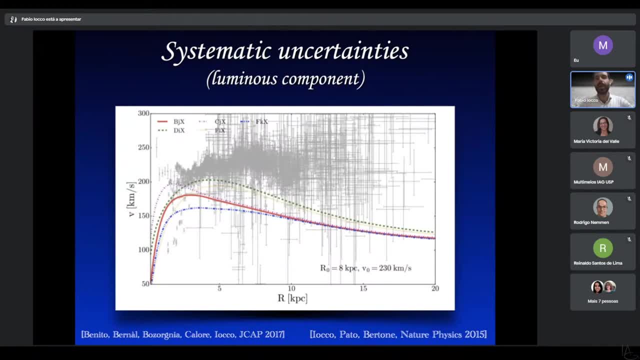 is that we have a lot, a big number of different possible morphologies of the stellar component. Now, all of these carry a statistical uncertainty which I'm not showing here just for completeness, but, as you can tell, they span a big 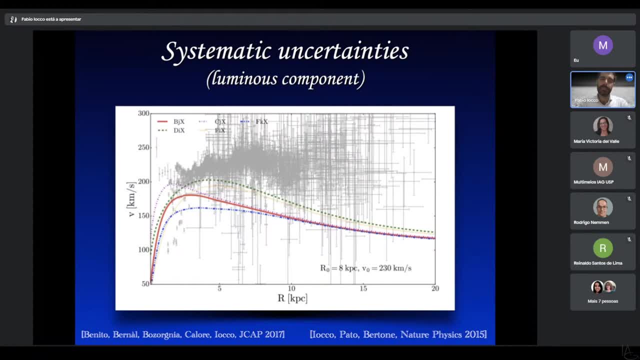 a big difference in this space, And now, this is one of the uncertainties that I was talking about. There is a statistical uncertainty That's well posed, But the biggest uncertainty is systematization, And that's because there are certain things that are systematic. 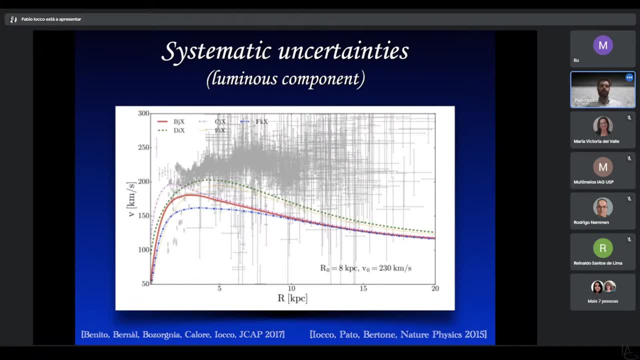 And that arises from the kind of traces you use for the bulge. So, what stars you decide to assign to the bulge, which stars you decide to assign to the disk, how you weigh them? Okay, Still, the result is unequivocal. 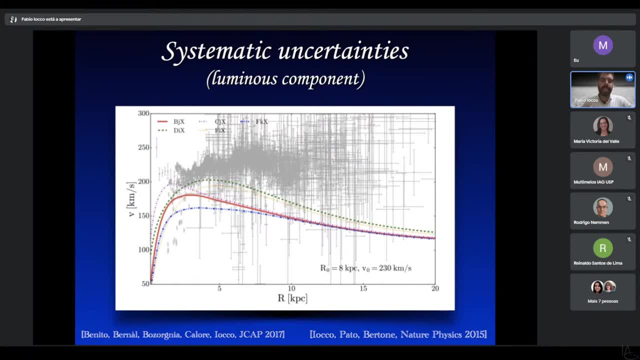 but the details of this result might change And if you're really interested in knowing exactly how much is the dark matter density around the Sun, that is a problem Because for each one of these possible morphologies, depending on how different they can be, 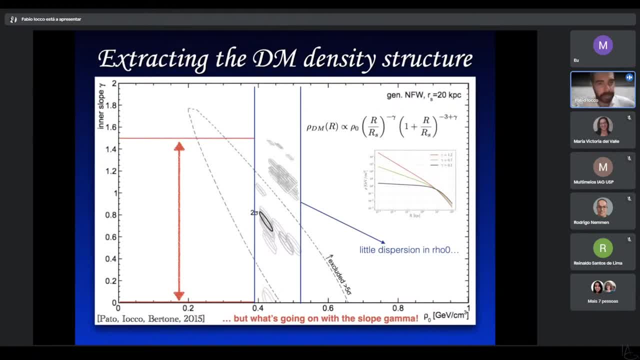 you get a different two sigma region. So there is a good point for that And the good point from this is that the spread in local dark matter density, even if you consider the ensemble and you're very brutal, you're not. you're not doing. 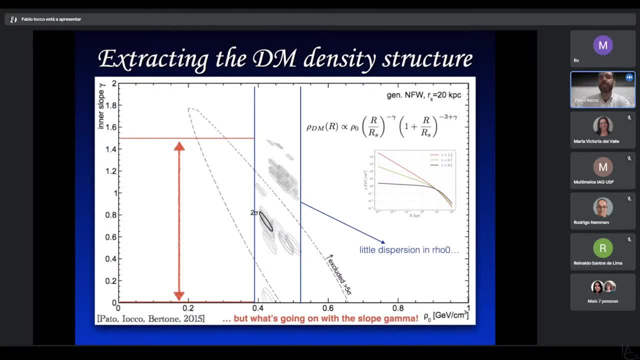 any statistical convolution. You're just saying: okay, the uncertainty is the minimum two sigma to the maximum two sigma of all of them. You can read the exact number in the paper. So it's very, it's a very well determined results. 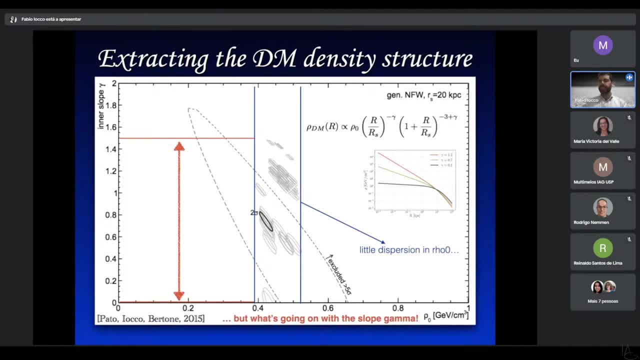 And it tells you: look, this is the dark matter density. There's no way out. There is an uncertainty, but it's not moving very much. However, if you're interested in the slope of the dark matter profile and to extrapolate, 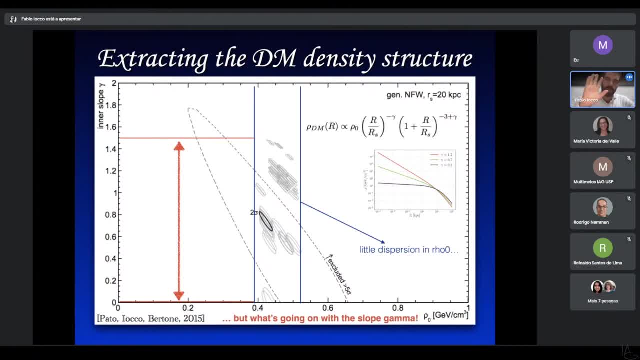 this slope towards the galactic center, which is not something it's well-posed to do, And I will come to that, But still, even if you want to do that- and I do not recommend to do that- then you're in trouble. 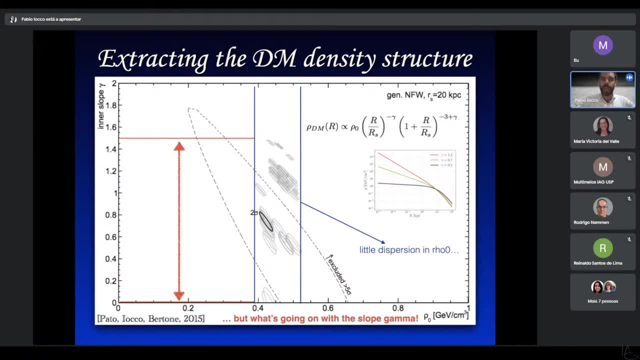 because, depending on the stellar morphology you have, this stellar morphology is allowed for a 0.1.. This stellar morphology is allowed for a 1.2.. So you get something very, very different, as you can tell here, That's. 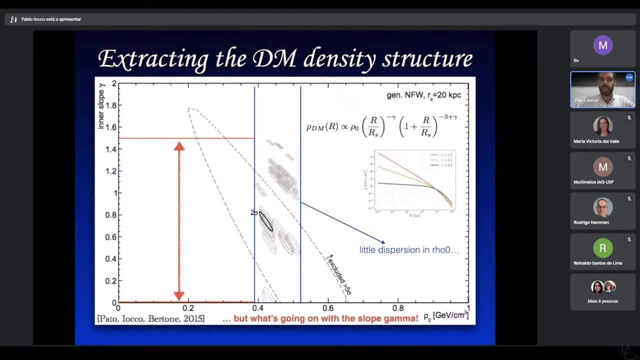 that's these ones. Yeah, And this is these ones. So it's a remarkable uncertainty. That doesn't very much affect the total dark matter content in the Milky Way, because when you integrate these over a small volume, it doesn't really change anything. 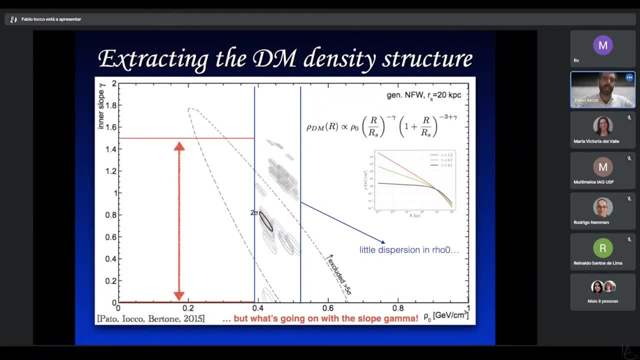 But if you're interested in how much dark matter is in galactic center, I recommend to use this method. but it gets even worse. You are pretty much cooked Okay. So so far I showed you one good thing And I'm very. 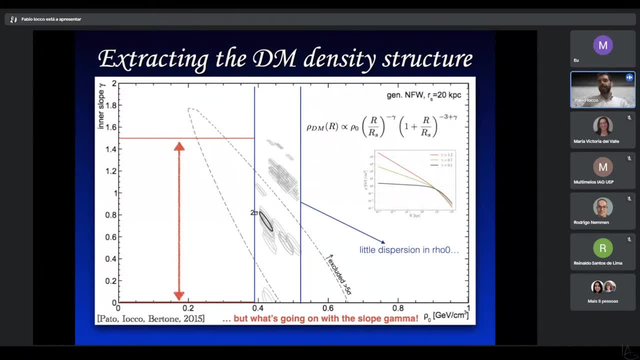 at this point, I'm very much concerned about the slope of the dark matter density gamma because, as I showed you, that's what we want to use to validate the lambda CDM extrapolation. How much time do I still have? Okay, 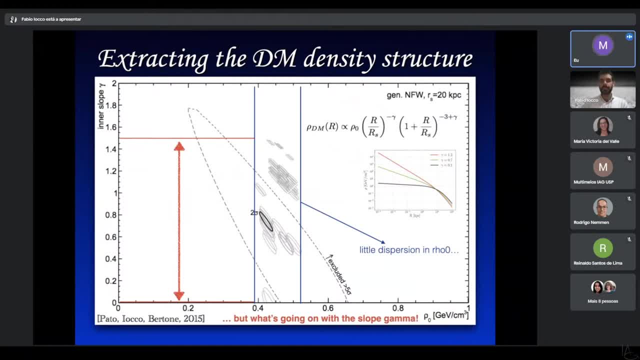 but you can understand what I'm saying. Okay, well then, it's fine. How much time do I still have? Oh, 15.. Yeah, but don't worry too much. Oh, I worry, but I worry for you. 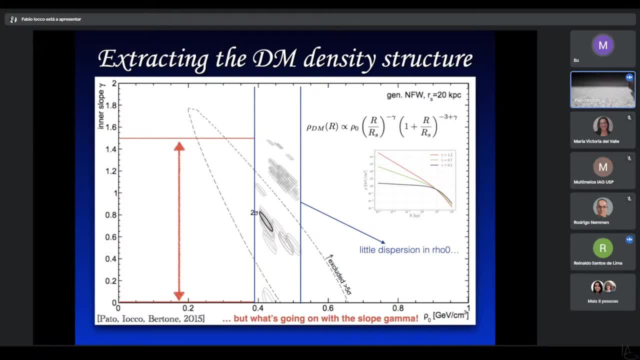 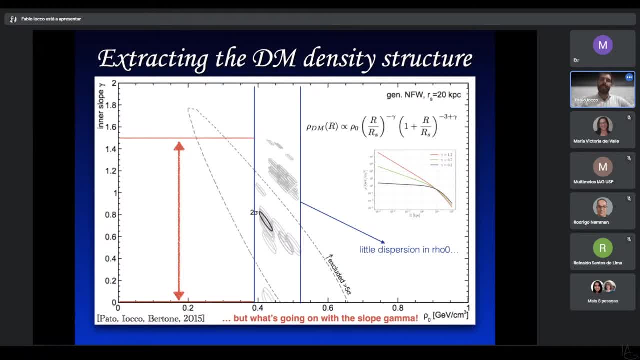 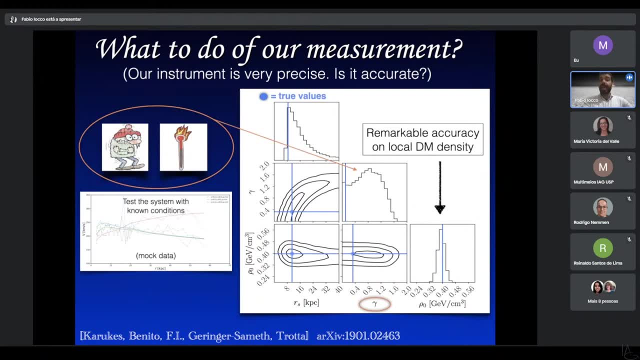 about the slope, because the slope it's what it's prediction, if you want, of the lambda CDM with gas. Yes, So I was very proud of this analogy that we show that our instrument is very precise, like at least for the. 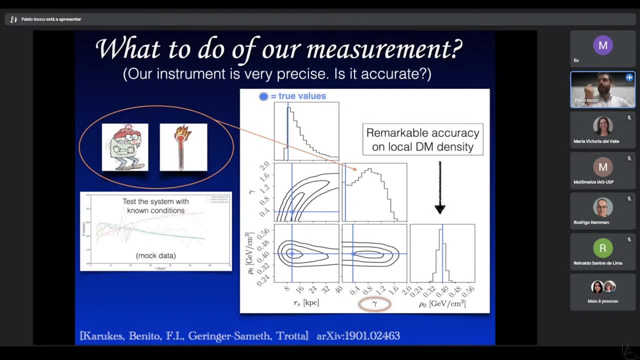 to look there. we didn't density, But it's very narrow. But is it accurate? I mean, a thermometer can be extremely precise and you evaluate which does mean inaccurate, okay, and in fact we find out if you look at the panel in the very, uh, in the very. 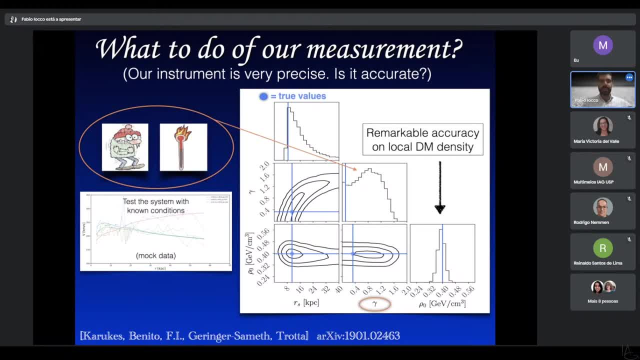 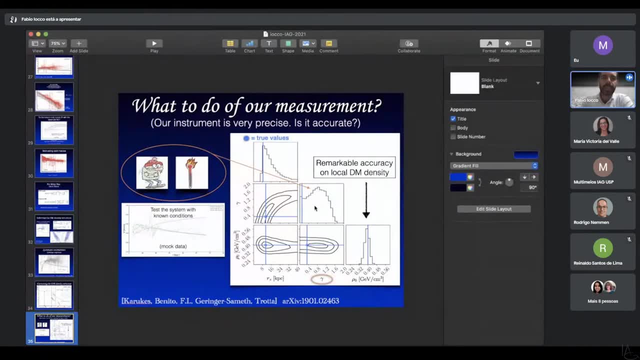 uh, in the central. so, okay, you cannot see my cursor. that's a damn. now you can see it here. if i do this, can you see it? okay? yes, let me do this. so in you seen this panel, the, the true value. we reconstructed the laser and we tested the accuracy of the system. so we knew what, when we did this, this was with. 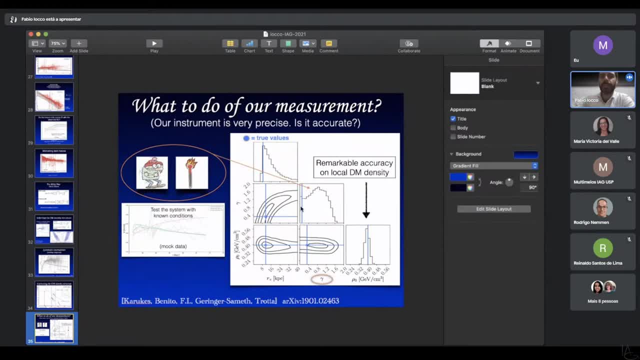 fake data. what we produced- and we knew that the system, if you give it a value of gamma, it will reconstruct another. it will do it with the big uncertainty and on the top of it for each realization- is far from the truth for some regions of the parameter space, whereas we are very accurate. 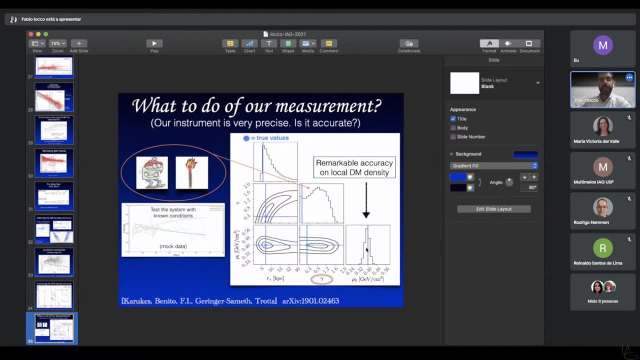 and very precise for, uh, the dark matter deaths. so we derived the conclusion that, really, if you want to use the dark matter, the rotation curve of the milky way, to determine the slope of the halo and use it, that's not a good idea. you're, it really depends on the morphology. you are not. 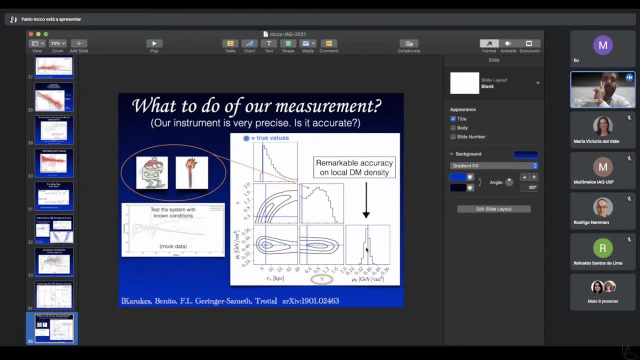 even accurate, and the mutant fails in the galactic center for reasons that i will explain. so i do not recommend to use it for gamma. okay, uh, let's hang on. well, this is the termination of the milky way mass. all the uncertainties i'm talking about do not really affect the determination of the. 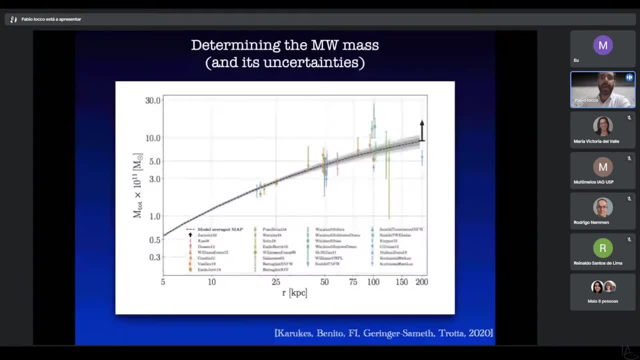 milky way mass because they get integrated out somehow. so that's a very solid conclusion. and you you are interested in the Milky Way mass for reasons that evade me. you can check the paper or ask me questions about it. That's not the main thing, Actually, the determination of the mass. 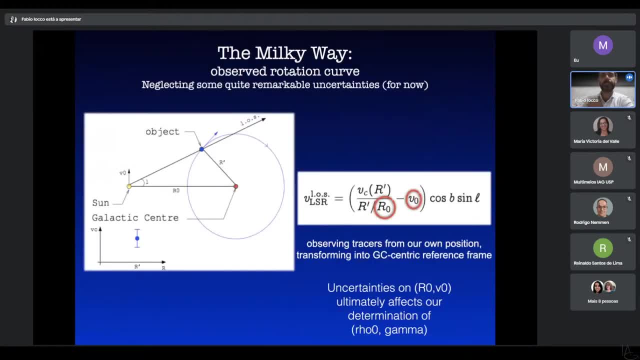 that we have is in good agreement with different other methods. so that's good. But let me come to the last point that I wanted to make. I showed you what the uncertainty is. So the statistical uncertainties on the observables are fine. We have them under control and they do not play a major role. What is really affecting? 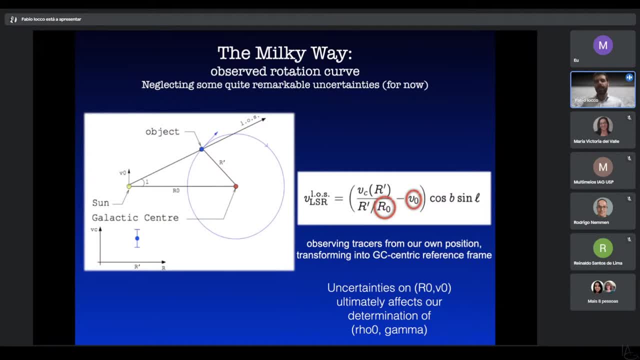 the determination of gamma and, somehow, of the local density is the morphology, the stellar morphology, and that's a systematic. There is one thing I didn't tell you: We are sitting around the Sun and we are observing something that is rotating around the galactic center. 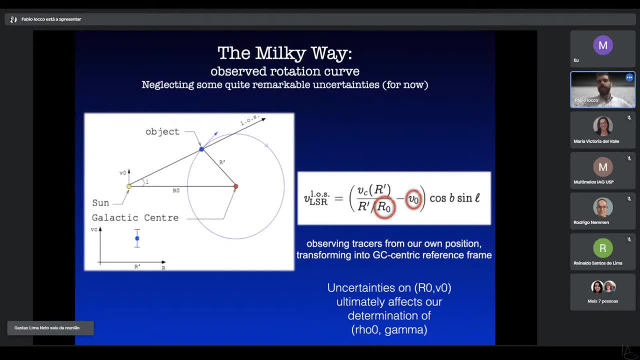 Now we learn in the first year to change reference frame. but to change reference frame you need to know of two systems that are Galileanly shifted, so they do not have the same origins and they have a relative, but they have the same origin and they have a relative. 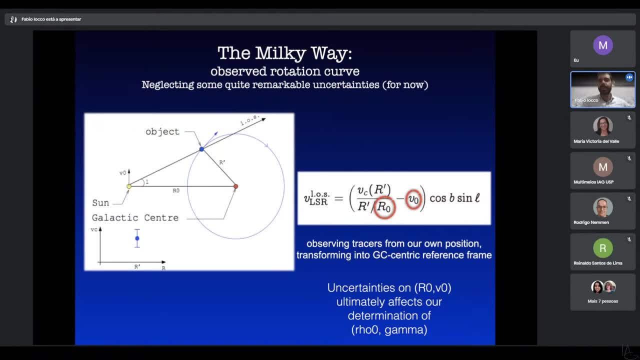 velocity. What do you need to know is both their distance and their relative velocity. and we do measure our distance from the galactic center and our velocity from the galactic center, but we do it with measurements, with determinations, and those measurements 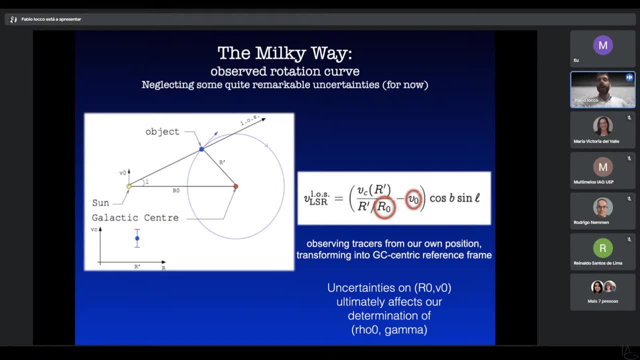 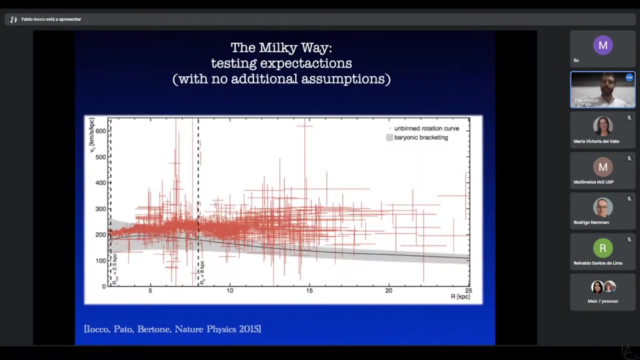 are affected by uncertainties too. So, on the top of the statistical uncertainty, what is the absorption line or the spectral line that you're observing? you have to transform it in the reference frame and you are affected by other uncertainties, So these uncertainties actually propagate into the rotation curve. how it looks. 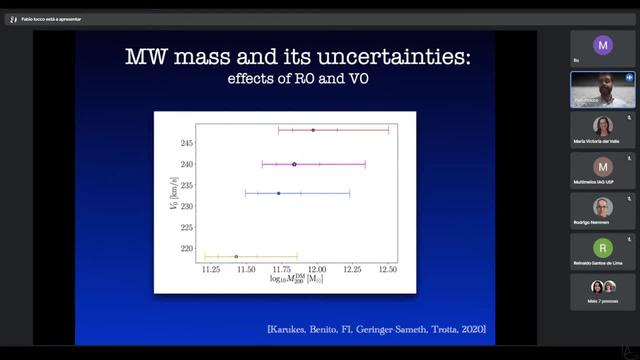 and the determinations that we have. This sort of affects the determination of the Milky Way mass, If you use different determinations of what we call the galactic parameters, so our distance and velocity with respect to the galactic center, and of course it goes up. 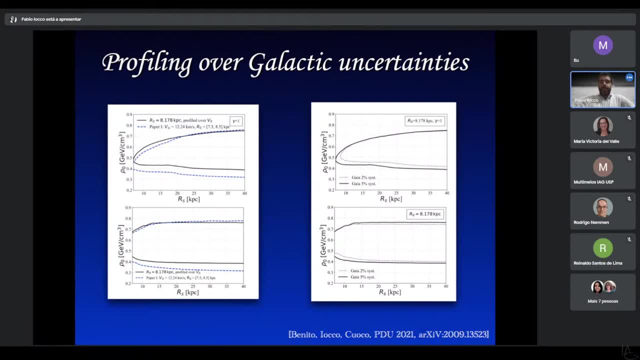 But the interesting thing is that once we start pulling in and much, much, much, much, much, much marginalizing over the uncertainties that we have on the galactic parameters, the interesting thing is that the results are consistent. The galactic parameters will not affect very much the determination of the local 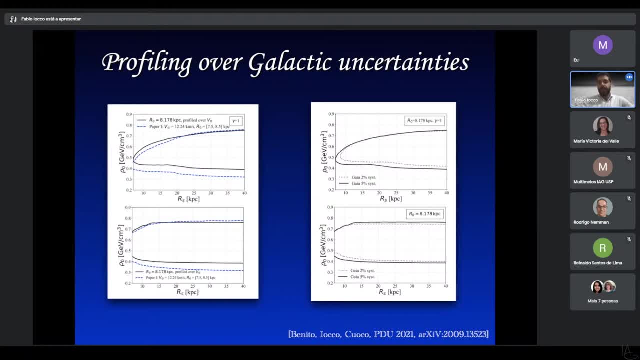 matter density, not dramatically, but they do affect gamma. Now take this point, bear with me, because now the part of interest for the astrophysicist is somewhat over. There will be a small break and then I'll come back to that, If you're. 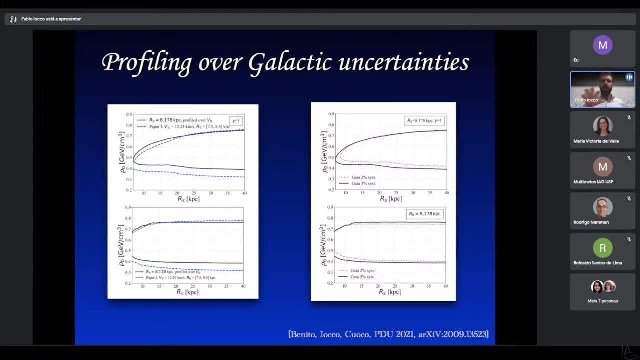 interested in the galactic center. maybe you can ask me later on, But now I gave you a list of uncertainties: Statisticals- they're under control, Systematic, because of the morphology they are a pain- And galactic uncertainties. 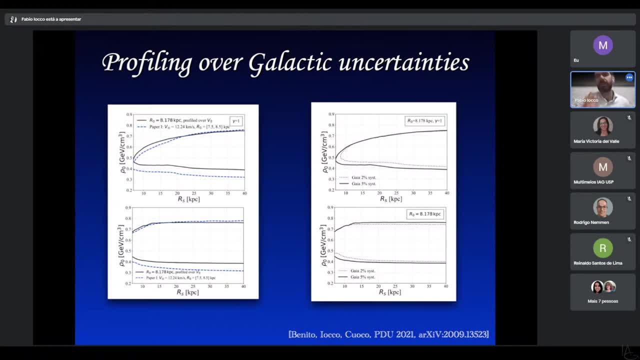 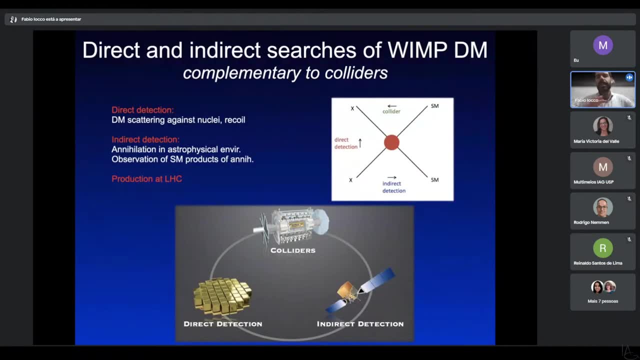 they do exist. They should be taken into account. let's say They're not dramatic, but we should take them into account. Now let's go for a moment to WIMP, Black Matter Searches. It's something that is fading for a host of reasons. It's not dead and this work was done. 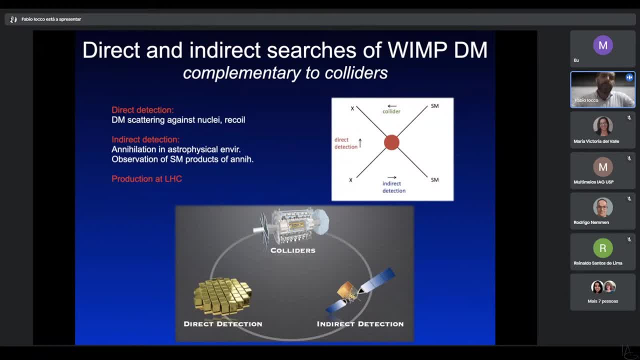 when it was more alive than it is now. But searching for the nature of dark matter, that so far has not gone into the game. We do not need any nature of the dark matter, We just need it to be gravitationally interacting When people 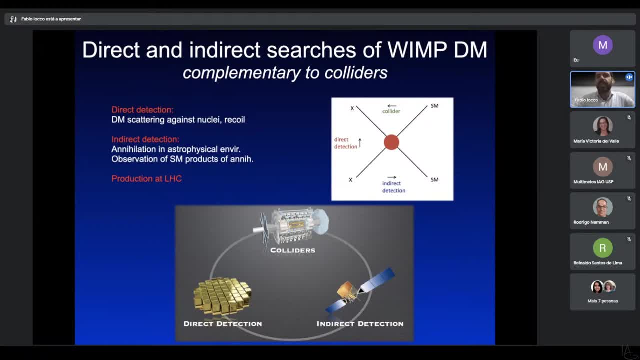 looked and still look at WIMP dark matter. they're using this sort of scheme. Look, I can observe these particles annihilating into standard model particles and that's the right arrow of the diagram. so top right here, Ti chi particle, particle annihilating the standard. 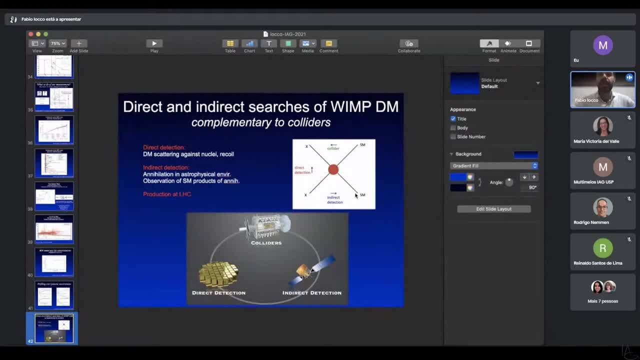 model That's called indirect detection. So you look at exotic stuff, high energy, astrophysics, Then you might produce the collider. That's the other direction. So you might observe something getting out of missing energy in your collider. or you have a scatter, So you have the particle. 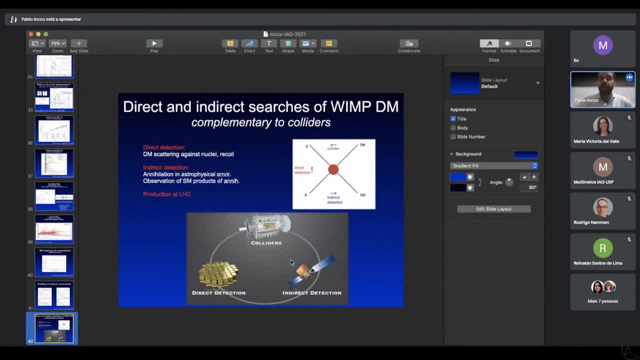 scattering with the standard model. That's what you want to look, with direct detection underneath, And that is the up direction of this schematic Feynman diagram. is what you look at- direct detection and what is sensitive. And that's what you want to look, with direct detection underneath. 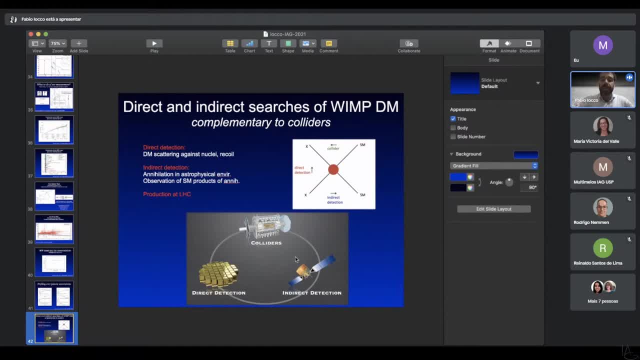 Now, if you put all these things together and you try to infer what is the actual interaction here in the center, the red dot, which is the diagram that we're interested in, and you do it observationally, which is very well posed and we believe it's very well posed, 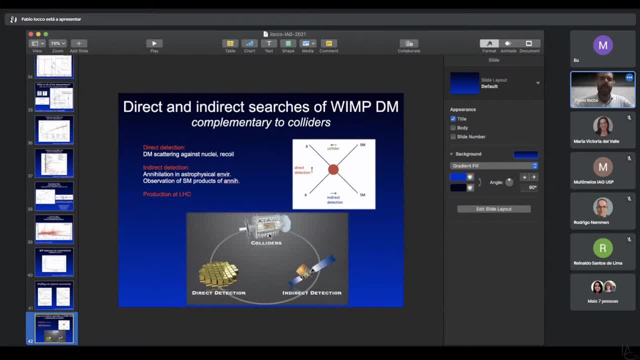 you will use real data from the colliders and you will assign uncertainties to them. You will use real data from direct detection. then you will have experimental uncertainties due to the number of counts, to the type of material. You do observe real counts for. 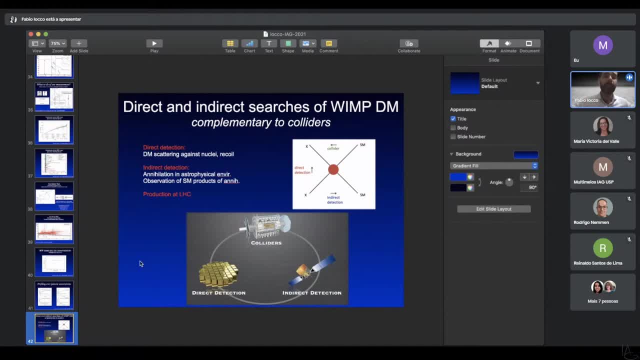 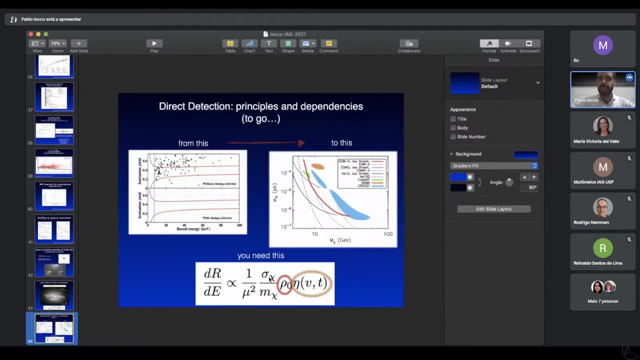 indirect detection. and then magically, when people extrapolate these things back to the quantities of interest, which are sigma v and n, for instance, or the cross-section sigma key, nobody really took into account, back when we started this work, the real uncertainties. 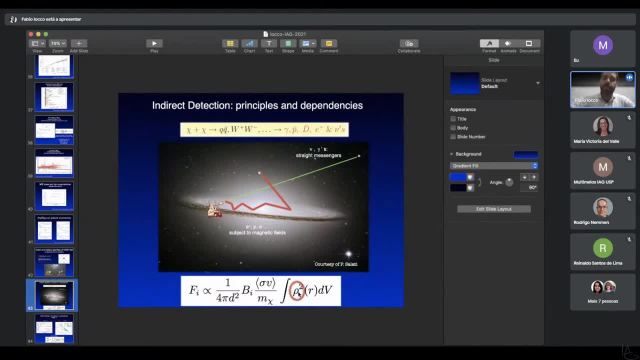 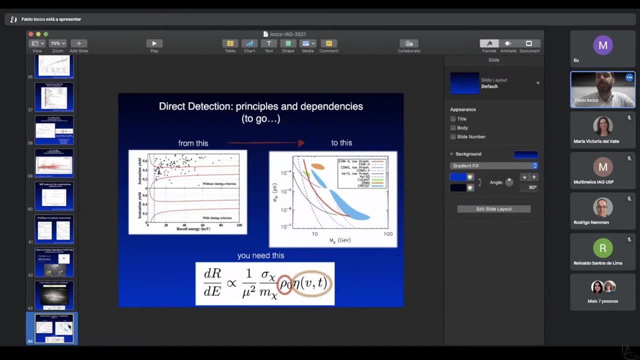 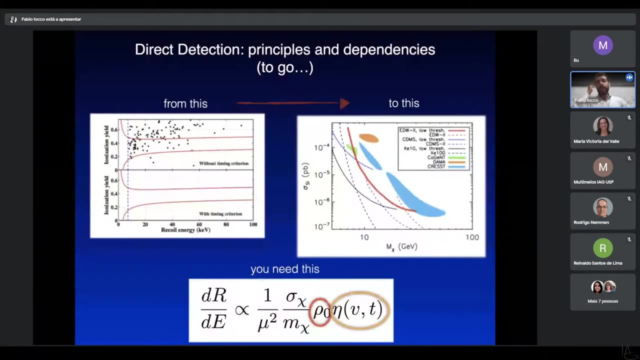 the observational uncertainties on the dark matter density that you need to extrapolate the signal. You have to make a choice on what it is, and you have data. Why picking a benchmark that comes from simulations And that's the same for direct detection, okay. So what we did at this point was say: 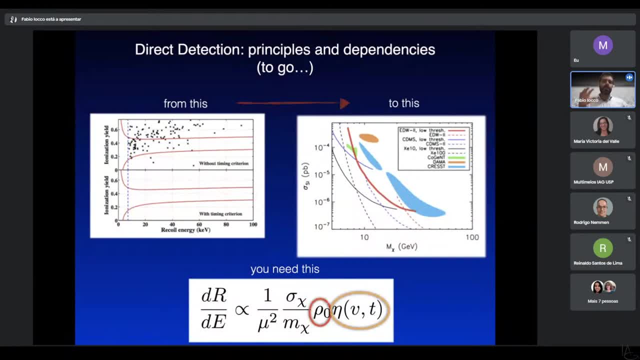 okay, we have a bunch of uncertainties. Let's say that I want to use all the data that I have- direct detection, collider, indirect detection- to reconstruct the parameter space of a specific model. So I will do a model-dependent search of a specific type of dark matter. 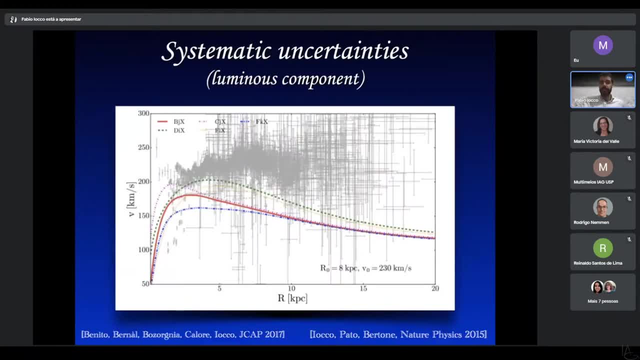 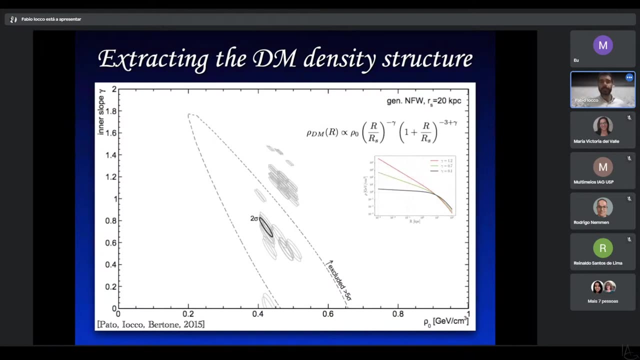 and then I want to fold in the observational uncertainties that comes from a surface. So again we're propagating from the uncertainties that come from the rotation curve down to the parameter space- okay- of the particle, of the extension of the standard model that I'm considering. So this is again my trouble. It is different slopes. 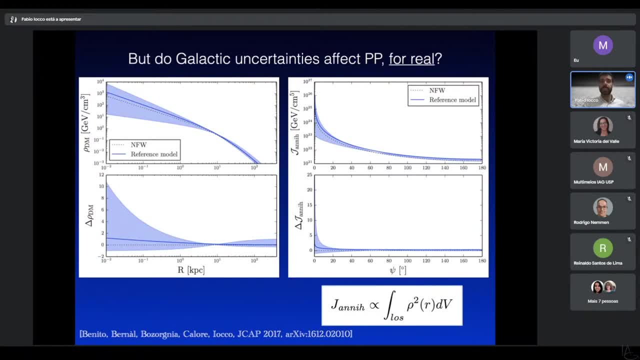 different local dark matter densities depending on the morphology There be. do they really affect uncertainties on particle physics? And the truth is that, look, if you're interested in the dark matter density, that's the spread that you get around the solar. 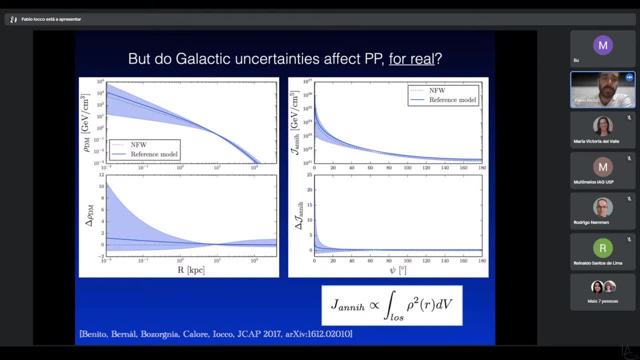 rays. It's a factor of five And, yeah, something of the kind, If you're interested in dark matter annihilation in the galactic center, that's actually. it boosts of 10 to the 23 to 10 to the 25,, two or three orders. So, yes, indeed, the astrophysical uncertainties might affect particle. 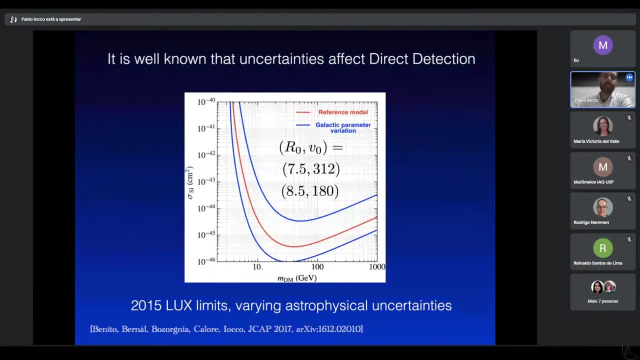 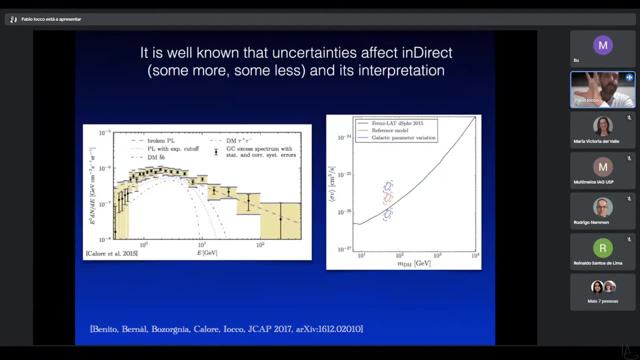 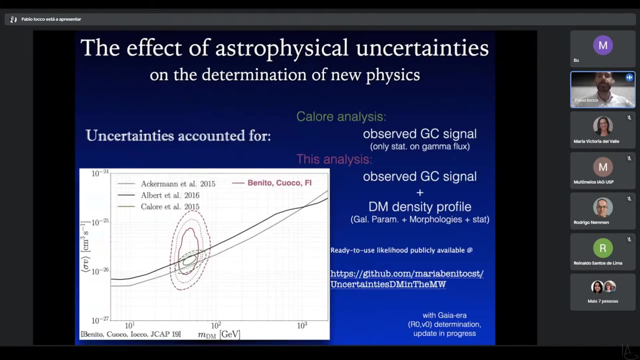 physics for real, And so we started a specific case in which we use the data of the LAC's limits. we use the galactic center access as a probe just to say what happens if we interpret that, and then we apply uncertainties to it. so the point i'm trying to make is, if you want to study a 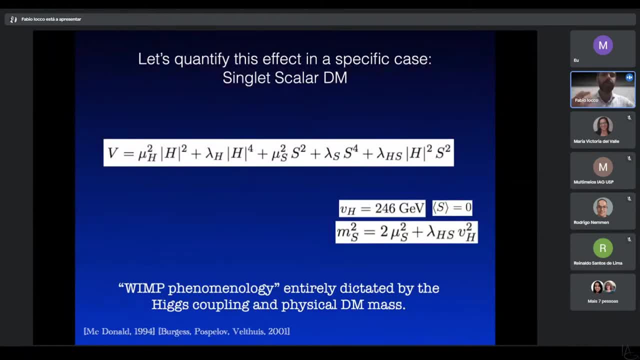 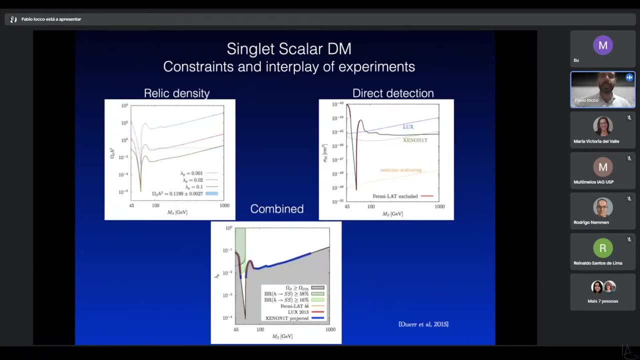 specific model and we perform this exercise just to show that it's relevant. we do not necessarily believe this is the right model. we're just giving an example. when you apply data to interpret the dark matter as this lagrangian and you want to put constraints in the parameter space of this, 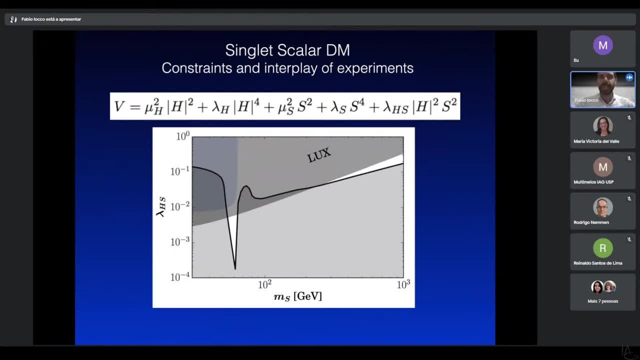 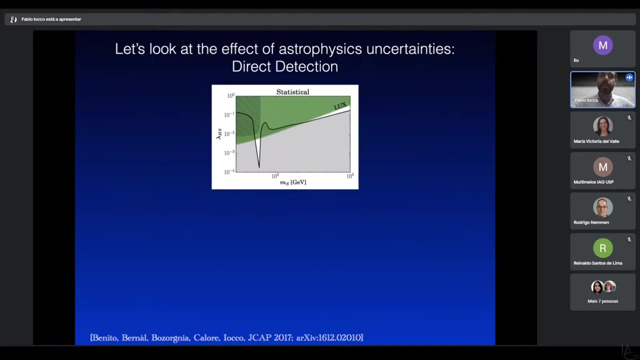 lagrangian, you will find that these are the constraints that come from Lux observations, flank observations, uh and galactic center annihilation at some point. these are the constraints in the parameter space of this lagrangian. and look what happens. if you only take into account the statistical uncertainties that I showed you, can you see, can you tell that? 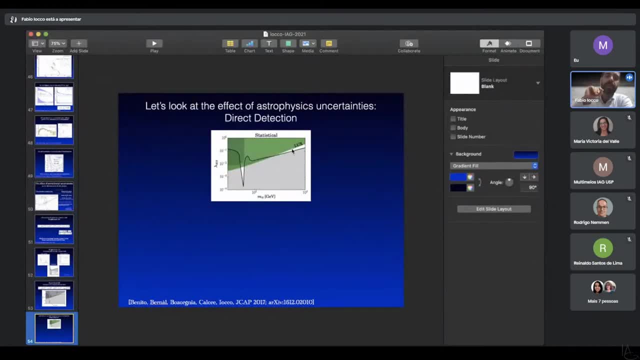 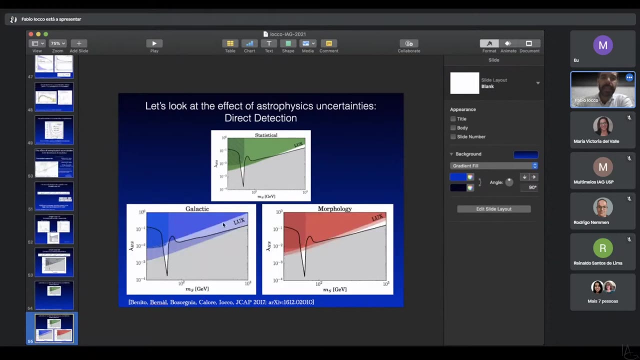 I am taking one particular realization of our knot and I'm saying: look, there's statistical uncertainties, there's two shades of green, but I bet you that you don't see these two shades of green. what happens next is that this is how this plot transforms that, if I apply galactic parameter. 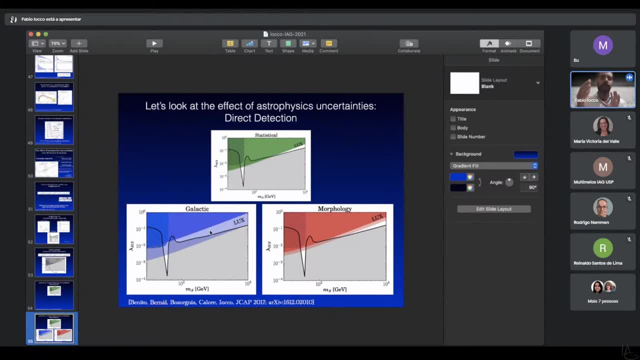 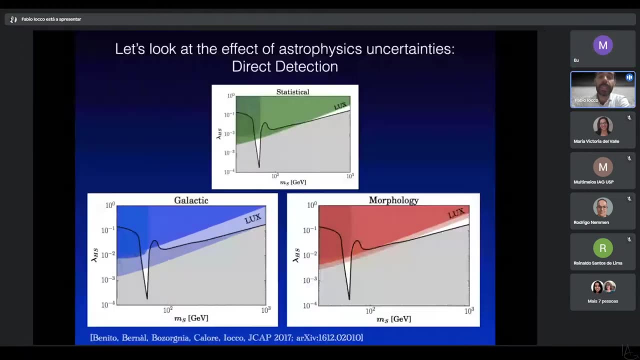 uncertainties. so the fact that I do not know very well distance from the galactic center and the relative velocity, and therefore I apply the systematic that I have and I have this sort of you can. you can see the two shades of green. okay, but it's very small. I mean usually when I use a 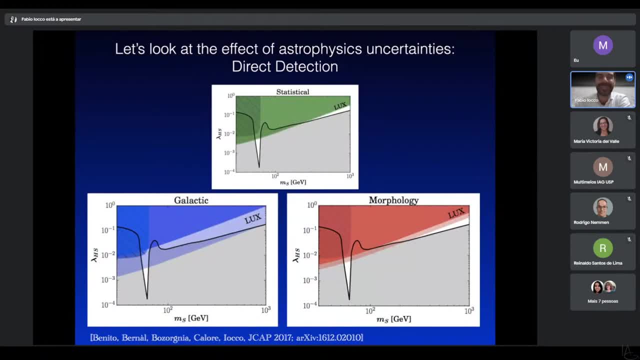 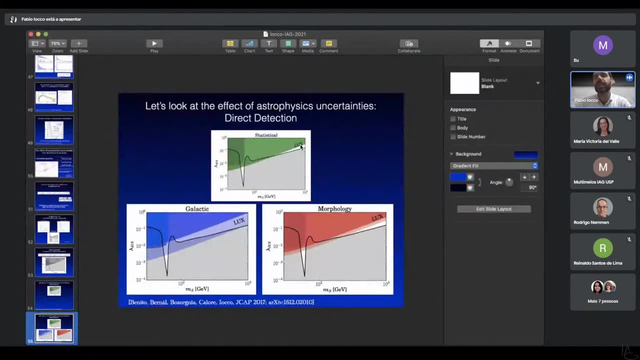 normal projector, you cannot see it. what I'm, what I'm trying to say, that's. that's a fair point. but what I'm trying to say is that it's very limited the different shade of green. so the impact of the statistical uncertainty on this limit is admittedly small, and that's fine. 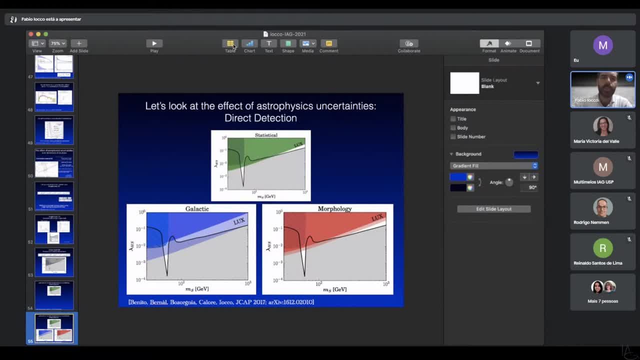 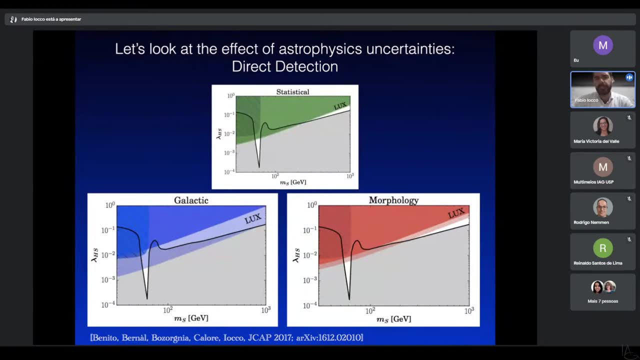 now, if you want to be extremely fine-tuned and you're a particle physicist and you have a model that really falls into this green line of the parameter space, that might make a difference for you. but we agree, it's very small. in contrast, if you want to take into account the uncertainties, 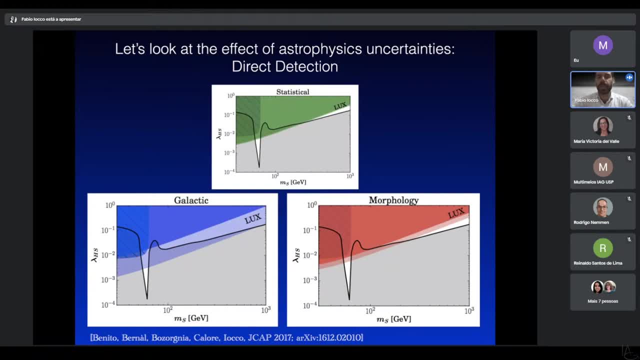 on R of naught and B naught, you have a big change- see the bottom left- and if you're taking into account the, the uncertainties on the morphology, you have a still have a sizable change, way more than the statistical uncertainty. So the exercise we played with this paper, that was done also in collaboration with uh, with people. 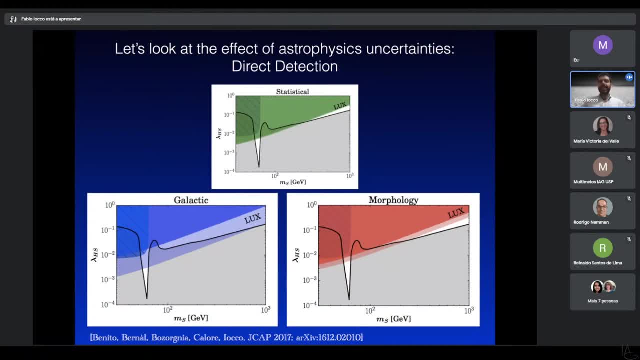 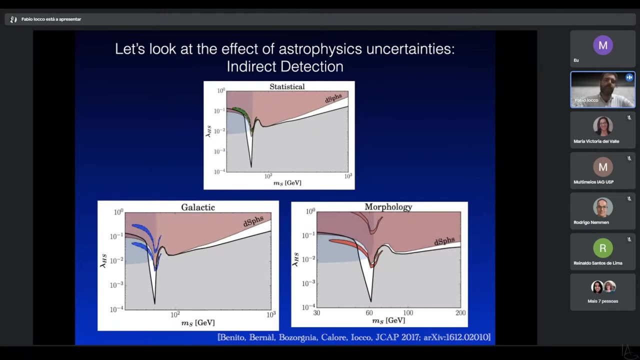 when I was there in Sao Paulo, was to show that actually, the astrophysical uncertainties had an impact on the determination of particle physics in the very parameter space, that particle pieces that I used to look at. okay, now, this is where the interpretation of the galactic center accessing 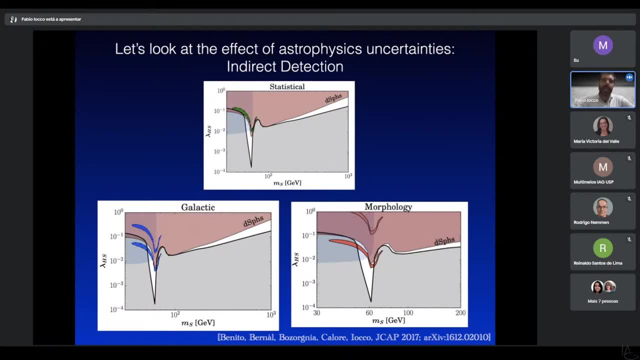 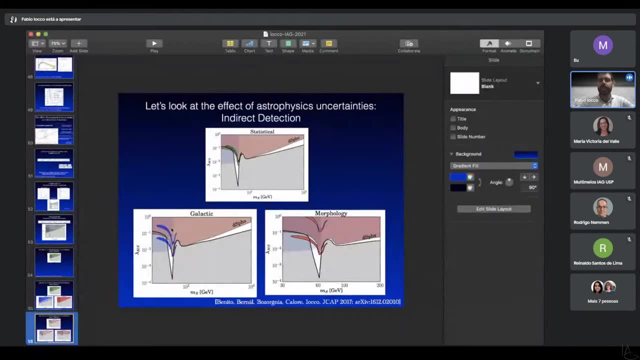 gamma rays is supposed to be, if you interpret it as dark matter, annihilating. and this is how it moves in the plane. if in the bottom left you can see it here how it moves in the plane, if you, if you change the galactic parameters, and here is, if you change the morphology, so this region moves from. 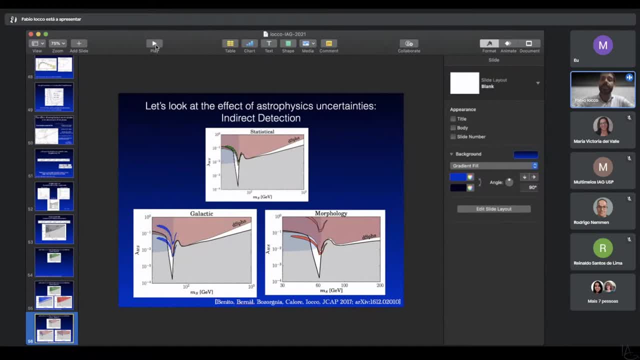 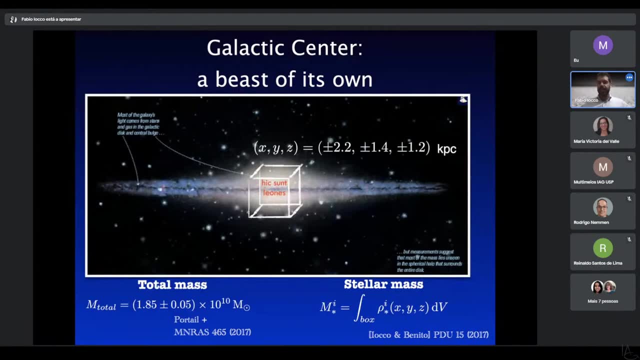 being entirely forbidden to being totally allowed, and so it is a big change. you have to take care of astrophysical uncertainties, so that was a simple message. we can quantify it. if you're working on that, I'm very willing to give more details, but the the 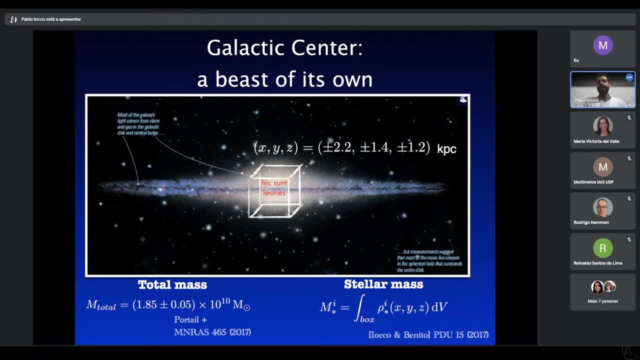 the point the, the Benchmark and the take-home point is astrophysical uncertainties on the rotation curve of different nature to impact the determination of particle physics, okay, of physics beyond the standard model. now, if I have five more minutes, um, I will give you a very disappointing and very depressing message. otherwise, I will just go to my conclusions and will spare. 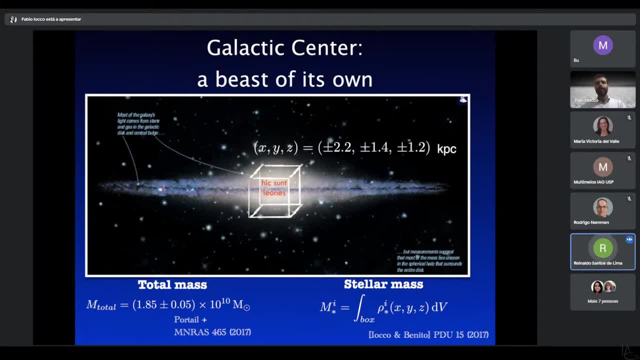 you depression and mine, because it's late and you have, so you want me to get depressed and depress, okay, yes, yes, thank you. now I'm curious. I told you I will go home and actually I will stay home, um, so I told you that it's a very bad idea to extrapolate the uh dark matter profile toward. 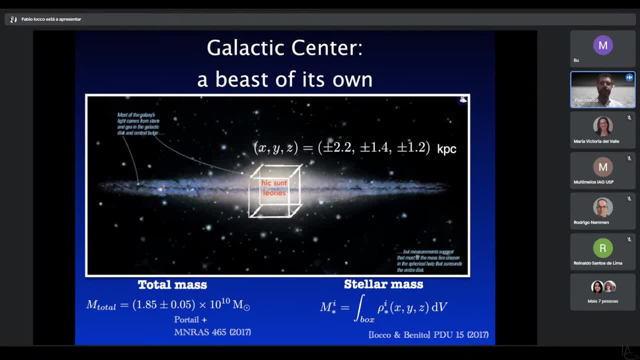 the center, the galactic center, and that's that has a very good basis. the thing is, first of all, even in modern simulation you start seeing that there might be a break in the dark matter profile break and the region is that the galactic center region is domination, is gravitationally dominated. 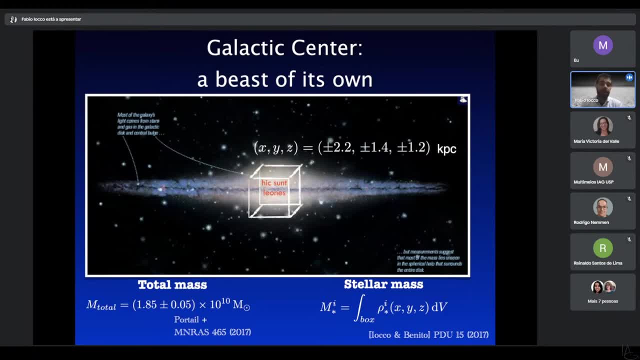 by the variants, and that's well posed, because they're called dissipational and they fall into the gradation challenge. so extrapolating a straight power law might not make sense. but the other point, but but you might argue: okay, I want to believe it's a straight power, okay, fair. 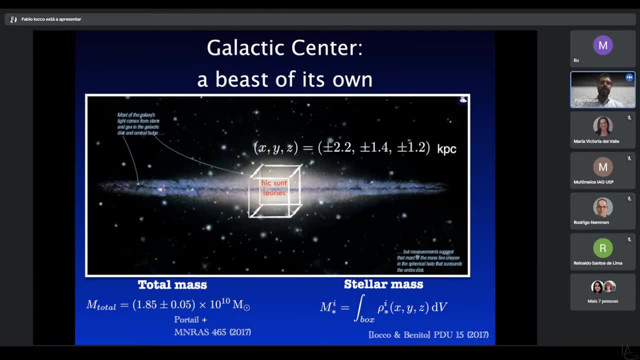 enough. the point is is that we don't know if the rotation committed can extend toward the innermost regions. now, for innermost regions I mean something below 2.5 kilobars, so basically the bulge region, and the reason is that, in order to apply the rotation curve, you have to assume that there. 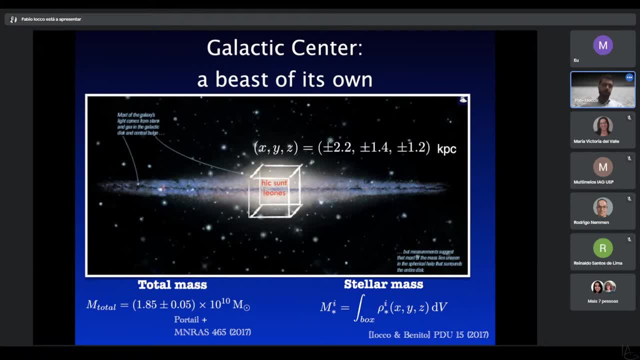 is a rotational the, the, the disc is rotational supported, which doesn't apply to the bulge. and also you have to, uh, to have to be convinced that the orbits of the objects that you're observing are circular. and there is quite um an evidence that they're not really circular, if you go even. 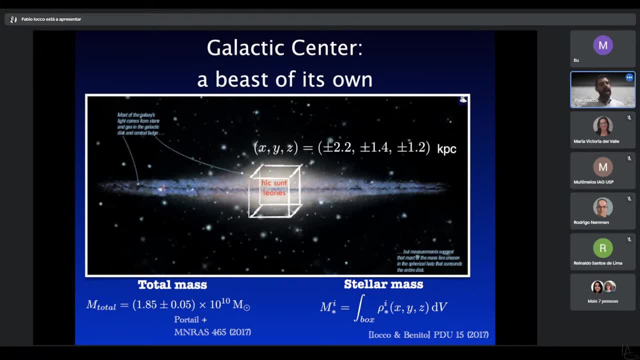 the tracer object the word of God. so we discard them usually, and on the top of it they might not be, even if you have some circular objects. they might not be coupled to the gravitational potential. they might have some sort of initial angular momentum or motion that they didn't manage to get rid of. and so you're just. 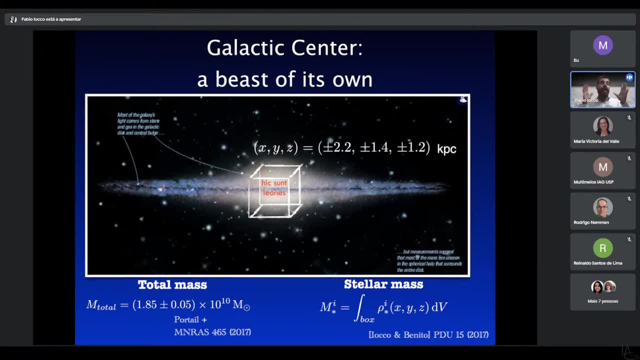 tracing something else, okay, so I recommend not to extrapolate any profile with a gamma beyond so closer to the galactic center than three kiloparasyte is emitted to study the potential in the bulge. and that's just to apply pure jeans equations. so 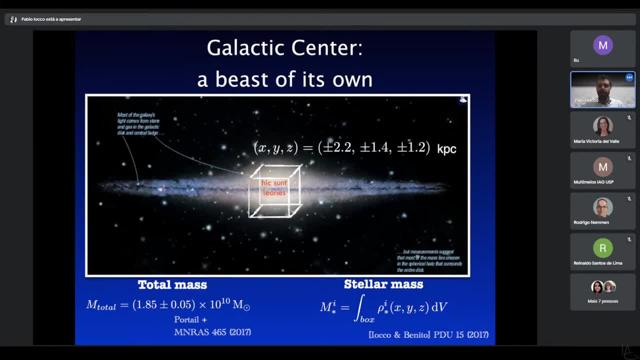 you have a bunch of tracers that you can take stars in the, in the bulge region, which is more or less a box. you can see the size here, uh, and say, okay, I can tell the total mass because I I can observe those stars, I can invert the dreams equations and I have the total mass. fair enough. 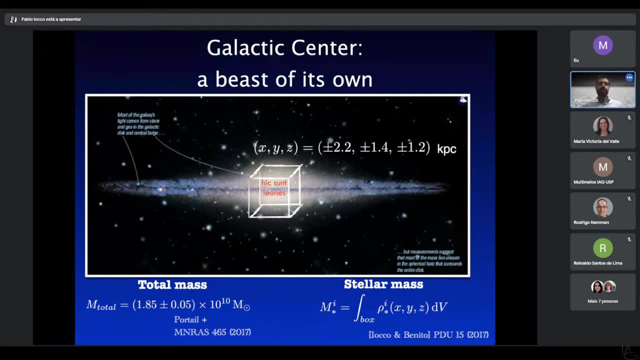 I can observe stars and I can impair the stellar mass and so just subtract the two. it's very simple in principle, in theory. now, the difference in theory and practice is that, as everybody knows, is no difference in theory and in practice there is a big difference between theory and practice. so 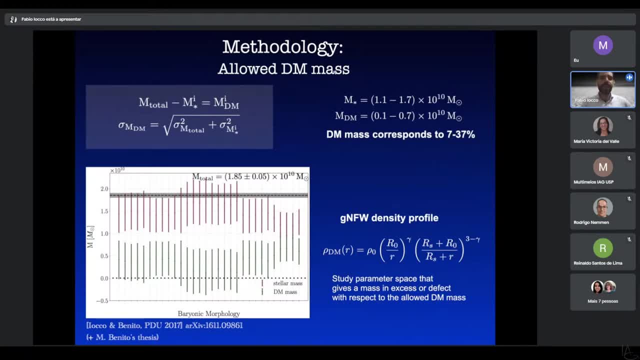 when you do that, you get very nice numbers and you get very high uncertainties that make the dark matter mass inferred through this method comparable with zero in the galactic center, and that's very well posed. I mean that's observational, so it's a result period, it's empirical. on the other hand, you do expect in 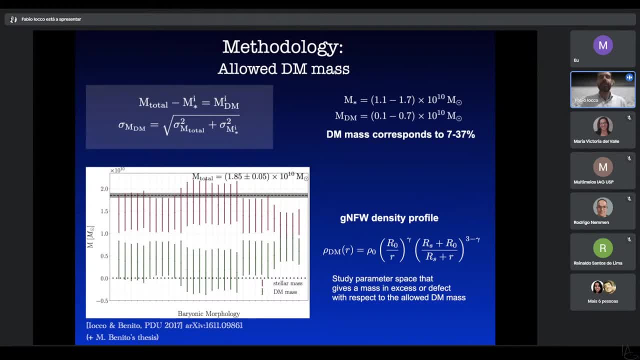 a lambda CDM galaxy information. you do expect there to be very little dark matter in the galactic center because the body is concentrated there. the dark matter is dissipation less, so it stays in the outskirts of the hill. so on the one hand, okay, I'm happy, but it's a not, not no-brainer, but it's a very 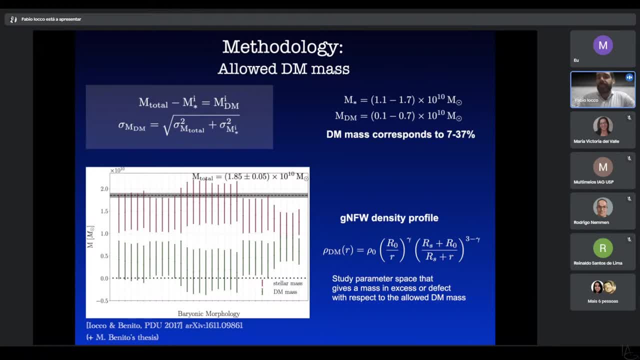 simple answer doesn't even match information. now the thing is okay, it's not zero, it's compatible with zero, but it's non-zero. I get a number and then I won't interpret this number with an additional dark matter profile that I set free from the external one. I just imposed some continuity conditions. 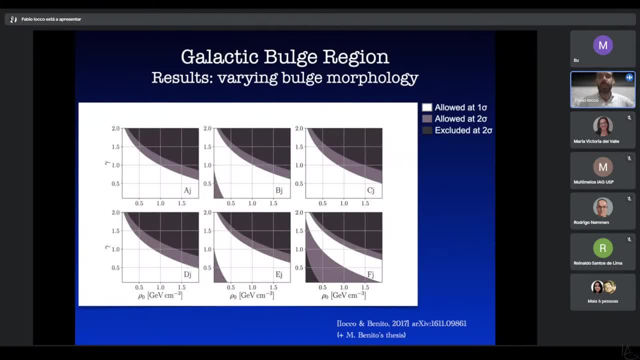 now the parameter space allowed is the white one. I did request this color coding and I realized that I was stupid. my student had warned me against doing this, So it's counterintuitive. I don't know why I did it. I apologize with everybody. Maria told me. 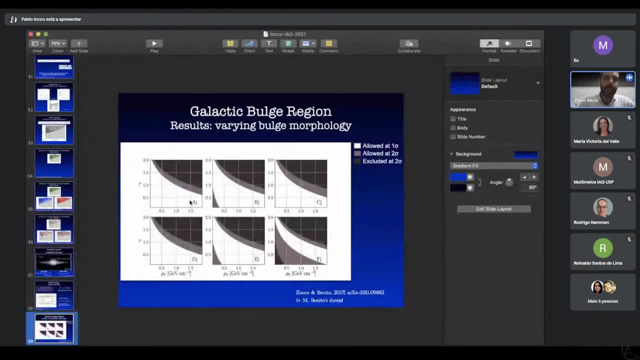 And so the white region here is the allowed space by that mass, the mass that you infer. okay, So, depending on the morphology, on the combination of disk and bulge, you have a huge parameter space. So you have a good answer. 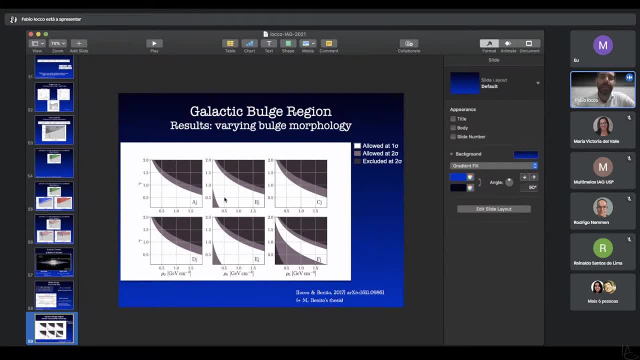 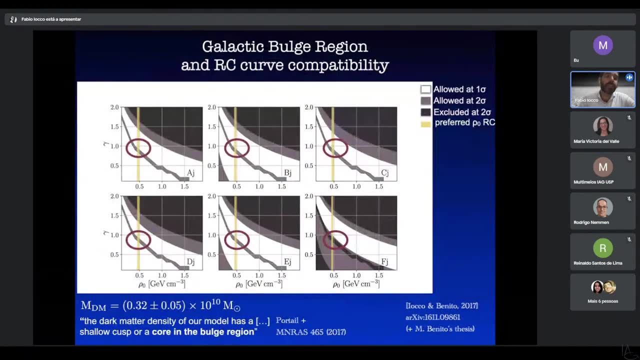 Like. you can always arrange for a dark matter profile in the gothic center. It's just that you don't have enough information. Now, the good thing enough is that if you on the top of it, you overlap what you expect, like putting a constraint of continuity. 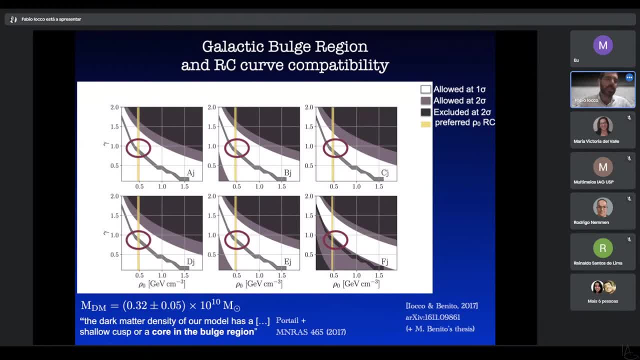 with the external one, the one in the external regions. you end up in that region and that's fine, but you're far from being able to claim that it's a flat profile, as some people did. okay. So this was Maria's point: to criticize a paper. 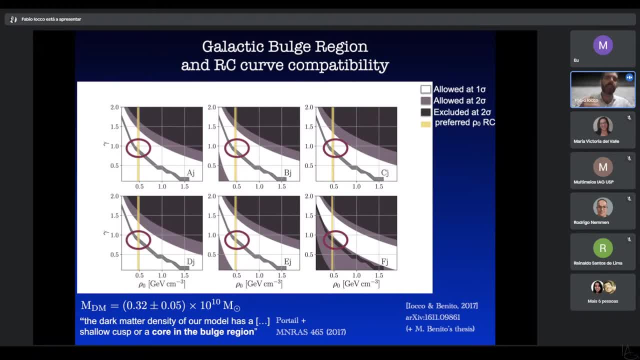 that appeared saying that the dark matter density profile in the gothic center has to be flat. My point- I don't know if this is Maria's point- Maria's point was that's wrong. You cannot claim that there is an evidence for a gamma being zero. 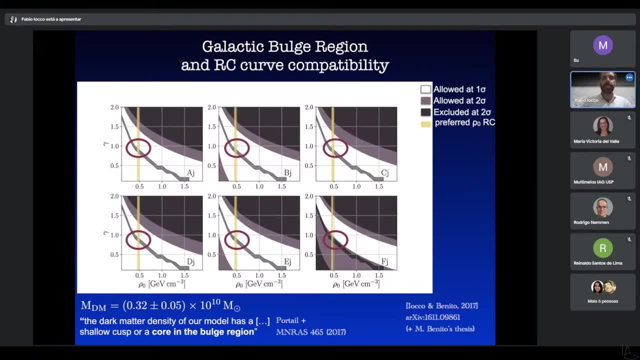 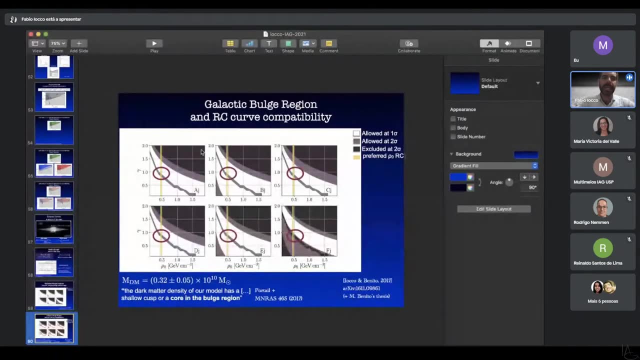 That's fair. that's a fair statement. My point is we don't have enough information to say basically anything about the galactic center. I would not defend any statement. I would defend the statement here If someone tells me it has to be, you know. 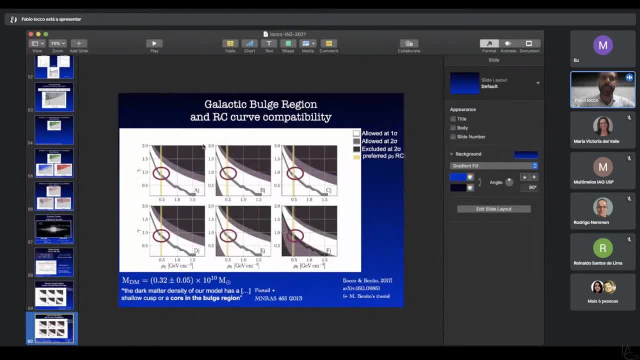 there has to be two point: the slope has to be 2.0.. I'm saying no, unless you have very little local dark matter density, it cannot be That statement I would defend. But if someone asks me, what is the index gamma? 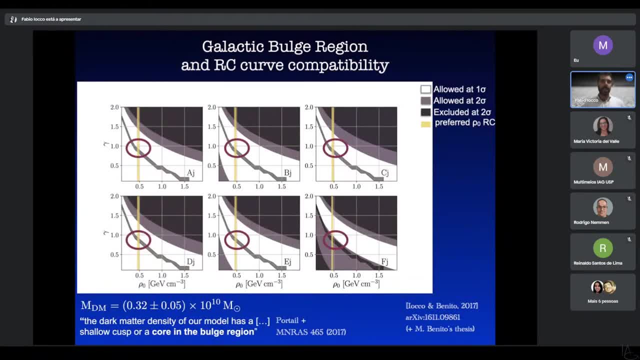 in the galactic center? I would tell you, I don't know It's. there's a big uncertainty. If I extrapolate from the outer regions, which I am not willing to do, I am committing something that I I'm committing to something I don't want to do. 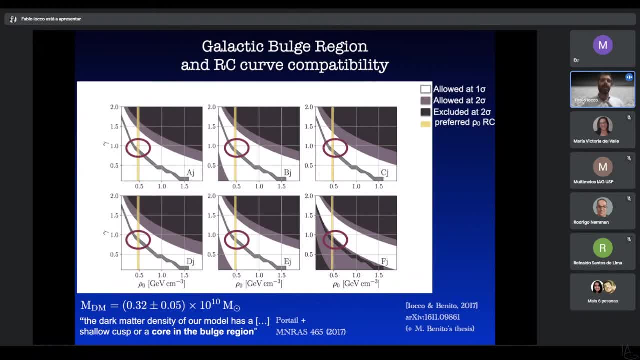 And on the top of it, I know that even the index gamma in the outer regions might be affected by misreconstruction because the system is not accurate. So that's a very negative message. That's why I tend to skip it. But I think people need to know. open your eyes. 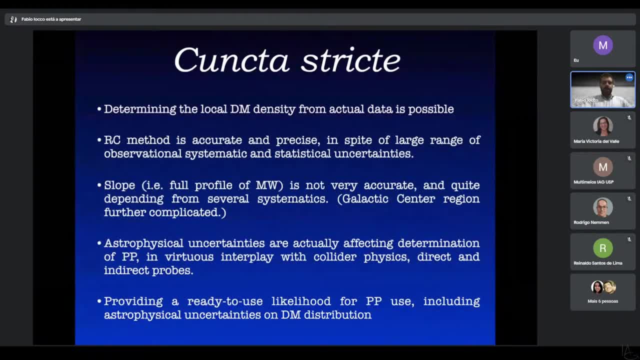 So I will leave you with my conclusions that I can summarize, probably briefly, saying that determining the local dark matter density from actual data is possible, is very well posed, And we have a relatively sound determination from the local dark matter density. We also have an evidence of the fact. 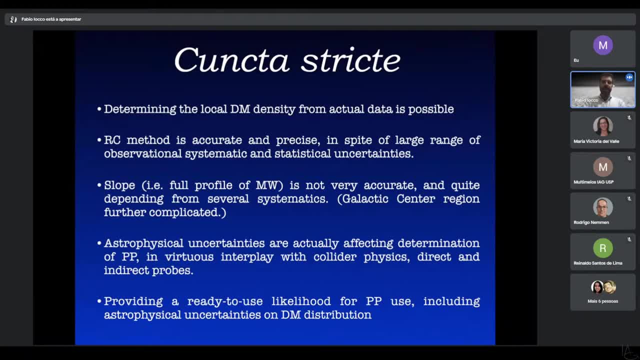 that the rotation curve of the Milky Way cannot be supported by stars alone. There's absolutely no way. okay, The determination of the slope is a problem, And let me not elaborate more on this, But the other thing is that our statistical uncertainties are actually affecting the determination. 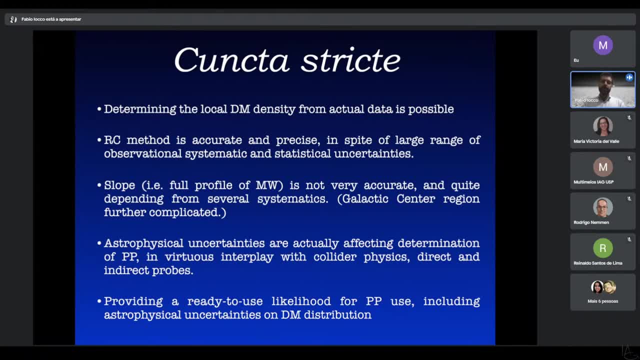 of particle physics. So, if you want to use that, if you want to determine particle physics, if you really care about the determination data grid and the determination of particle physics parameter as data driven from the astrophysical part as it is from the particle physics point of view, 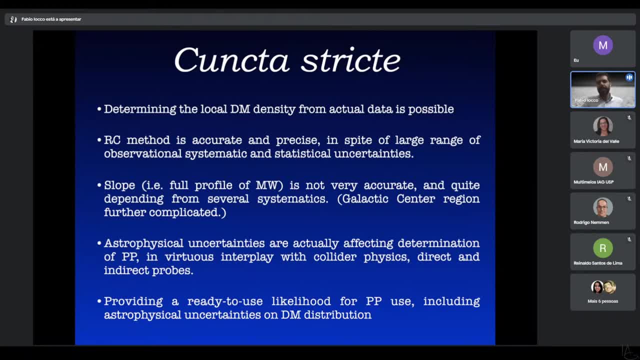 then you have to fold in the uncertainties from astrophysics And, of course, Maria and I provided you with a tool that you can use at your leisure. It's online. there is a GitHub. I don't know if I gave the link. 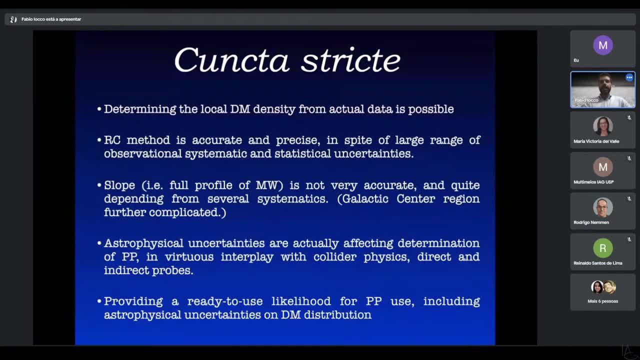 You can download it and you can contact Maria for further instructions. As of me, I thank you for your attention And please ask me questions. I wanted to get a drink for the questions, but I think I don't have time. 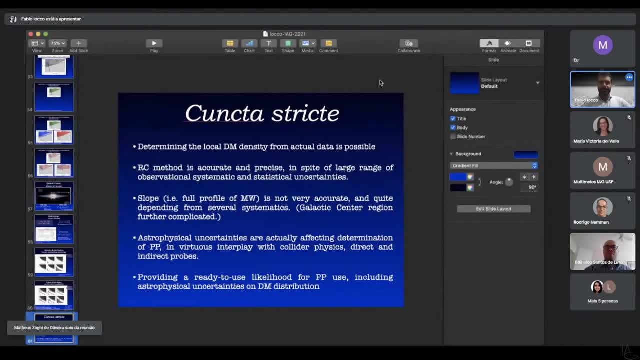 So you just ask me questions. Thank you, Fabio, for the very clear presentation. I think it was very didactic. I myself I have a question. I can start here. In fact, I would like to confirm something that I understood looking in the beginning. 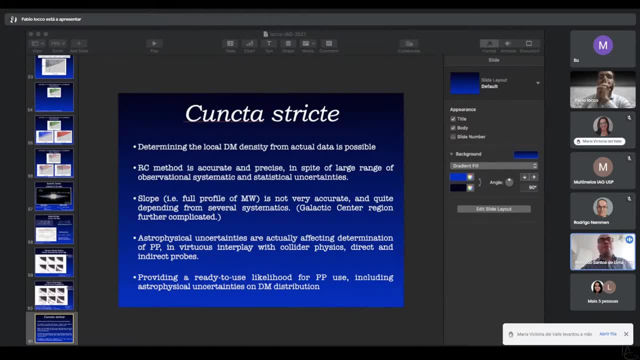 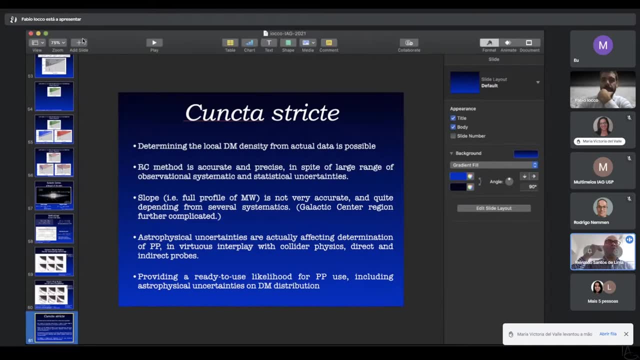 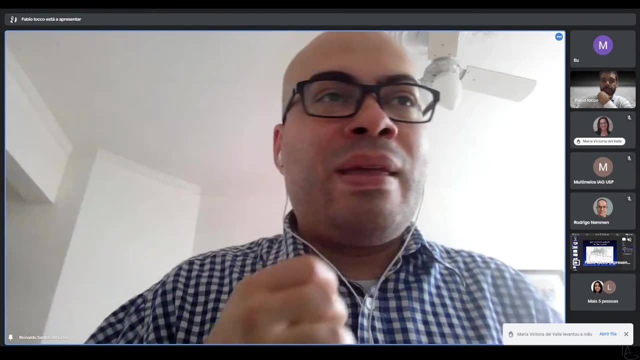 of your presentation. So you showed some study you made some years ago where you took different models for the distribution- 3D distribution- of stars, gas and, I think, the gouge, But this one, Yes, yes, I mean, we are talking about this. 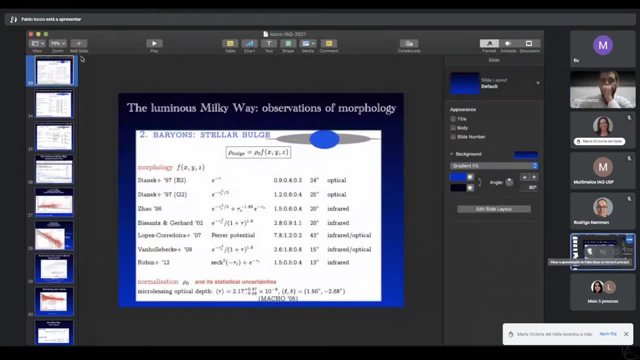 Let me hold on a second. Yes, and you combine it different. yes, So I just would like to confirm this information. Did you detect any bias as something that the newest models are requesting? less, Yes, Okay, Less dark matter or something that could lead some sensitivity. 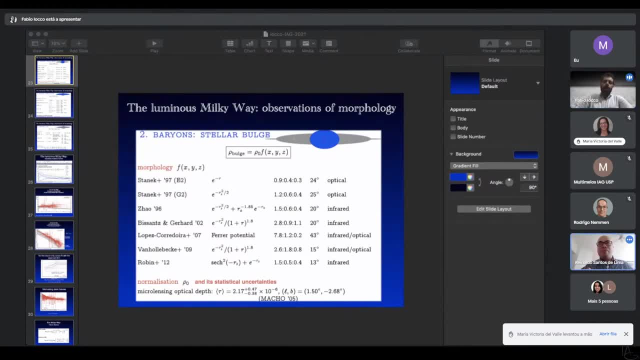 bias in the instruments. No, no, no, no, We didn't go through such a thing. So one thing that I I'm sorry for being pedantic, It's not meant as a criticism, but we always try to not use the word modeling. 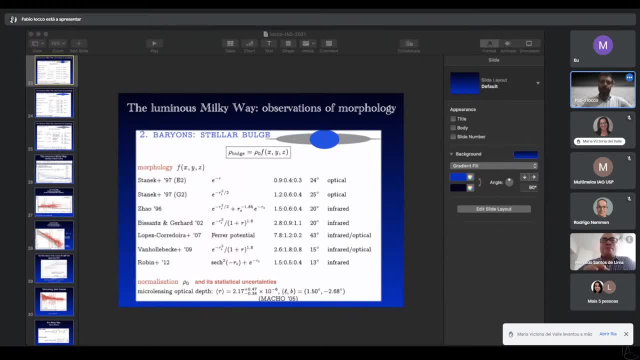 because all these are observationally inspired. okay, So we actually, before submitting all the papers, and even when we talk, we tap on each other things. We don't call them models because it seems like it's theoretical, It's not. 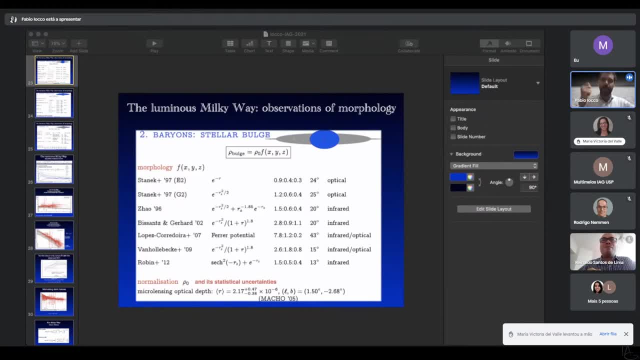 It's data-driven, So it's a more. it's an observationally inspired or driven morphology, So for each stellar component it's observationally driven. Okay, It's not a, it's not a model. Eventually there's a model, but if you call it a model, 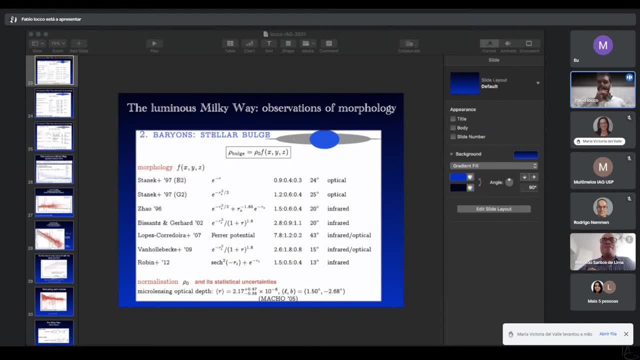 it looks like it's theoretical. It's not Okay. Didn't want to criticize you at all. I'm just saying for my sake of mine, No, no, Anderson, but the parameters of this model are a fitter from the data, right. 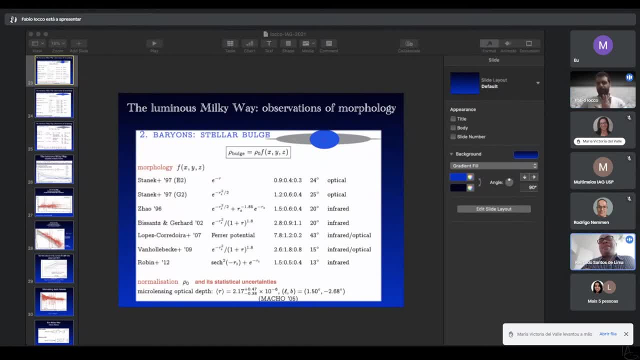 Yeah, absolutely So there. yeah, I'm not criticizing you, I'm not criticizing you. I just just want to make this clear. No, no, Anderson, your point yep, But we didn't go through such a study. 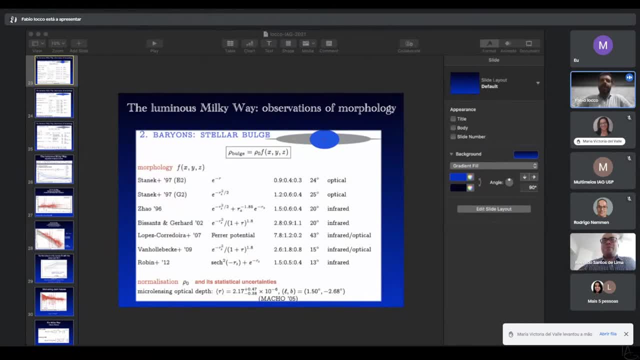 What we did is we threw out a couple of morphologies that were in blatant conflict with the data. that we did Okay, Because they they were incompatible with some later data, so clearly they were wrong, Great Okay. And what we did most recently? 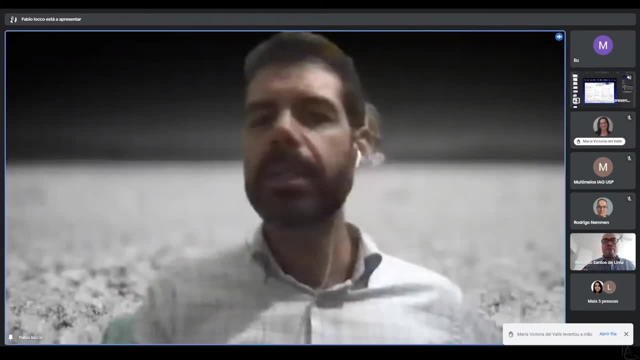 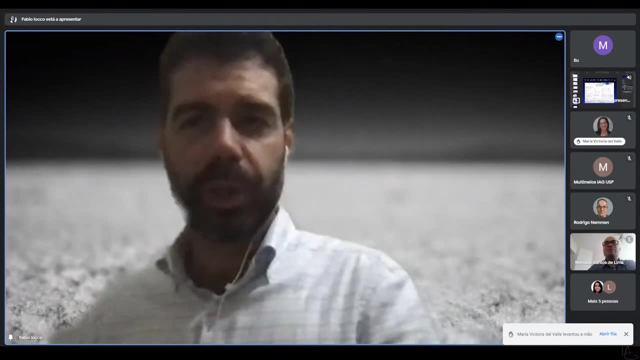 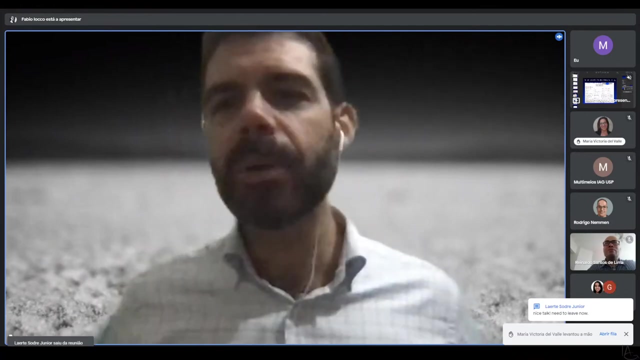 there were some determinations of the surface stellar density obtained through Gaia measurements. So whenever we have to take a reference bound, we use those, but the general conclusions don't change if you use the others. so of course we need to have a reference model because it's easier, but we present the running. 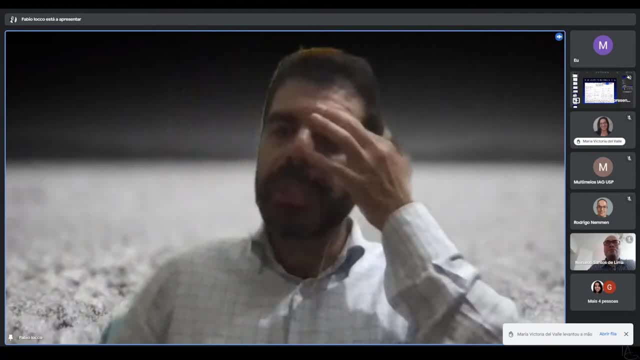 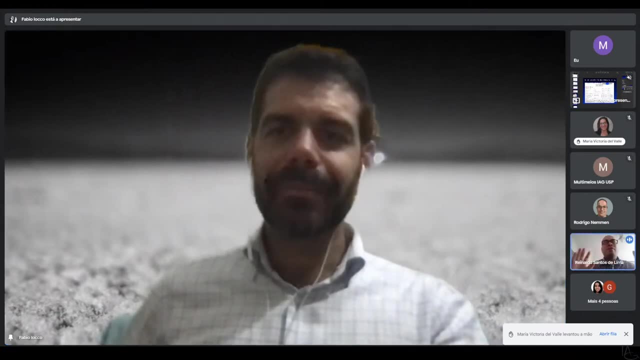 overall, especially if we want to get into this. but we didn't go through such a systematic study as you're suggesting. right, anyway, there is not. that indicates there is some sensitivity. systematic error. that's the newest uh data are requesting uh, less density of a dark matter. no, 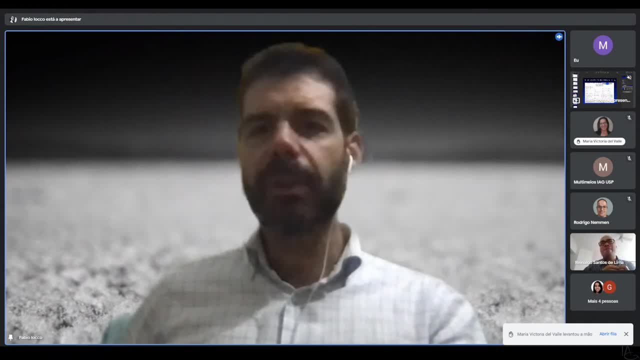 actually, if you take everything i showed you, it's not as much as the morphology of the stars is the rotation curve. also, everything i showed you is for this rotation curve that we put together, uh, some time ago, but then now there is the, the rotation curve based on the gaia. 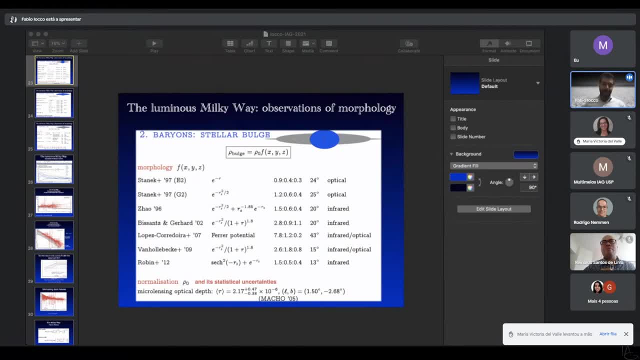 cephids. if i'm not mistaken, we tested our results with the gaia data. we're taking the rotation curve of the guy. i'm not presenting it here because it's not our work- but if anything, it wants more of that matter and they have now more. they have narrower statistical 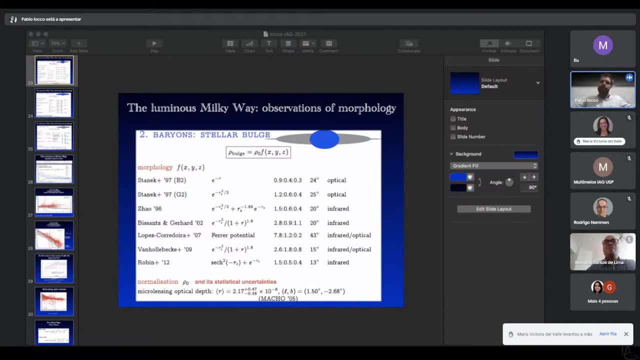 uncertainty. now the gaia data don't extend too much farther, so it's limited, but we are totally compatible. if anything, they're a little bit upshifted and we describe this in our latest paper with maria, so you can check out my name and benito and you will find results. it's compatible. 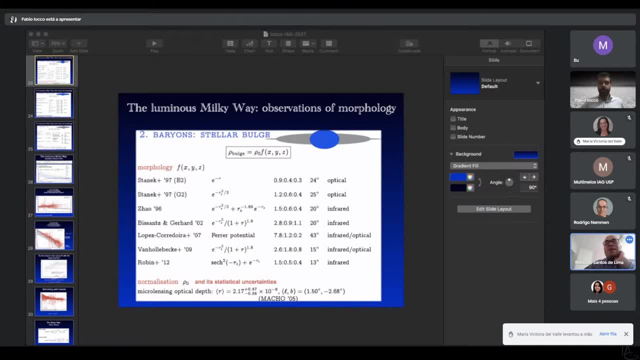 yes, this is actually. thank you, maria. there's another question. yes, i have a question also related to this, not to the details, but when you you use different prescriptions, let's say right and for, for the different parts, let's say, of the galaxy, and then you conclude that, for in all the cases, you need this dark matter component. 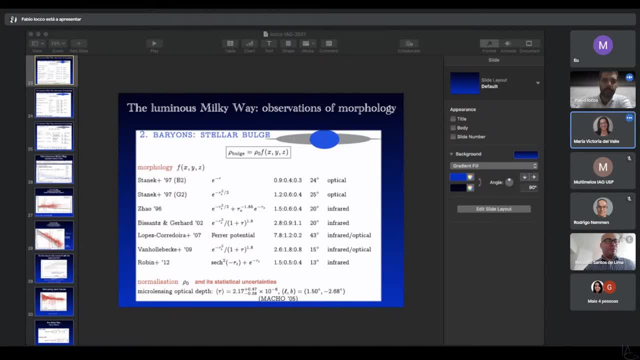 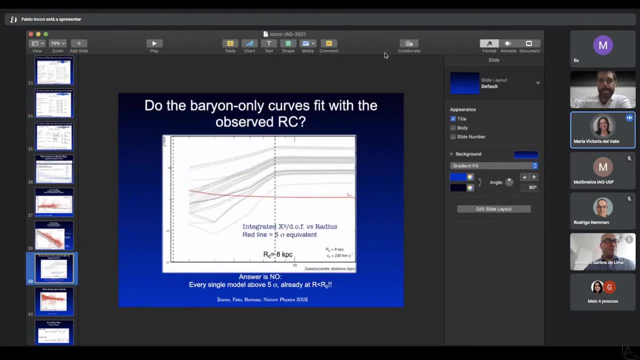 in the, in the solar cycle, let's say, right within, yeah, within, yeah, with winning. so i i am wondering how how much the, the prediction of, of how much this dark matter is in this, uh, within the solar cycle, between the different prescriptions is there, like i don't know, the integral, i don't 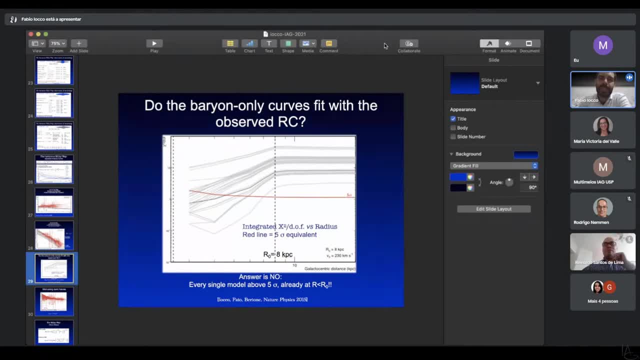 know about. uh, yeah, yeah. no, we didn't compute how much is the mass of that matter within the solar circle, the spread? uh, it's a, it's a trivial exercise. you can do it, or maybe maybe we did so. i remember we computed different masses for for all the different morphologies, but maybe up to a scale radius, not up up to the R naught, but 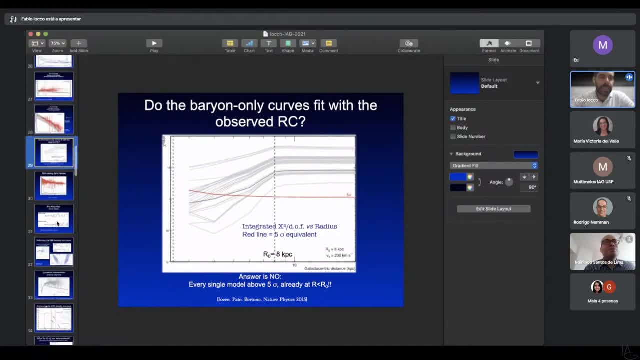 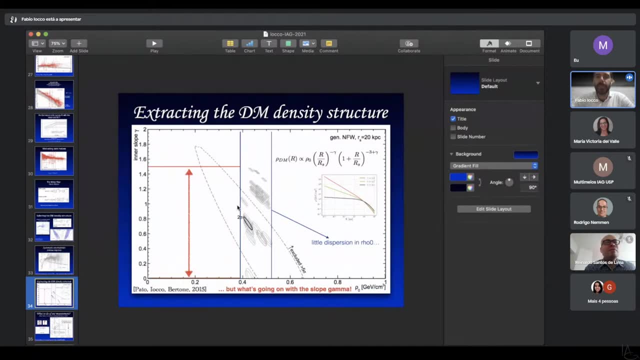 it's a very simple integral. uh, you, you take, you take this plot. yeah, you take, uh, you take R, naught and gamma and then you integrate. you have, these are two numbers. come, you take the central, it's two numbers- you put it in your slope and then you integrate it up to R, naught and then you 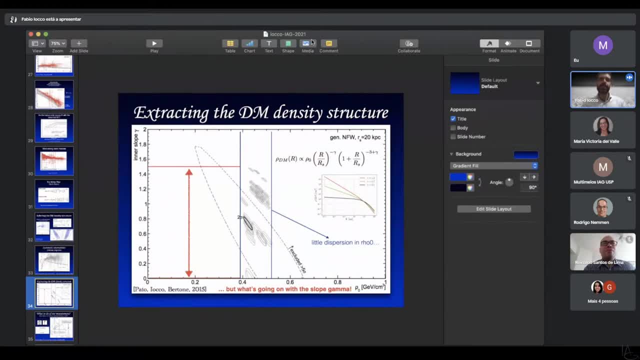 we haven't done it because- and that's that's, that's one thing. uh, the solar circle is interesting only because we are there, but it's astrophysically not particularly interesting, right? so whenever you present the results, you do it either to the scale radius or either to the disc radius, which is a 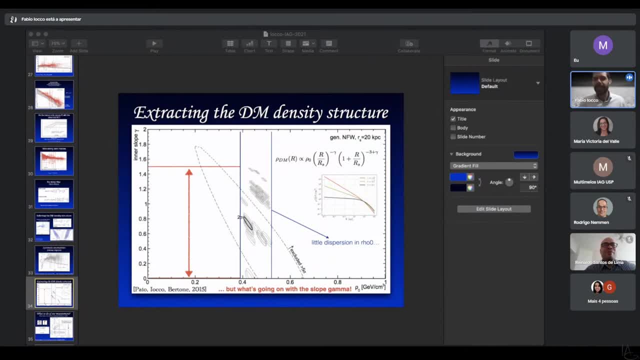 little farther than us, but once salute, she gave a seminar about the solar, the density of the dark night, of the local darkness, you know. so Lucia is quite a character, he's a nice guy and it was a physical physicist. and then he said: but but then I'm giving a seminar about this local dark matter. 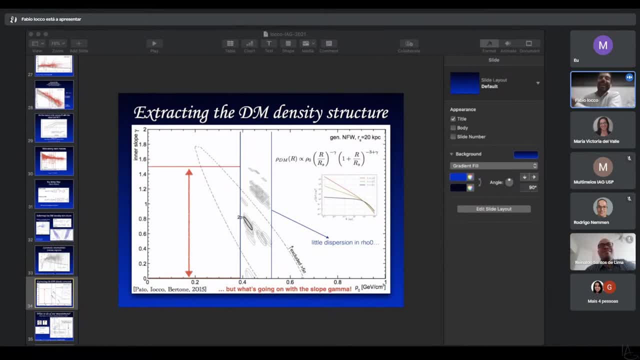 density, but I don't care at all. why should I get around the sun? well, some people are interested in that for particle physics, but from an astrophysical point of view, it's true that it has no particular interest. what it's interesting to me is the structure and how it fits in the lambda CDM. 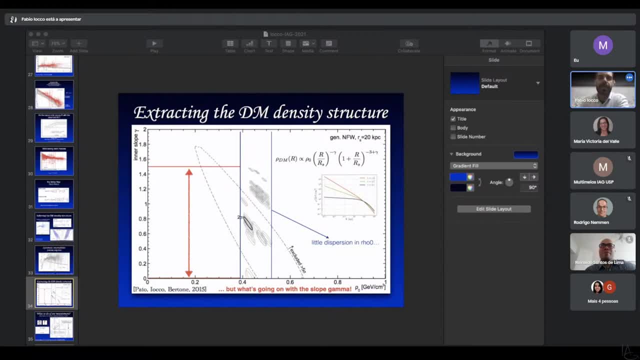 certainly the number is ancillary to the dark matter searches. certainly okay. one complementary way to answer your question is how much dark matter matters in the solar circle. so what's the relative weight of dark matter to barions? yeah, and I don't have an answer to that. 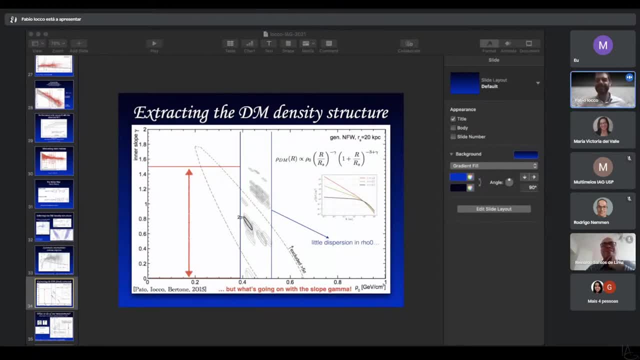 I knew it at some point. I knew it at some point, I think. I think the equality is around five or six, and then that matter starts mattering more above six kiloparsec. but I don't take this number on. okay, well, I apologize because of the noise of. I didn't hear any noise. okay, great, because I have. 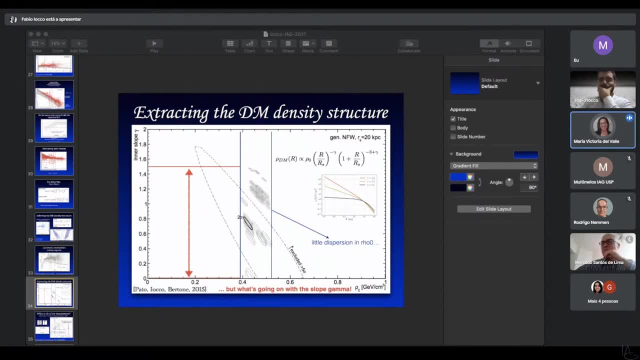 another question, but I think you you already answered that, because we are, we know we are not really in any privileged place here in the Galaxy, but is there any- I don't know- design observation plan to try to detect any sign out from this dark matter that is closer from us than I? 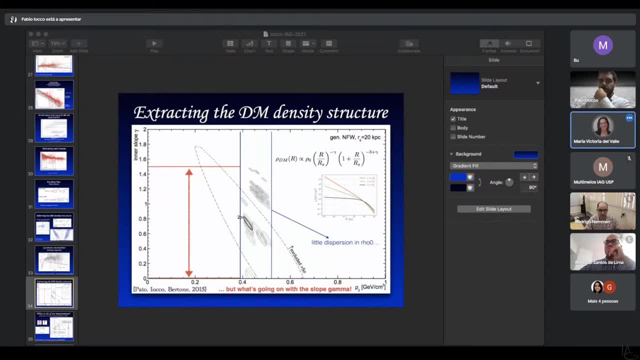 don't know the galactic center, or that would be ridiculous. I don't know so in terms, if you, if you are assuming it's a wimp and you want to look for animation, certainly you have to look at the densest regions. yeah, convolt with the volume. so it's actually it's not really true that the galactic center is the best place. 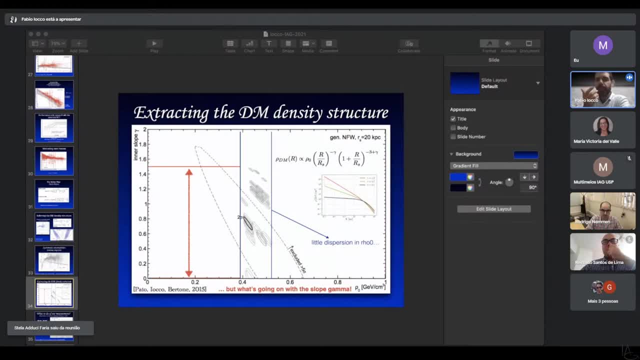 it's a little off-center, or, however, there are different possible observables, but they really. what you can observe depends on the nature of the documentary you're assuming. and then you say: I go look there and if I see something, if, well, first of all, if, if it is that thing, it can produce an. 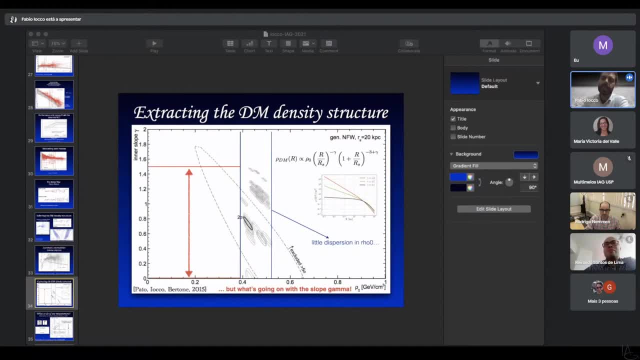 capture into the sun and annihilate into the sun And the branching ratio. the part of the dark matter that annihilates into neutrinos, it streams out. The part of dark matter that annihilates in any other kind of particle gets stuck into the sun. 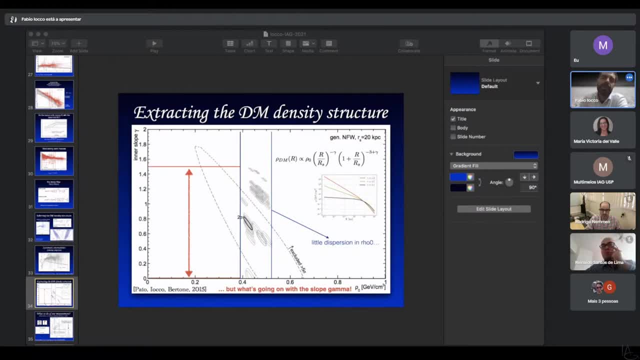 and that component is very small to the nuclear source so it's lost. But if you observe very high-energy neutrinos coming from the center of the sun, that would be a signature. There are leads onto that. IceCube looks at that and they're not very exciting. 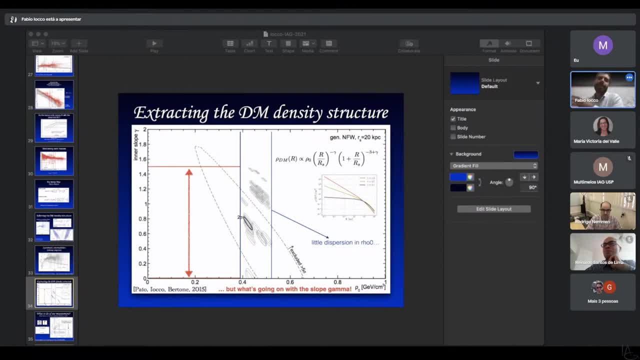 So if you take the limits that you have from other things, then you wouldn't expect a neutrino from the center of the sun, But it's closer than the galactic center. Yes, definitely, Okay, thank you very much. Thank you for your questions. 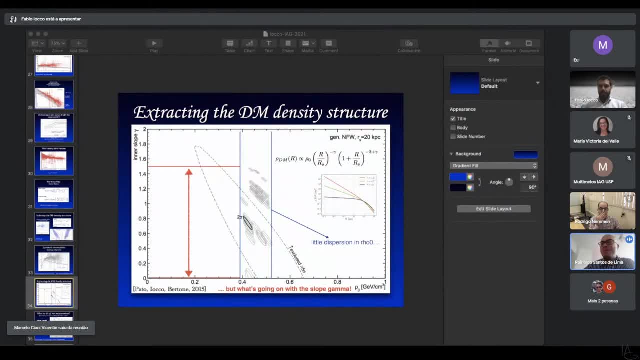 Fabio, I have one doubt. I always wanted to ask about dark matter. It's about: And you never had the courage. Yes, I never had the courage. I had a penalty. Yes, Speak, Speak. Would it form spiral arms in the galaxy? the dark matter halo? 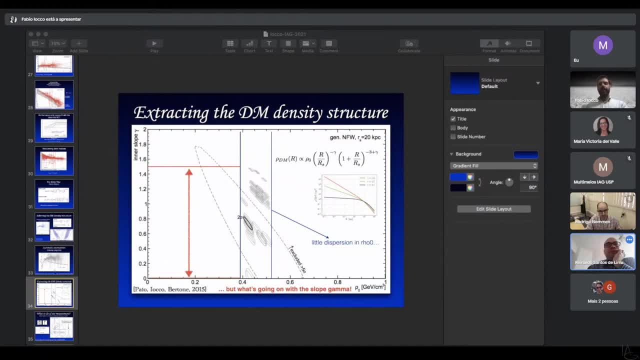 No, No, go ahead, please. Yes, because my question is if they form some kind of structure. I believe that there should be some torques between the gas and the dark matter and some exchange of angular momentum and some kind of frictional dynamic. 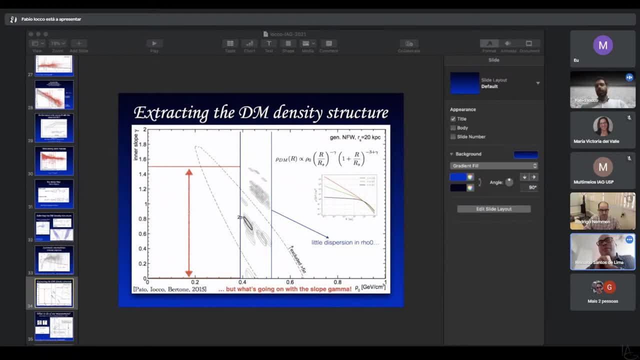 So you don't expect to form a spiral arm. The spiral arms- also from what I The latest I remember, and you certainly can ask galaxy information people- but the spiral arms in the stellar structures they're not an emerging structure out of gravity necessarily torque moments. 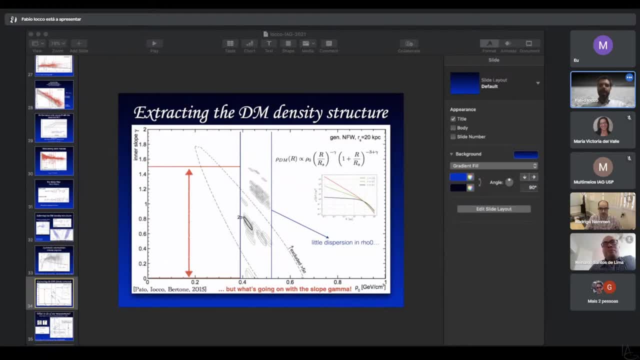 but from what I understand, the spiral arms- now there is more credit. there is some basically satellite passing, So the fact that there might be some satellites, it disrupts and then it looks like a spiral thing, but it's not really a spiral due to the torque. 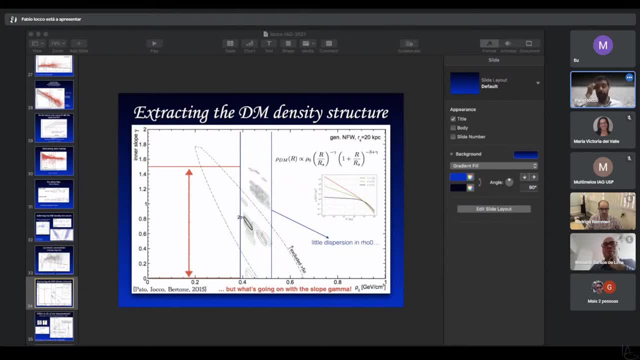 I might be mistaken on that, but that was my latest impression, That for the stellar component. Now for the dark matter. you don't expect to cause anything like that right, Because it's dissipationless, And so you expect it to be distributed as a spherical halo. 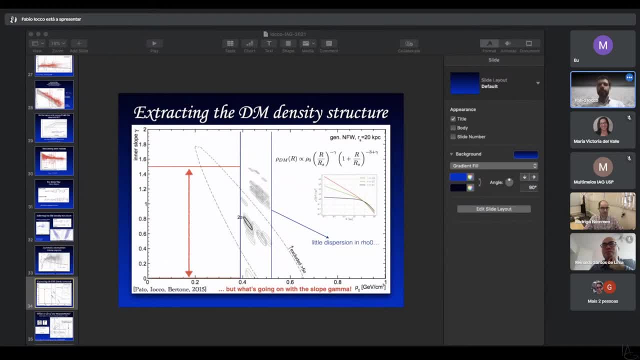 Though there is a lot of interesting work about the fact that you see. You see stellar streams, and you know that stellar streams are usually proceed from a disrupted dwarf galaxy. okay Now, so there are stars that were previously in a dwarf galaxy that was disrupted by a tidal encounter. 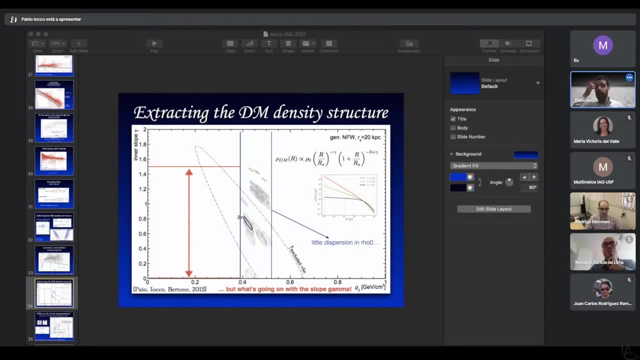 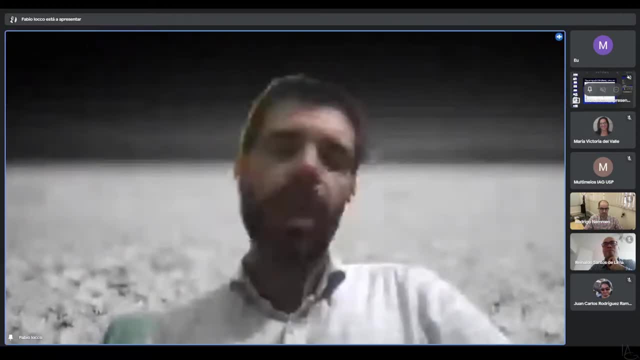 So it merges with the Milky Way and it's stripped, okay. Now there is the group led by Mariangela Lisanti, who is an amazing scientist that has done a lot of. There is also another group that, I apologize, I don't remember. 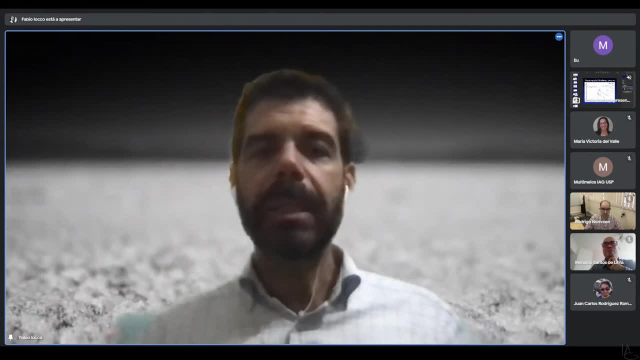 but they do very similar work and I remember the one from Mariangela. They are tracing in simulations streams and they know that if there is a stellar stream, there is a stellar, there is a dark matter stream associated. So they know that if we see stellar streams in the Milky Way, there must be a dark matter. 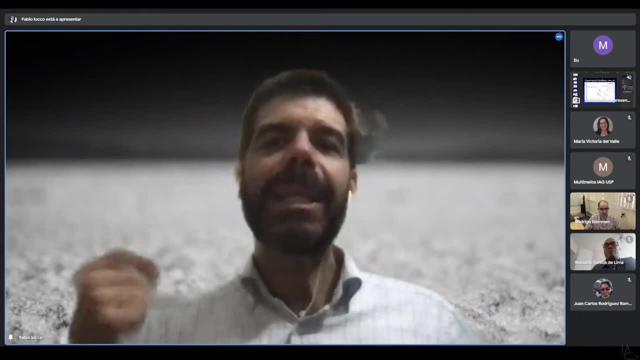 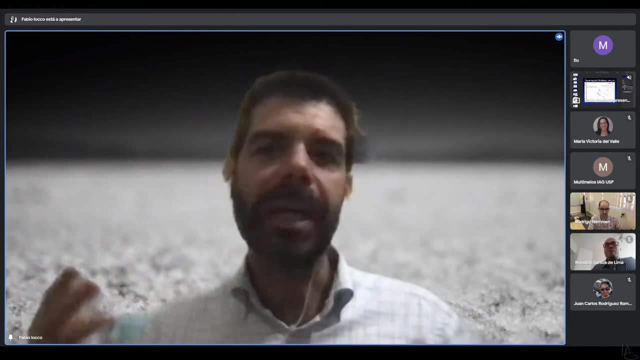 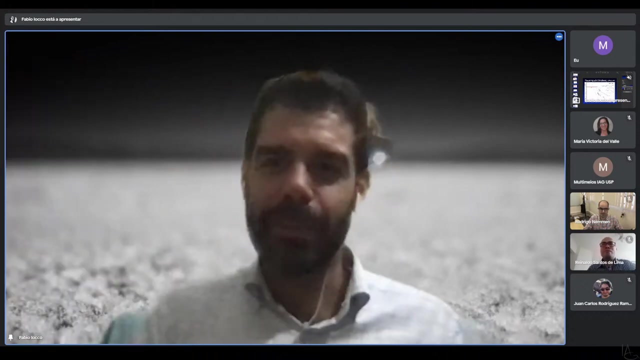 component stream associated. So even in simulations, the weight, the mass of that stream is not altering the total mass, so even one-third or something. but the phase space would be entirely different because that's moving, it's a stream that is moving. 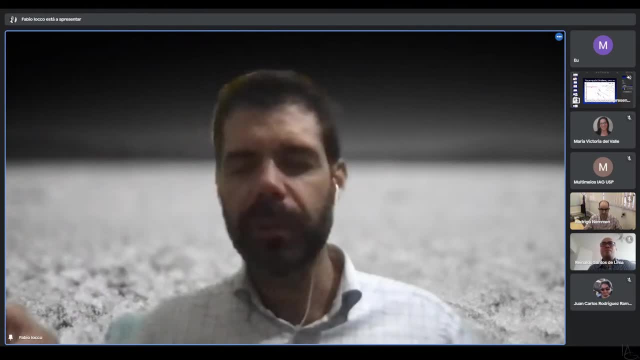 So if you're interested in this- and I know this brings all sort of conclusions in terms of particle physics- if you're looking at the particles in the detectors at the Earth and then the phase space of the dark matter is different, you expect a different scatter. 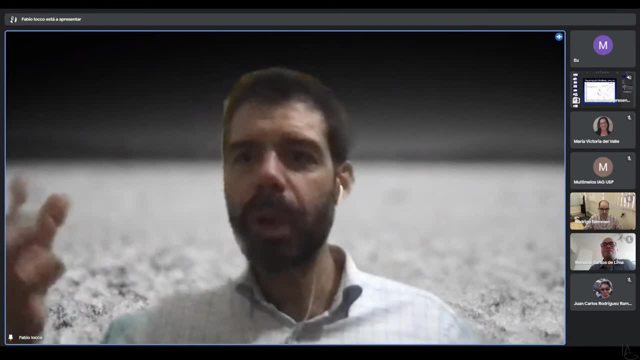 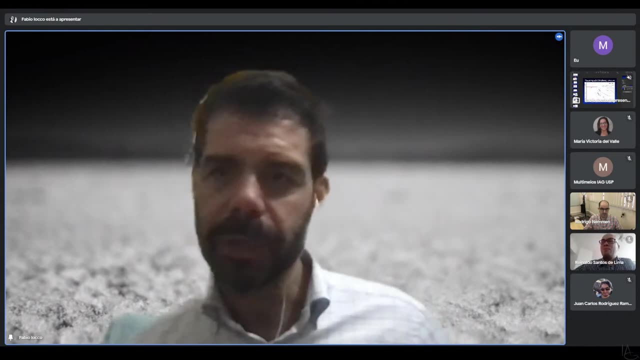 so that alters things. But if you're interested in knowing really what happens- and it's possible- I would recommend to see the last titles from Mariangela Lisanti's group. It's not only her. there's a lot of very good people, but I remember her name. 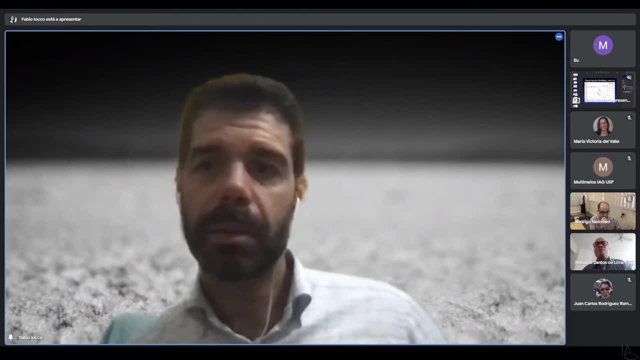 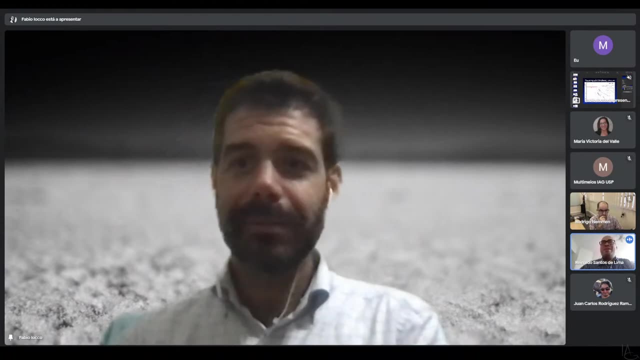 And you can check that. I think it's amazing work. Thank you, I will take a look at this work. Thank you a lot, Fabio And Rinaldo. I would like to thank you again for being here, for sharing your time, your research. 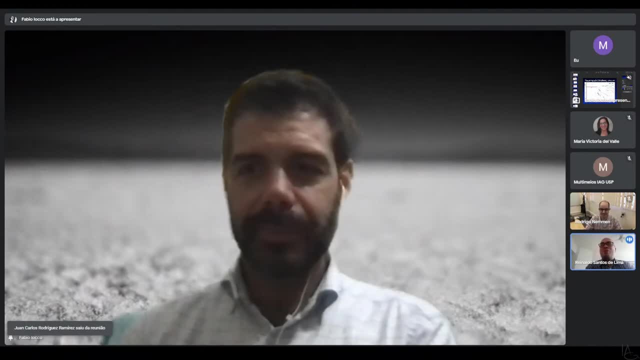 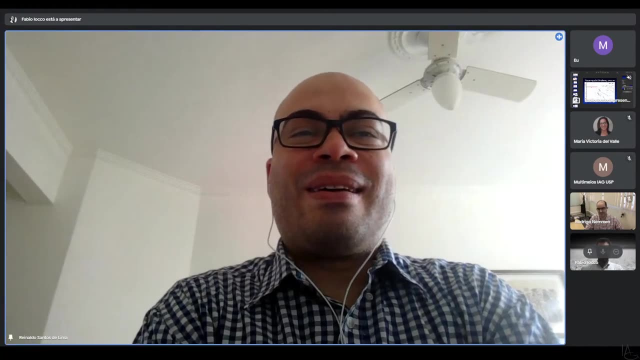 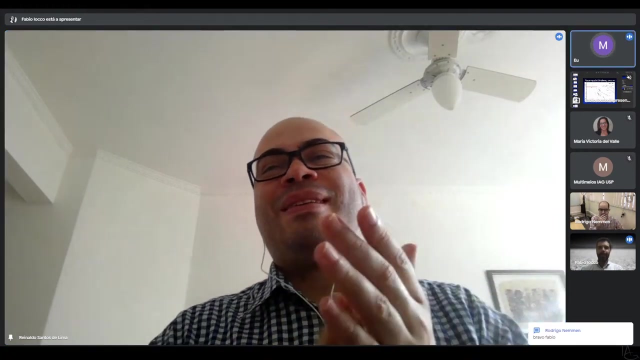 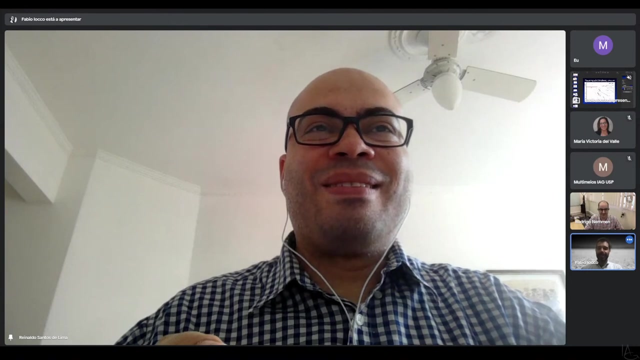 and your knowledge with us, And I would like also to thank everyone following the seminar and YouTube here in Google Meet. And now I think we can close the. we can stop the broadcast. Thank you, Rodrigo. Thank you very much. Thank you very much for your patience. 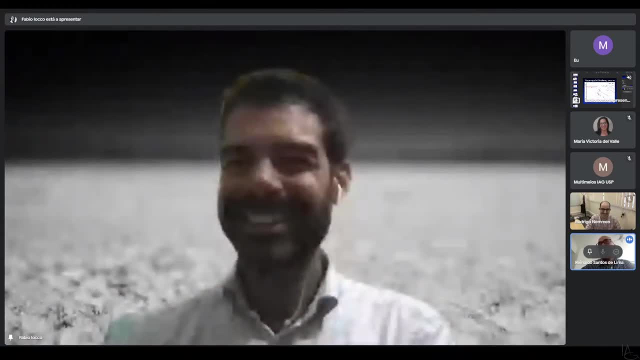 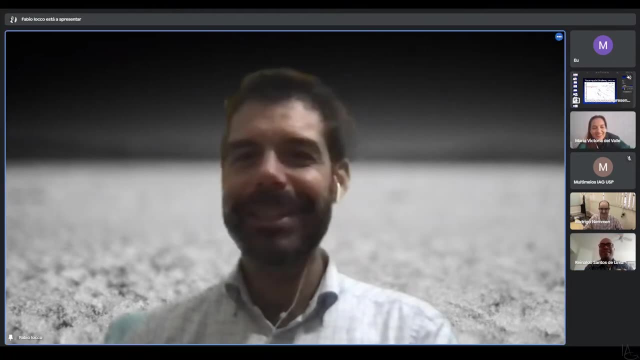 I think it was a little more than time. No, no, We always spend a little bit. Thank you very much, Fabio. You are welcome. I'm going to get a drink because unfortunately I don't have a cachaça. 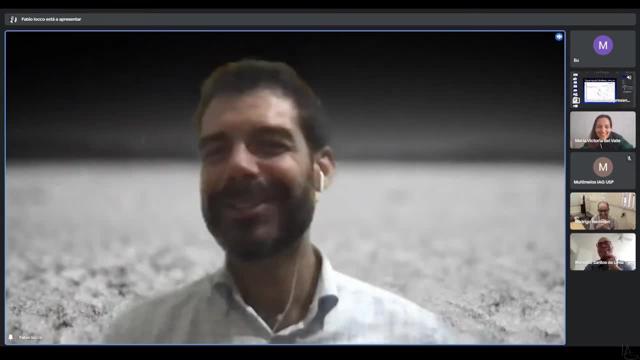 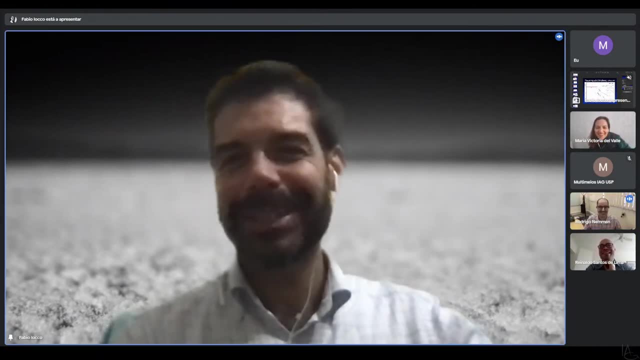 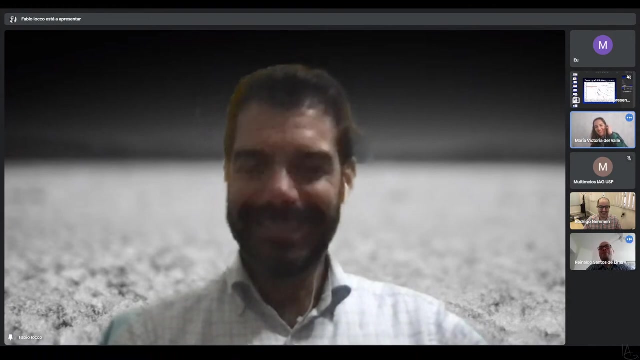 but I don't even have a good one. Let's make a Bye, Fabio. Thank you, I can go to São Paulo, That's it. Then you go to IAG. Do you have students here, Fabio, That you are guiding? 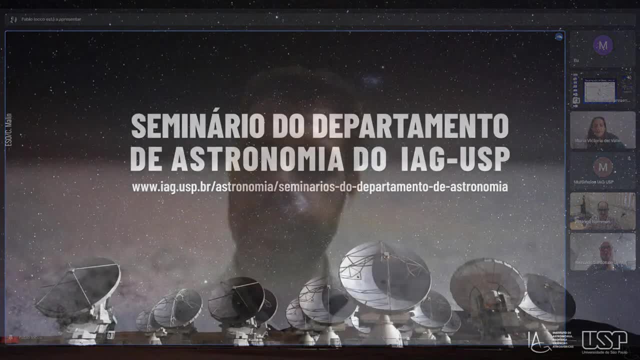 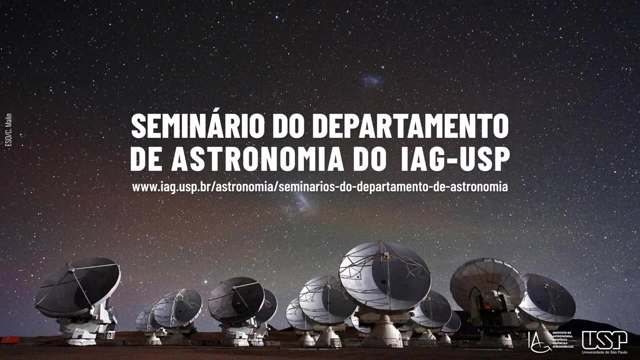 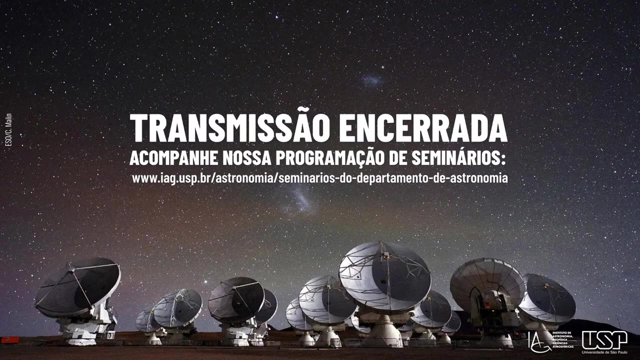